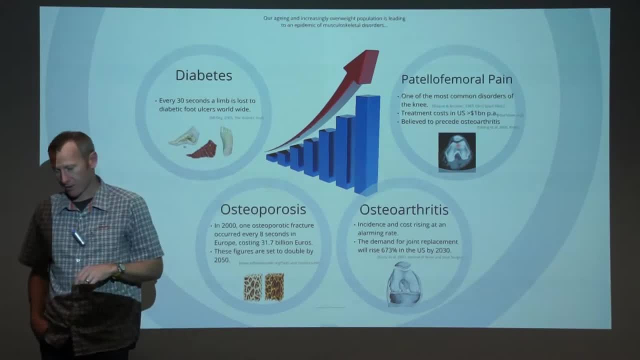 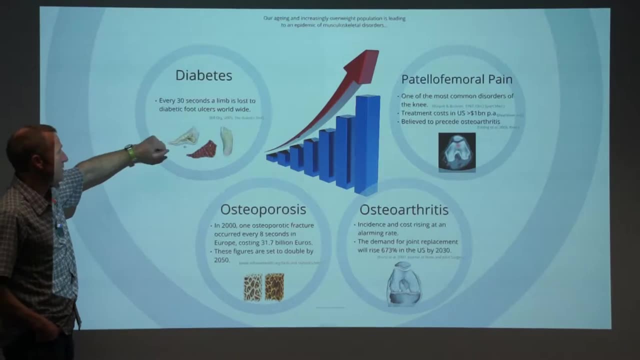 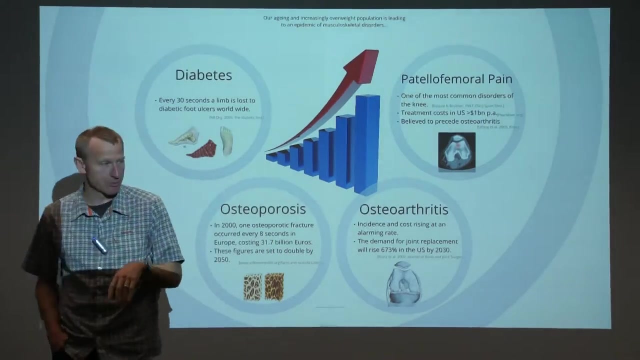 osteoarthritis to real big ticket items, things like stroke, which is the leading cause of disability in the world, as well as issues such as diabetes, And I've put one up here just as kind of a sport, more sports medicine oriented one, which is patellofemoral pain, And even though you may 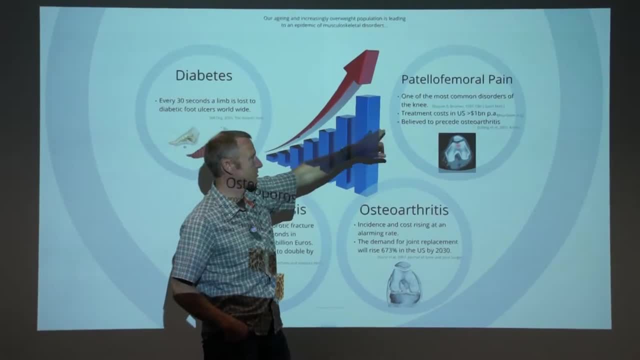 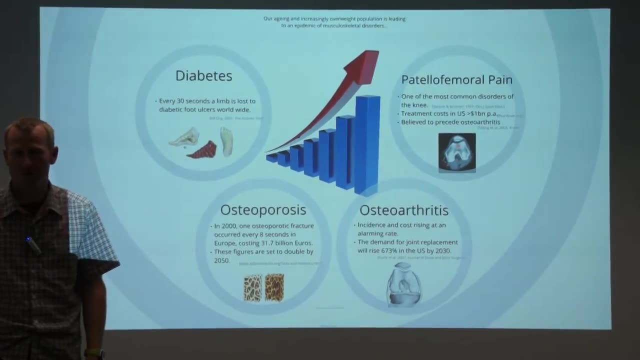 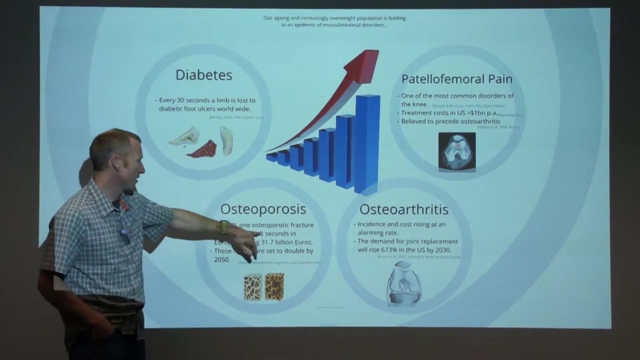 not think of this as a major problem. if you look at the costs- and these come from the United States, you know there's over a billion dollars spent per annum and rehabilitation costs for for this disorder. So and all of these combined have some pretty alarming statistics. So here you know. 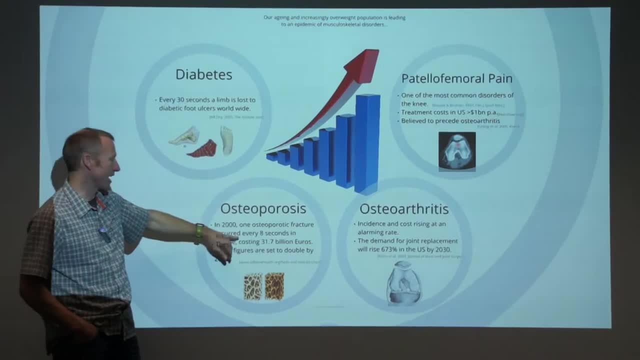 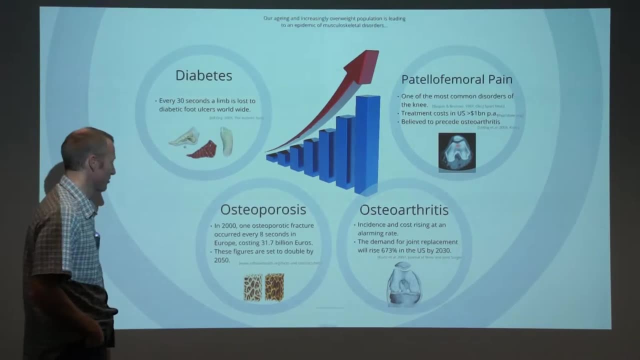 this is a bit dated now, But in Europe alone, every eight seconds there's an osteoporotic fracture. So while I've been sitting here rambling on to you, there's been already a dozen fractures in Europe, So that and these figures are set to double by 2050.. You know these are alarming statistics. 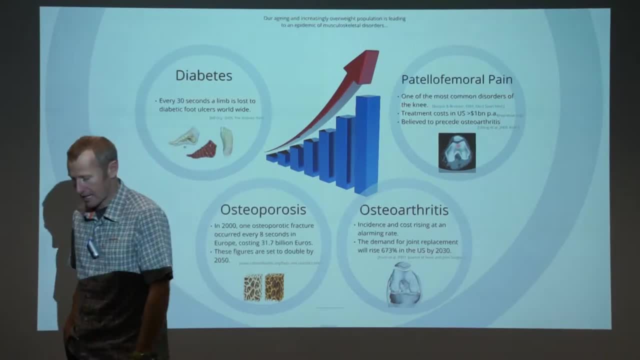 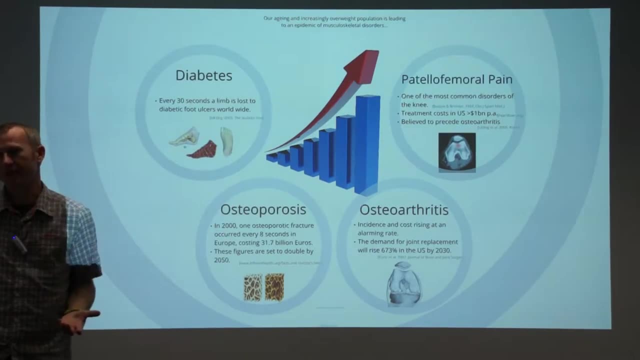 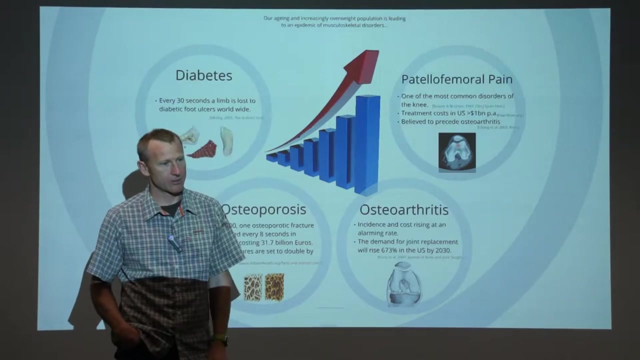 This is an interesting one. So joint replacements in the United States in the next 15 years are going to increase almost seven fold And we can't sustain this. we can't keep it up In terms of our current medical model. we just can't afford to have a seven fold increase in joint replacements. 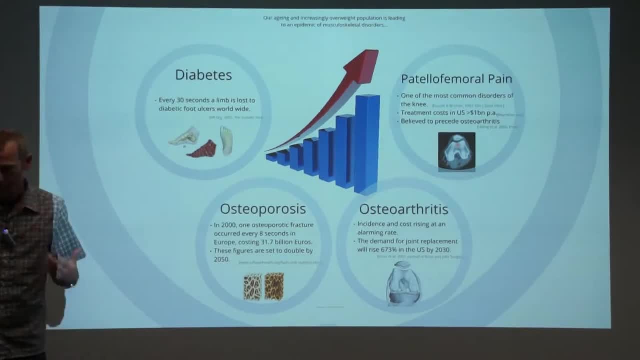 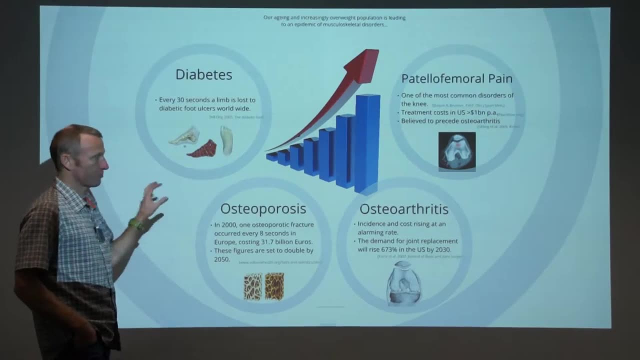 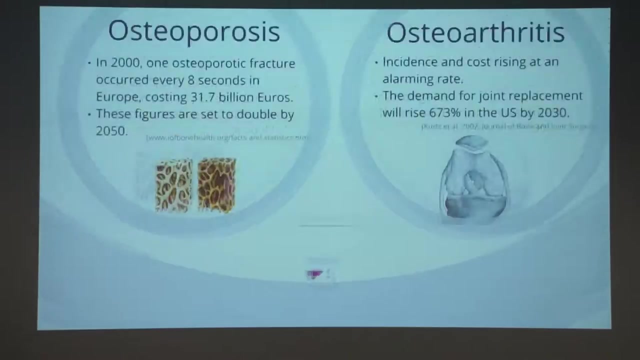 It's just not not possible. And so you know we need, we need solutions to these problems, And the solutions then have to be more on the preventative side as much as possible, as opposed to trying to fix these after the fact. So just a quick. 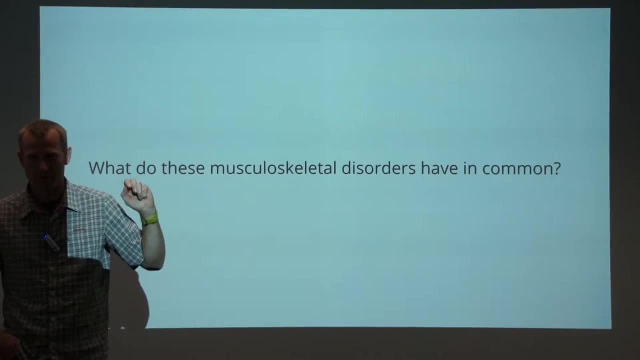 question out there. What are these disorders have in common? Anyone want to throw something out there. What could you see that maybe is common across those disorders from a very high level? Bones- Yep, Involved in the bones- Yep for sure. And what we think about the kind of the etiology or 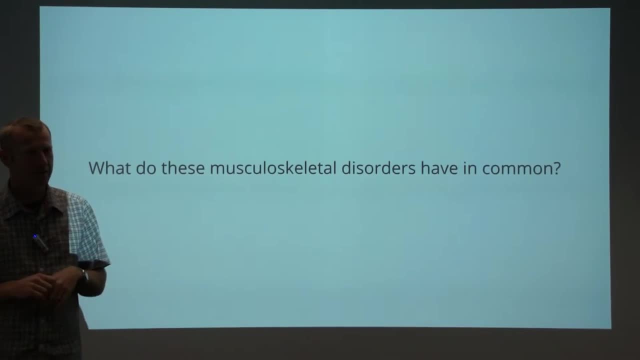 the progression of the disease or how people might get these diseases and other things. What's really common there? Is it due to genetics? Is there a predisposition to get it from diet? Is there a predisposition for the loads that we experience? 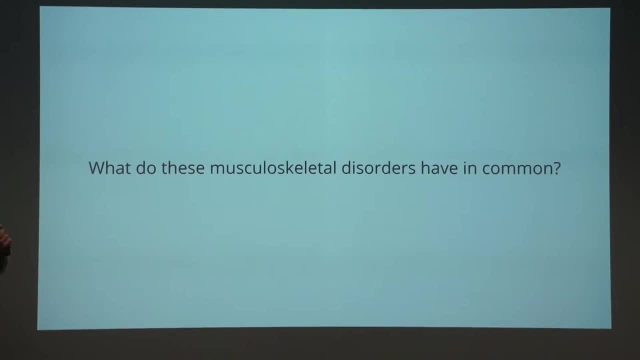 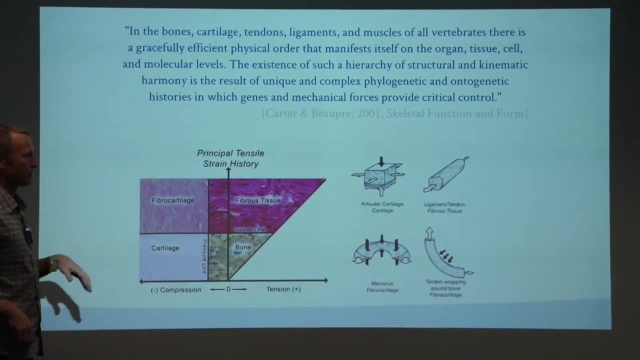 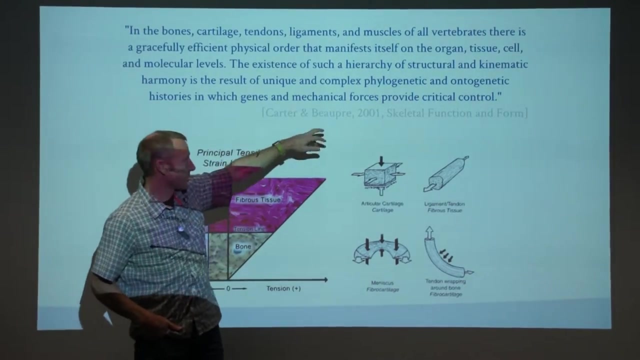 There's actually, of all of those disorders, loading is a key feature that is linked to the onset, the progression and the severity of these disorders, And so I did some work at Stanford for an interesting number of years, and I worked with these two gentlemen, Dennis Carter and Gary Bowpray. 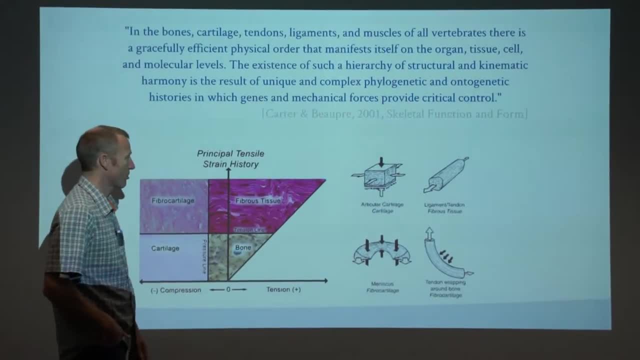 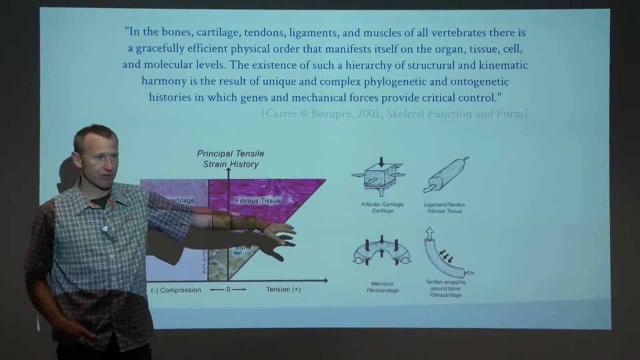 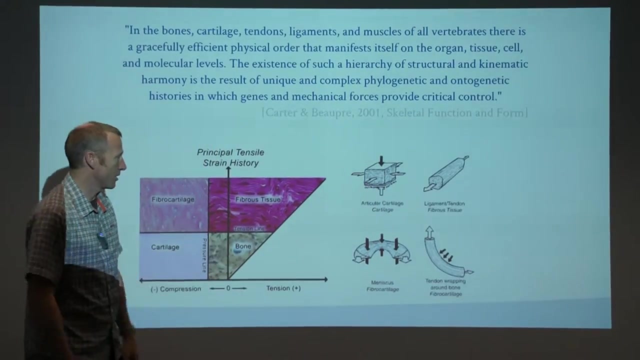 And for decades they've been doing some really interesting research to try and understand the relationship between the mechanical load history of a tissue and its phenotype. You know, how was it that articulocartilage becomes this particular phenotype, this tissue? How was it that ligament and tendon becomes this type of tissue? 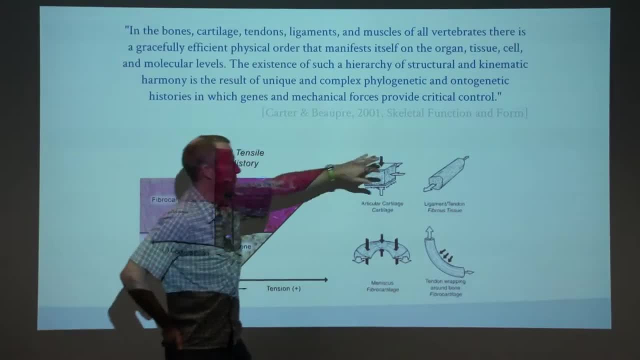 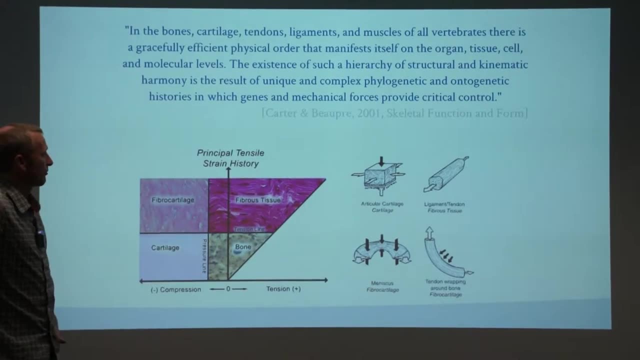 And they have this really nice statement from. this is a textbook that they've written in about what functional problems are. they've written skeletal function and form. I consider it the Bible if you're interested in musculoskeletal form and function. and what's really key here is: 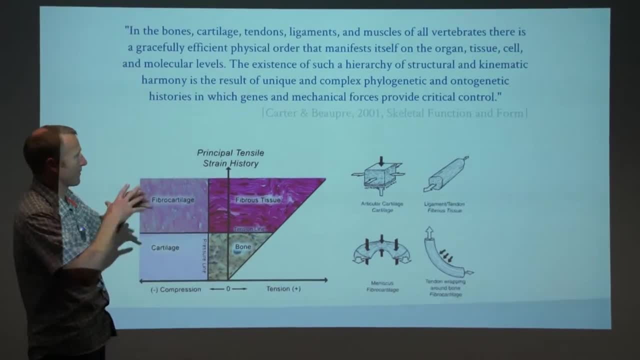 the statement that says the existence of such a hierarchy- and they're talking about the, the hierarchy that exists in the physical order of organ, tissue, cell and molecular levels, and I think that's common across what we are interested as well- that modeling per se can can cross multiple scales, both temporal as well. 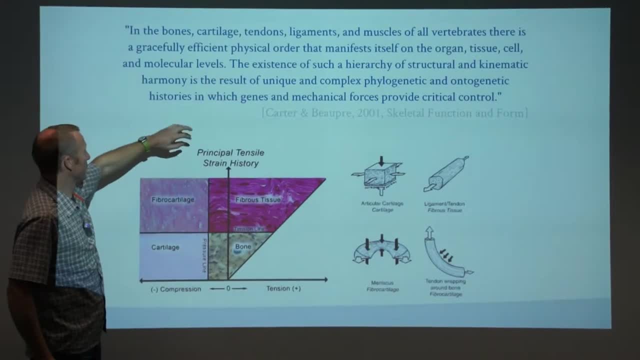 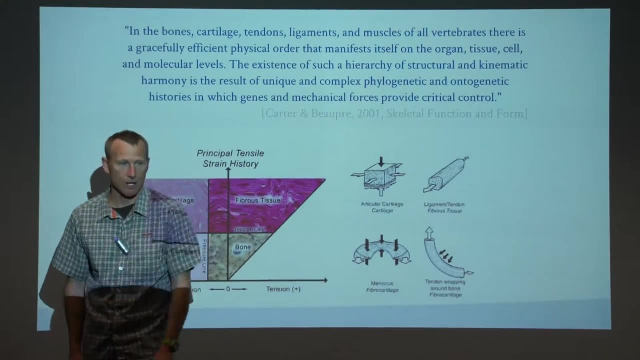 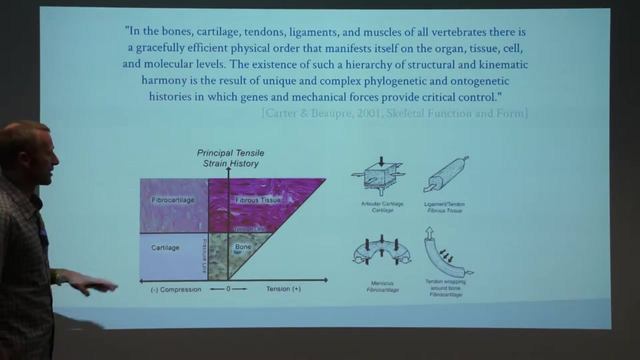 as spatial. so here it's. you know more of a spatial scale, but this is a result of a unique and complex phylogenetic and ontogenetic history in which genes and mechanical forces provide critical control and these two things that are critically linked, the genes and the mechanical loads. but what's really nice? 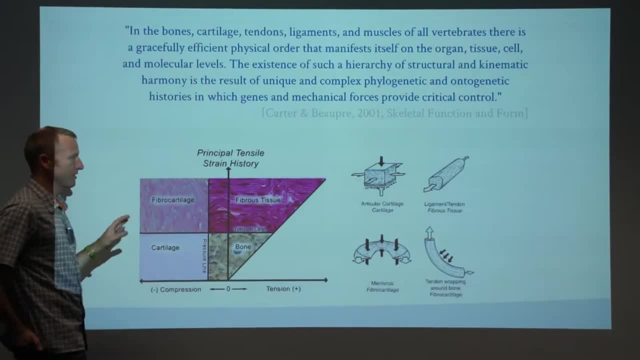 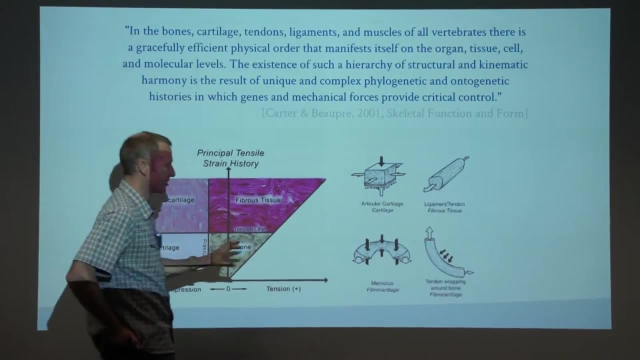 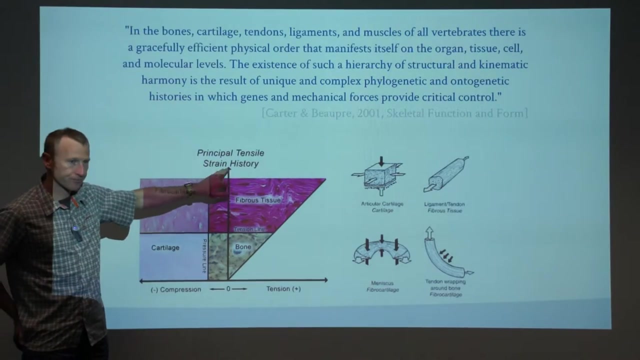 about their approach is that they can have relatively simple model of the tissue without going to the cellular or the molecular levels. they can have fairly simple models of the tissue to characterize the, the localized strain and the strain history of the tissue. and what this is showing is. 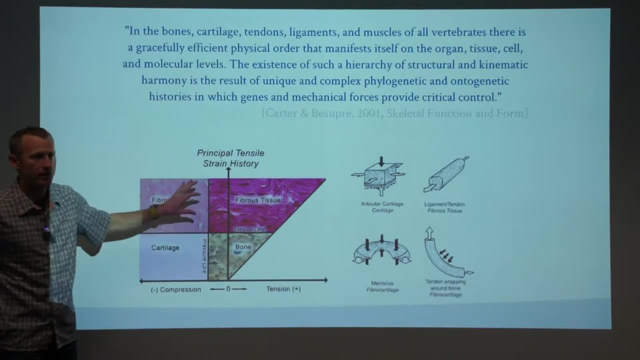 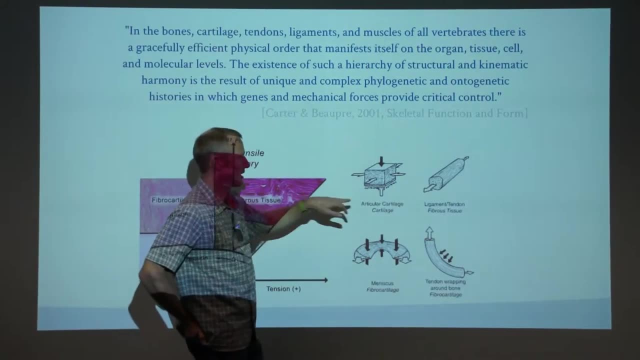 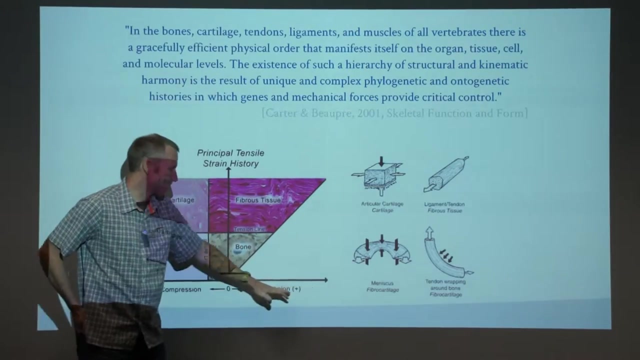 depending on where you sit in, this kind of area dictates what kind of tissue you have. so, for example, a fibrous connective tissue like ligament or tendon is typically under tensile load, so it sits in this top quadrant here. whether there's tension and its 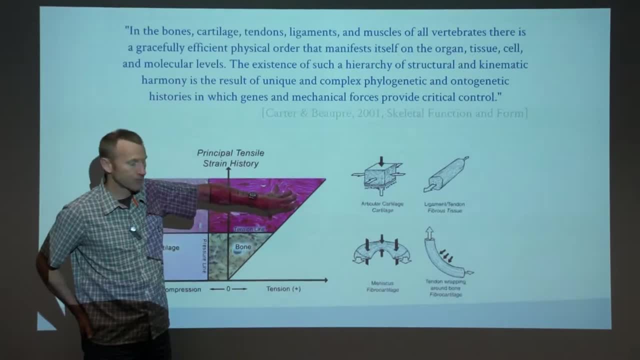 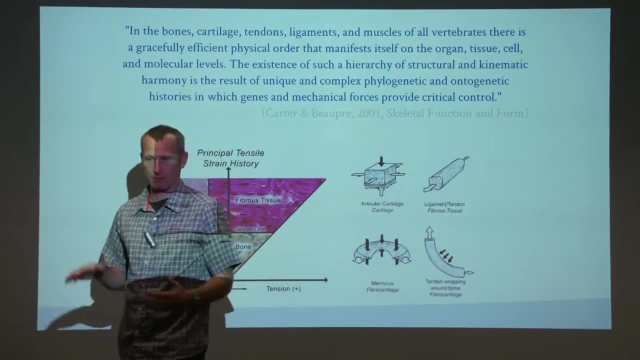 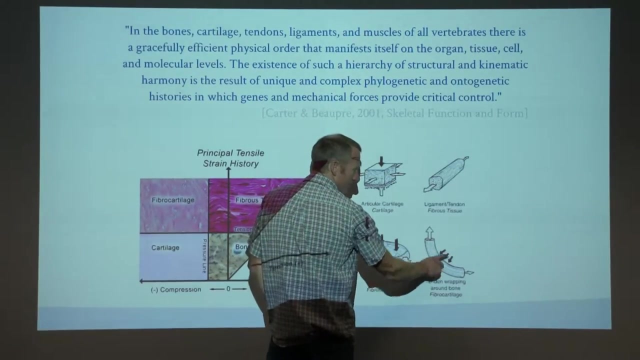 principal strain history is also tensile forces. but if you get an area of tendon that wraps around the bone, you can get a point here that's actually under compression, as the tendon wraps around bone, you could imagine then there's compressive forces here and what happens is that that bit of tendon there becomes. 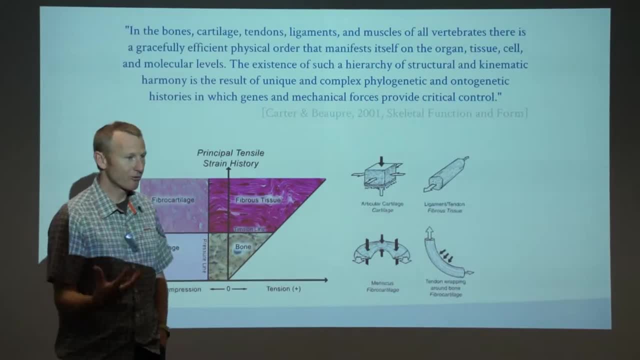 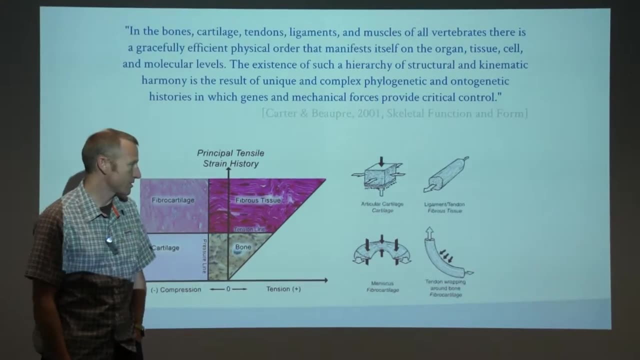 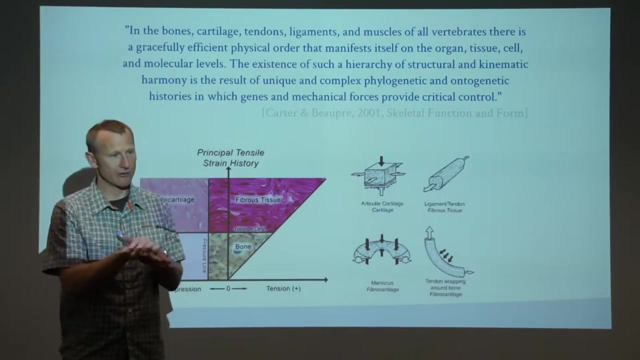 more like bone and so the mechanical forces. then there's a tight coupling and regulation of the tissues based on the load history that the tissue experiences. and there's lots of other good examples. Articular cartilage likes to see uniform pressure because it has very low friction at surface and 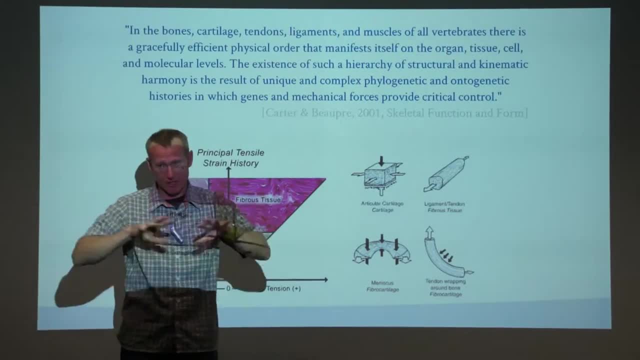 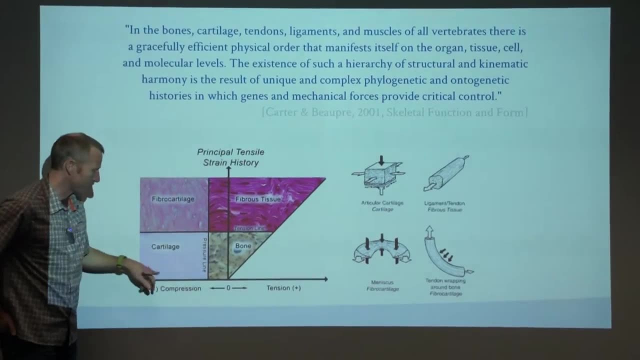 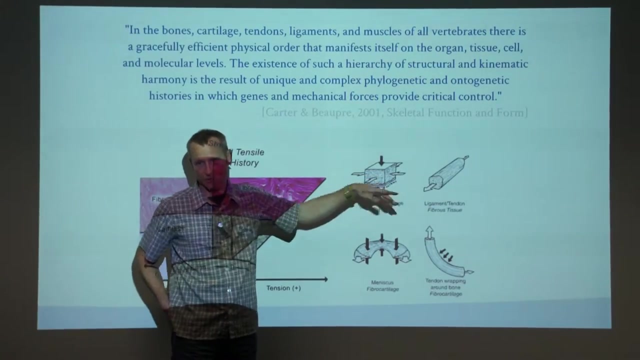 it's mostly water, 70% water. so those forces are taken up through uniform hydrostatic pressure and so it has. it sits down here in this quadrant with mostly compression, and the strain history is also compression. but if you damage the cartilage, if you damage the surface of the cartilage, you no longer 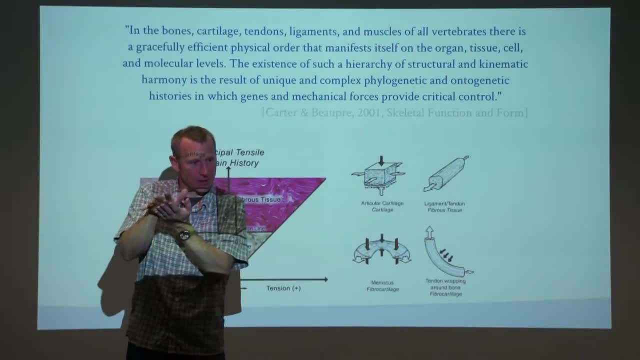 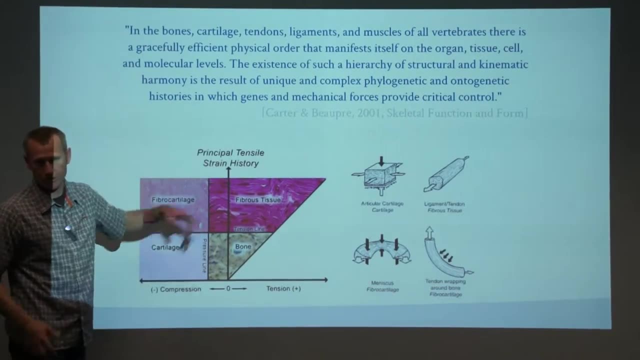 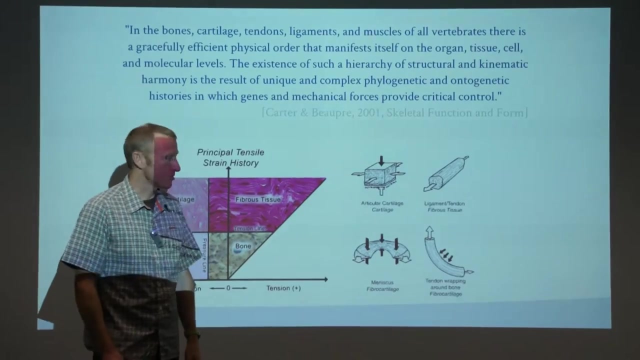 have zero friction at the surface, you can have shear forces, you have frictional forces that distort the tissue and suddenly you start creeping up into this area, you start getting more strain in the tissue and that distortion, stress, causes cartilage to turn to fibrocartilage. so anyway, 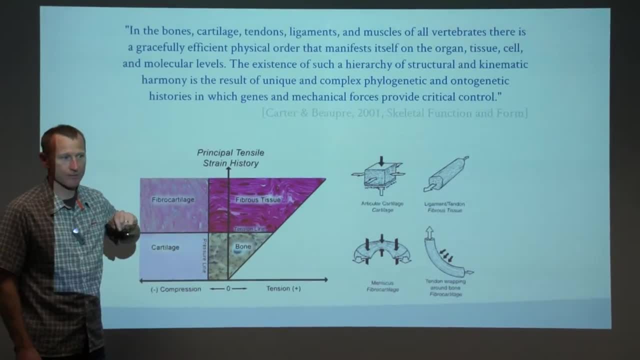 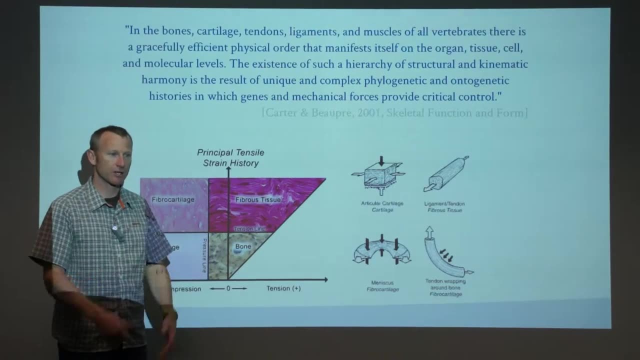 it's kind of nice paradigm, because if you're a tissue engineer, so there's people in this room who are interested in tissue engineering. if you want to understand this paradigm, you could then take cells in a culture and you could put them under the necessary mechanical loads and you can actually push them. 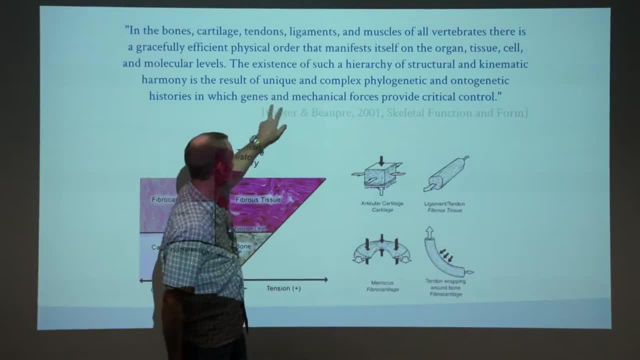 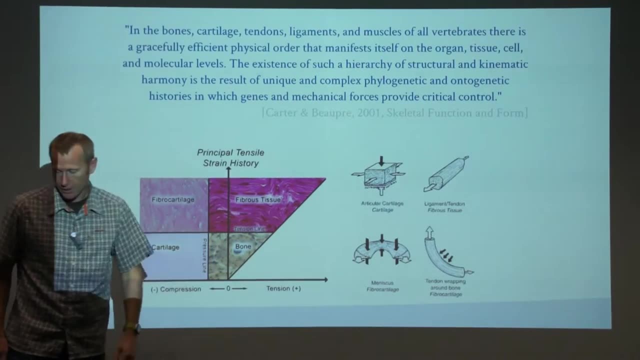 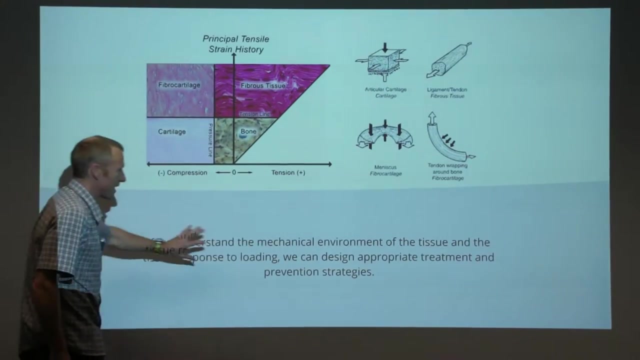 into different phenotypes if you give them. there's also this kind of link. there's also some biological goodies you can throw in there that that help the process. but it's really interesting to understand that you know that the tissue adapts and responds to its mechanical environment. so if we understand that, 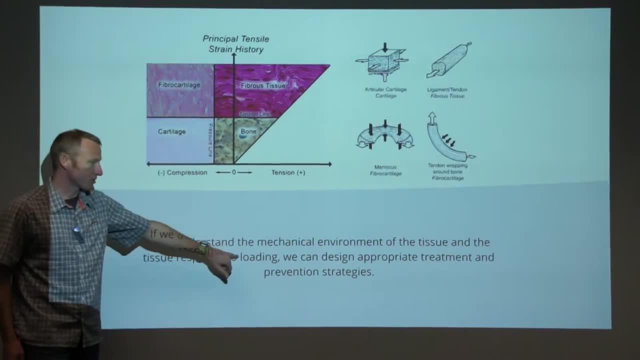 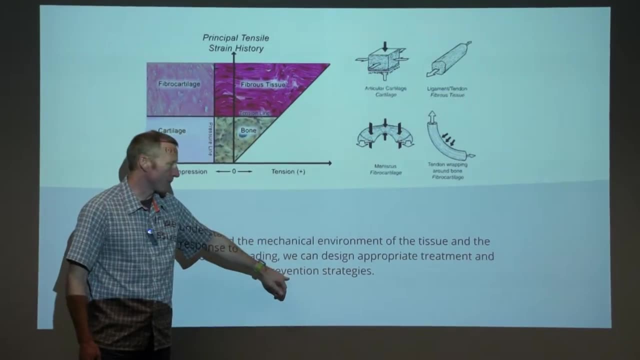 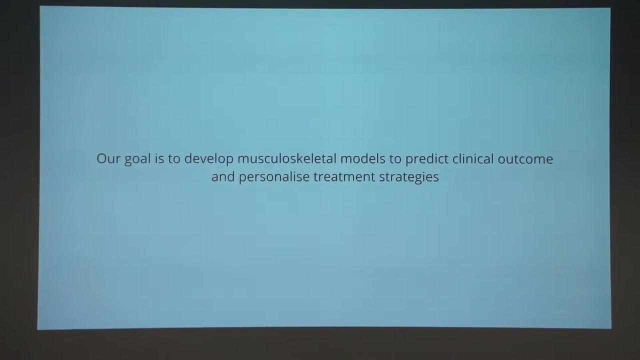 mechanical environment and the tissues respond to loads. we have a chance of designing appropriate treatment strategies, and that can also be used for prevention. I mean, prevention is ultimately the goal here. so this is our goal is to develop musculoskeletal models to predict clinical outcome and personalized treatment strategies. that's. 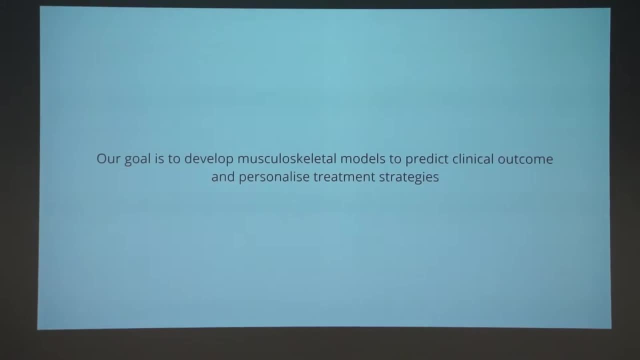 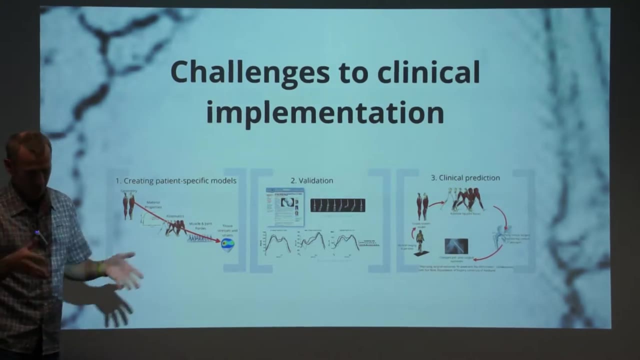 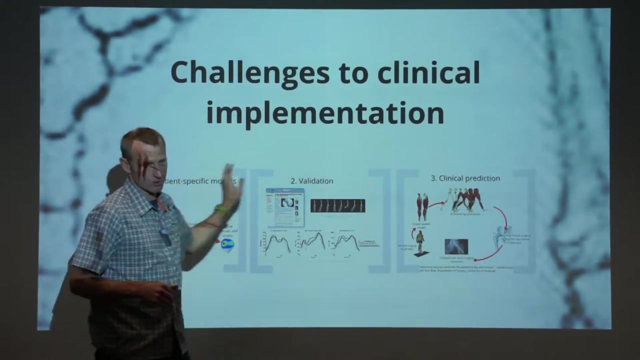 our bigger aim here and what we're trying to do. so, before we can translate this information from our computational model and go into the clinic, there are three main challenges we need to address, and I think these are across the board. what you'll see, whether you're modeling heart, lung, skin tissue. what you know, whatever. 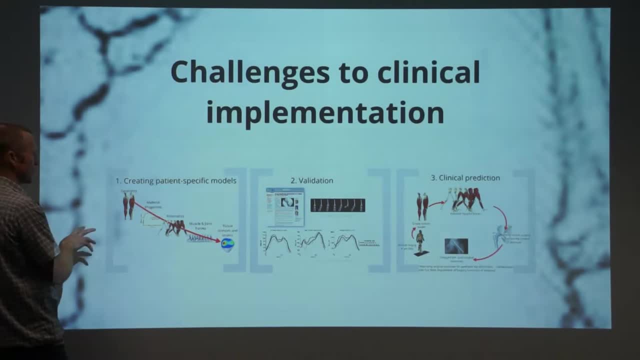 it is that you're you're doing here? the first of those is creating models that are specific to a patient, and more and more we're hearing these buzzwords: personalization, you know, patient specific models or subject specific models. and what does that mean and how patient-specific are we or how? 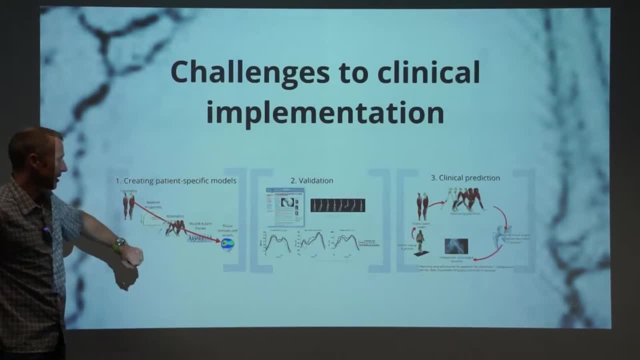 patient-specific do we need to be in order to characterize an issue or a problem disorder and then address it? there's some questions about about how we do that, but ultimately that this is a problem we need to address. the second main issue is validation. we need to have some way of always testing our models. 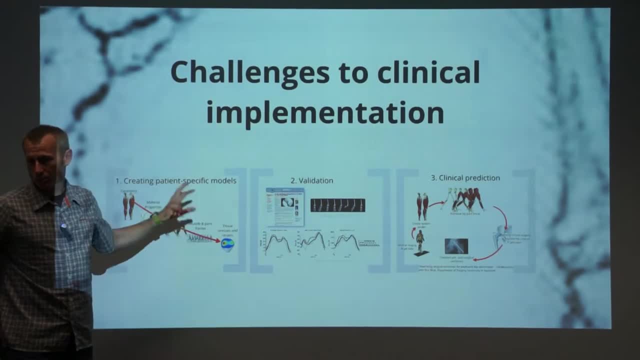 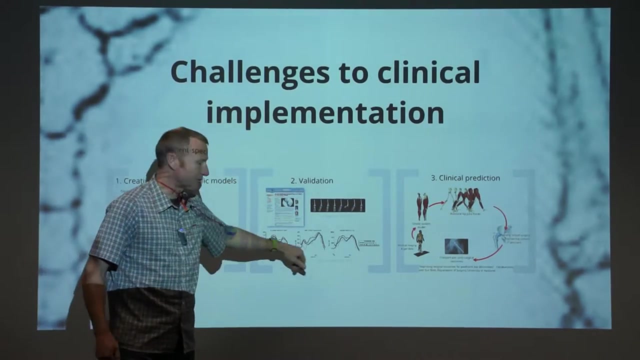 under the condition that the that they designed for models are always designed with some idea in mind of, for this is what I want my model to show me, or predict, and the predictive capability then needs to be tested, and this is what I mean by validation. if I say my model is to predict contact forces at the knee. 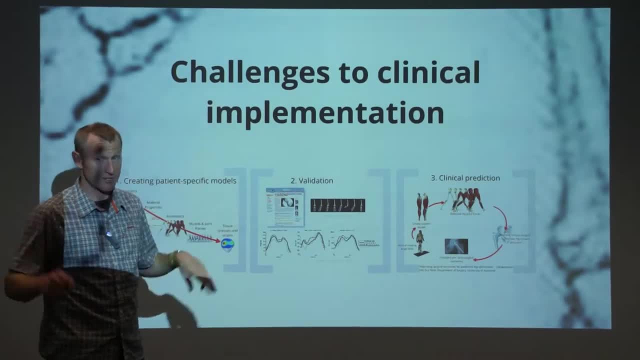 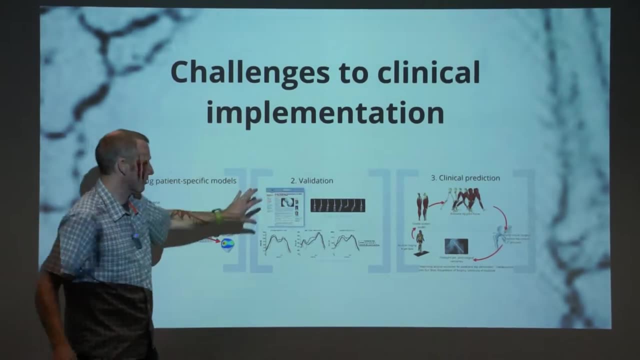 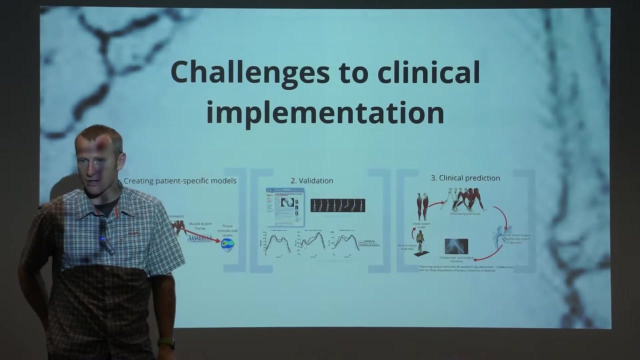 which we'll talk about. then I need some way of actually- hopefully experimentally- measuring those forces and then asking my model if it can reproduce those forces. so so that's a critical step. this steps really important to convince your clinical colleagues that what you're doing is going to be useful and can. 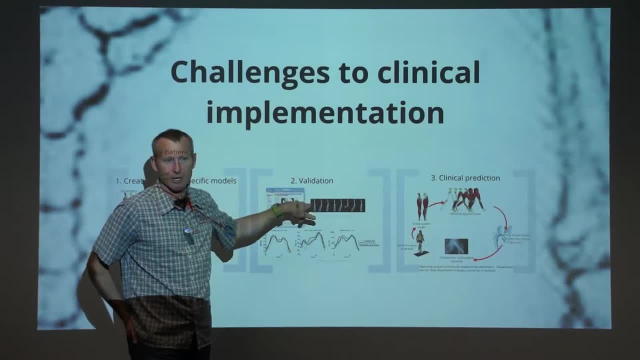 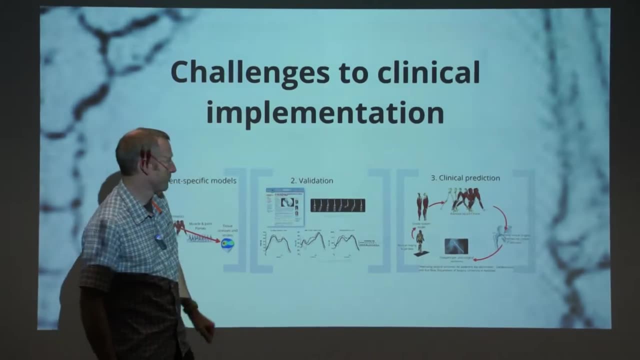 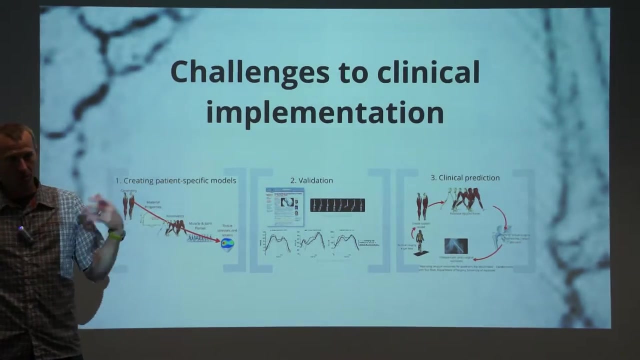 translate into the clinic, because if the clinician has doubts about your model, I mean that you're going to have a hard time convincing him or her to actually use this in a clinical setting. and then the final thing you need to do is show that our models are predictive, because if we can't predict new or or novel, 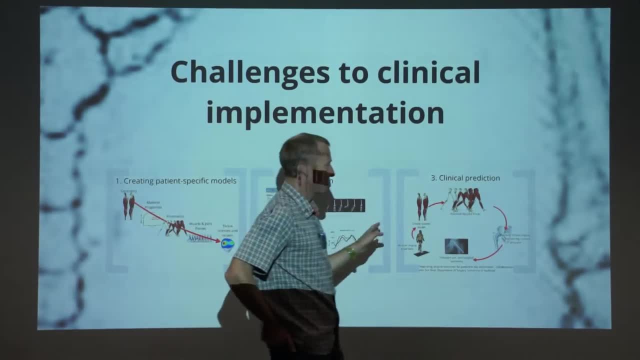 things with our model or come up with treatment strategies that we could test in silico within the modeling environment, then we can't predict new or novel things with our model or come up with treatment strategies that we could test in silico within the modeling environment. then 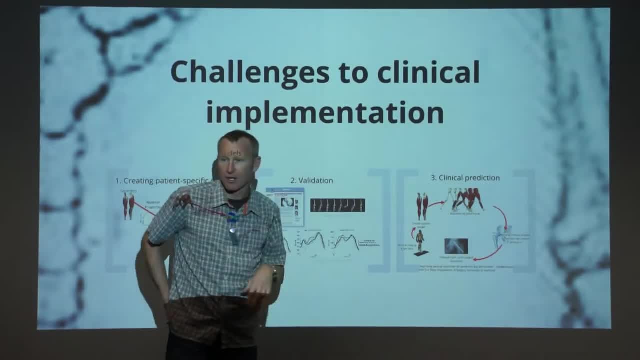 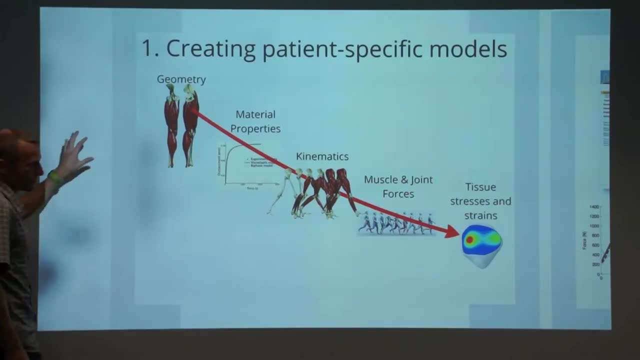 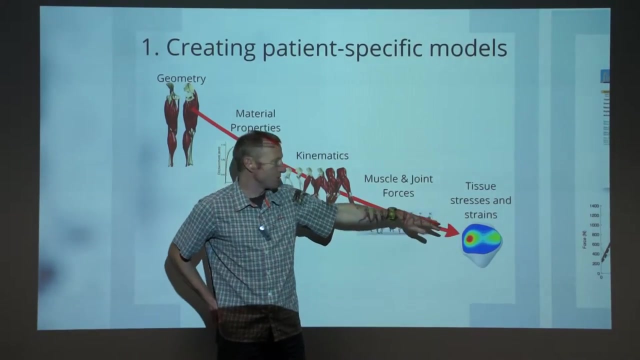 you know what use is the model, unless it's just to really understand a key biological question. okay, so creating subject: specific models. this is the workflow that we typically use. notice we're getting down to tissue level stresses and strains. you could push beyond that and you can go to cellular. 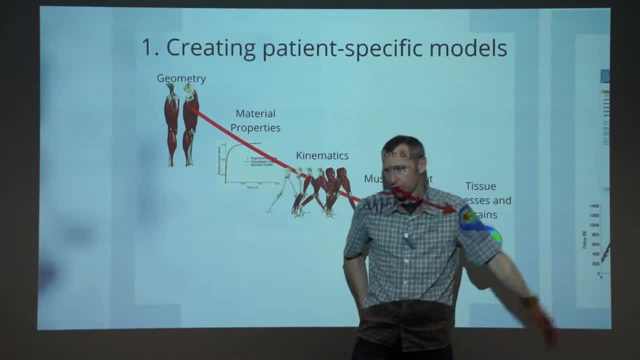 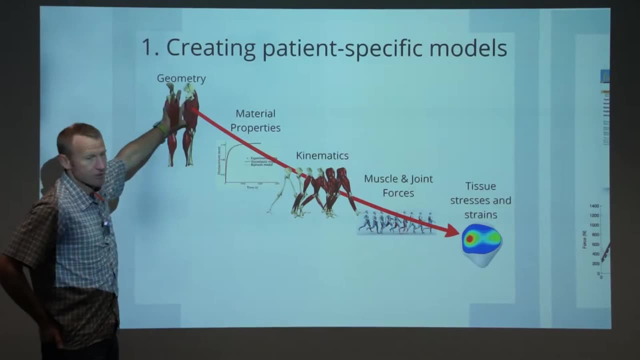 level. some of our colleagues do some cellular work or you know even further to molecular, but essentially the process and the workflow is very similar to what you've seen before. you're going to start off with some sort of geometry. you want to capture that, the geometry- and the geometry is very important. you want to characterize some. 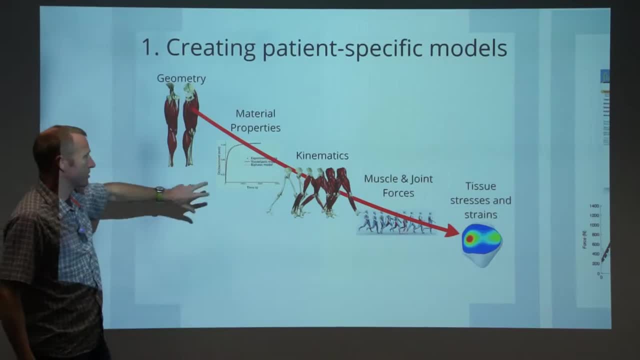 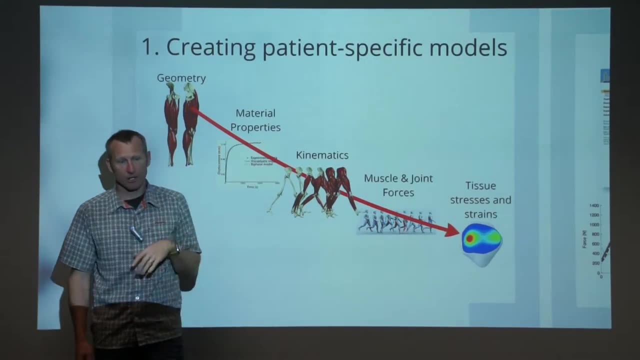 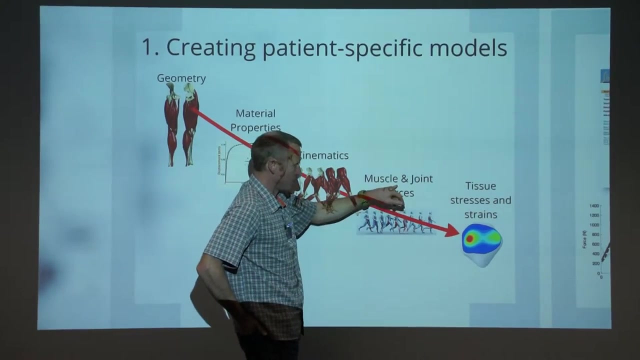 material properties of that tissue that you're interested in- you need to describe some loads and boundary conditions- and of the musculoskeletal system. we're talking, then, about the kinematics, typically, of of this multi-body segment system, which is our skeleton, and you need to describe the 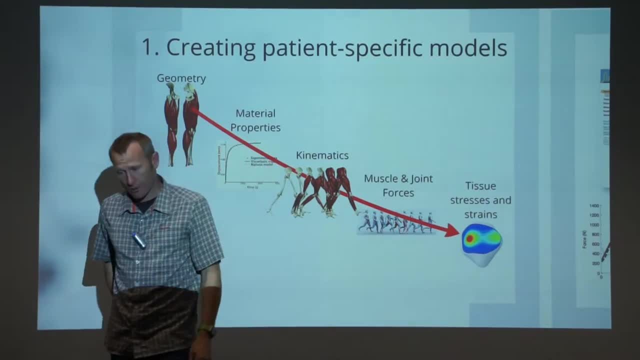 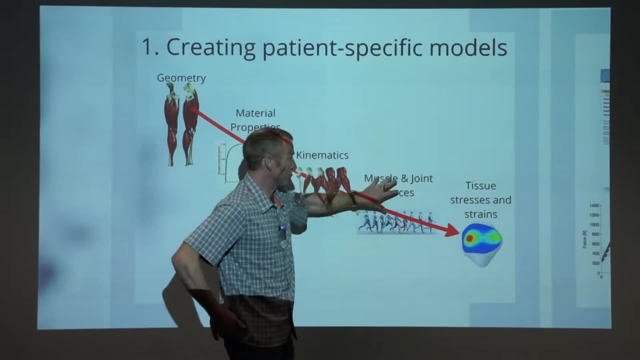 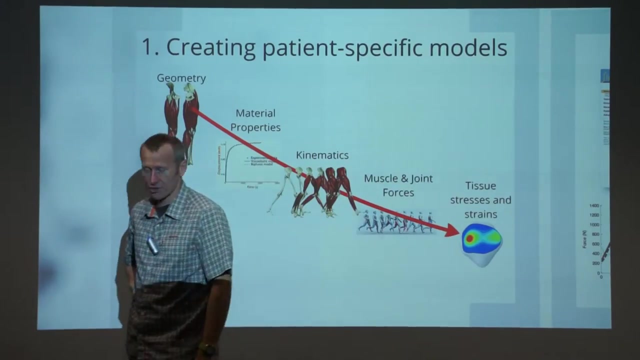 muscle and joint forces. the muscle forces are really what drive the internal contact forces within the joint, and so these are critical to understand and they're also very hard to get because you can't measure them directly and ultimately then end up in some sort of tissue stress. so this is an 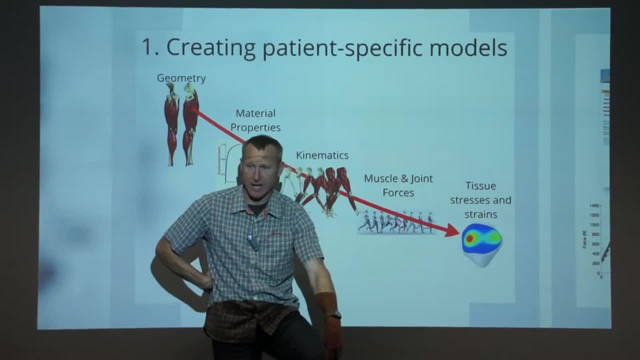 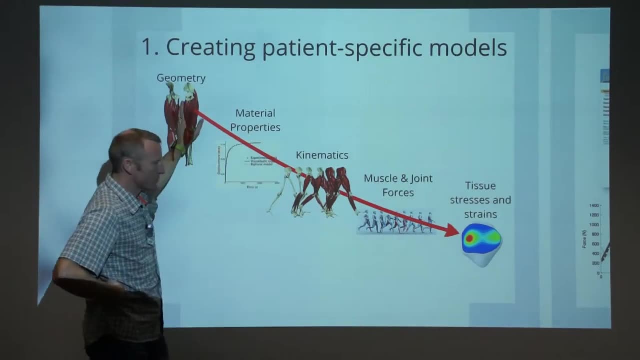 example of some work I've done on the patella femoral joint. you patella is your kneecap, so these are stresses within the cartilage of the kneecap. so we you know that might be a research question. we want to for an individual characterize. 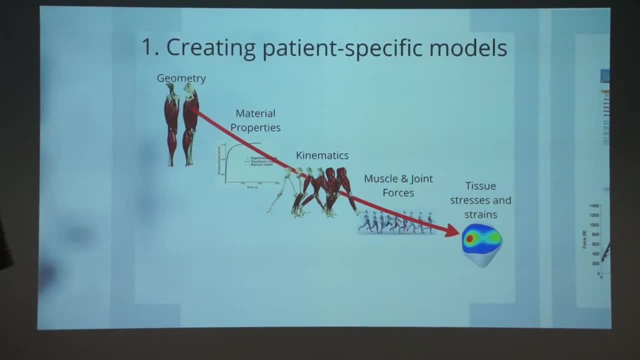 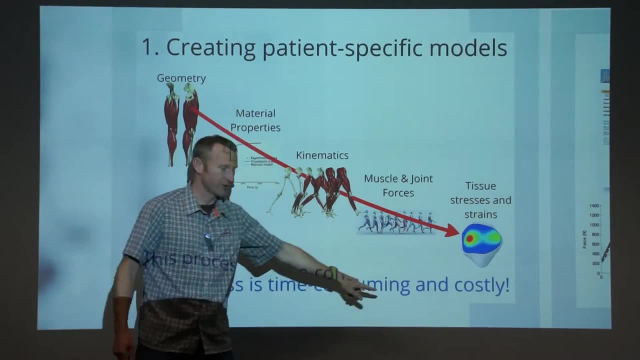 what kind of stress distribution there is in in the patella. so we want to understand what kind of stress distribution there is in in the patella. so unfortunately, this process is very time-consuming and costly. okay, these things obviously intimately linked. now, if it, if it's going to go into a clinic. 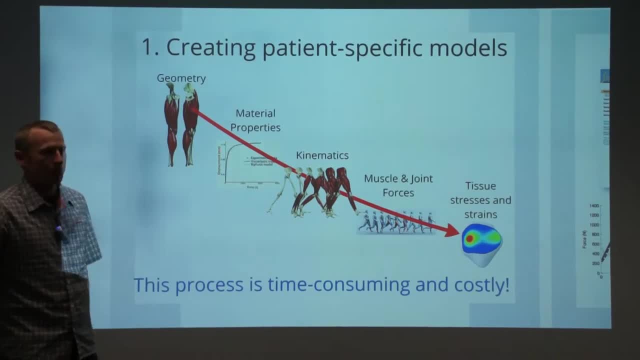 and you say, well, that's great, we can take these measurements potentially in the clinic, but it's going to take us three weeks to build our model and can't get back to you. it's not going to fly right in the clinical world. they're just going to say: forget it. so we need to address that problem. this I'll just talk. 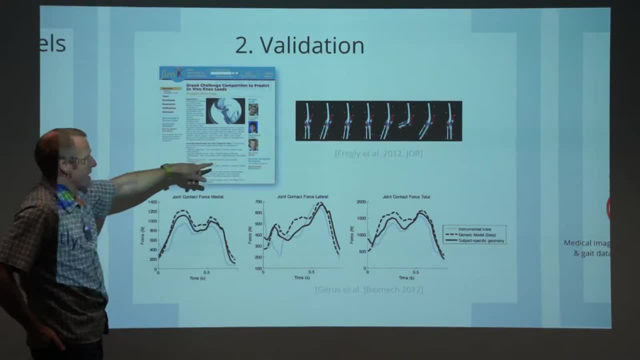 about in a project I've been involved in. it's called the granny challenge and it's with colleagues Dale de Lima, who's at the Scripps clinic in San Diego, and he has designed a knee joint replacement to have load cells within it. so, and then these knee joint replacements have gone into actual 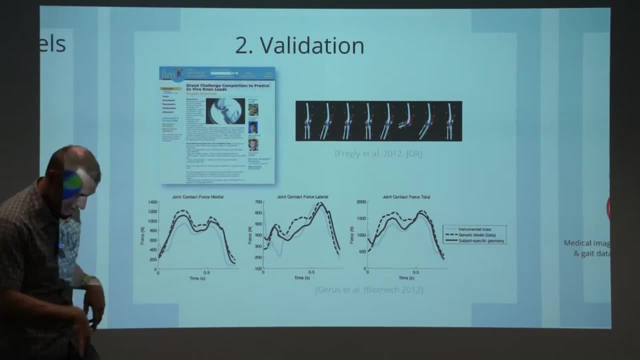 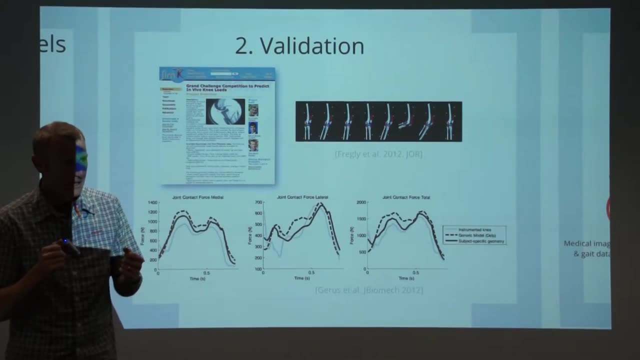 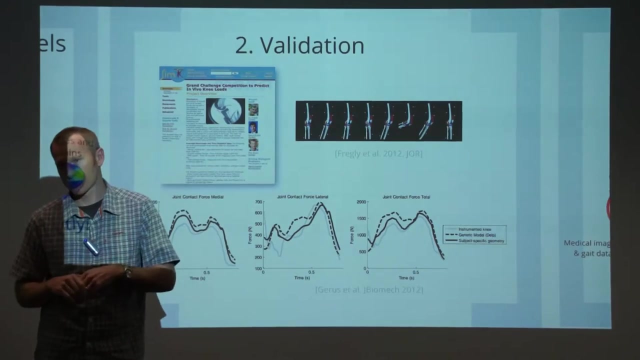 patients- four of them- and it's also down the stem of the tibia. there's also an RF coil that you can charge using an inductive power and you can transmit those forces out and capture them. so these people can walk around and we can measure the actual forces within their knee joint and BJ Fregley, who's at. 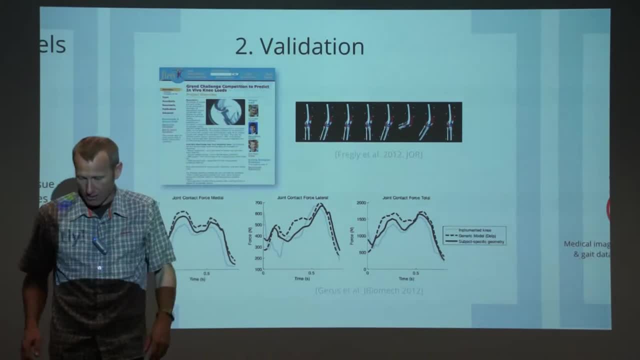 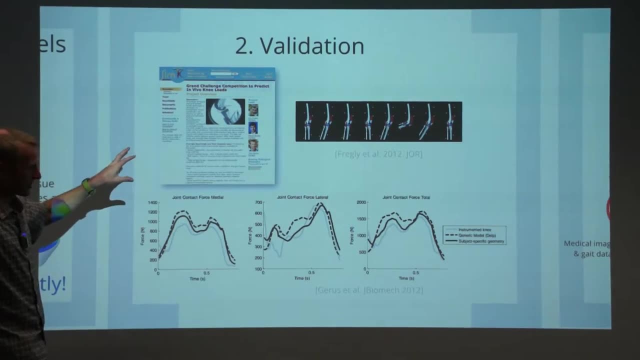 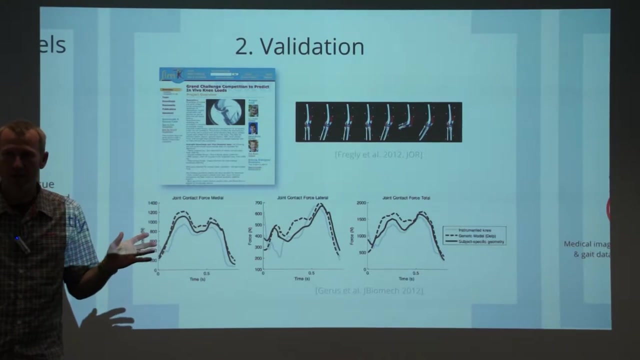 University of Florida, he Darrell and I had an NIH grant a couple years ago- that's it's just finished last year- to collect the data set on these patients and post this data to an online community, to the biomechanics community, and we said: you can have all of these patients in the clinic and you can have 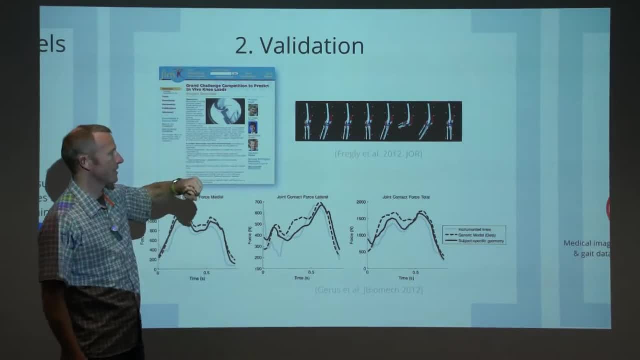 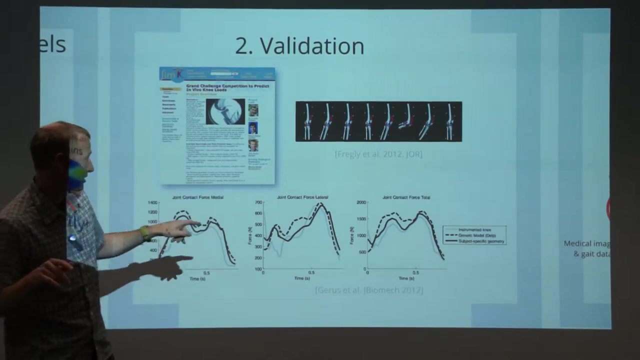 the information we've captured, from motion capture to geometry. we've reaction forces at the ground. we had people walking on force plates and we gave them everything we could accept, the actual forces that were inside the knee, and we said to the modeling community: how well do your models work to predict? 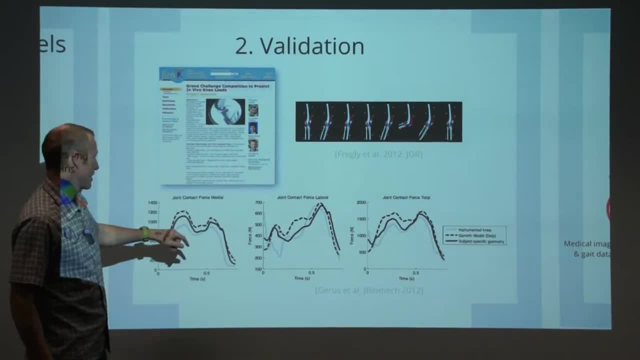 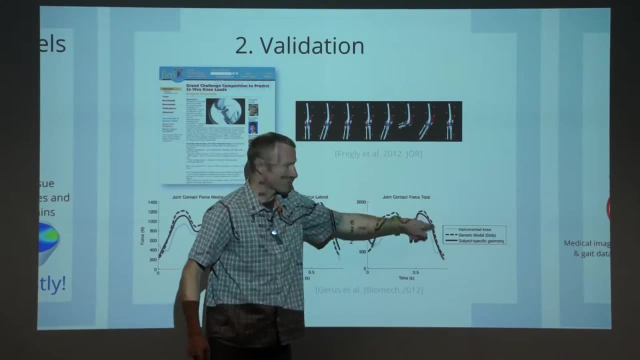 the internal forces of the knee. so these internal forces are on the medial side of the knee, so the inside of the knee, the lateral side and the combination of the two, so this is the total joint contact force. so these are some predictions that we're doing with our models, where we have some 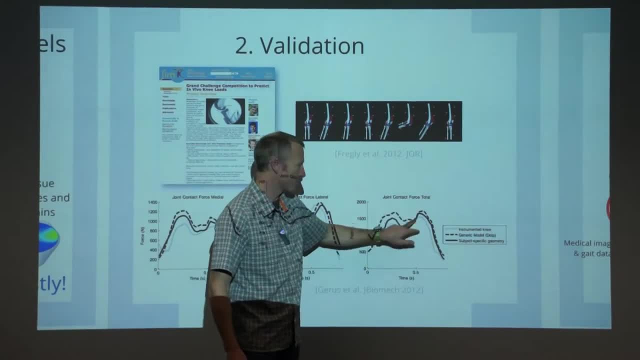 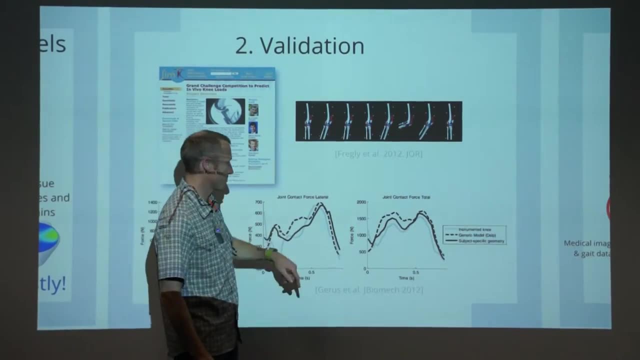 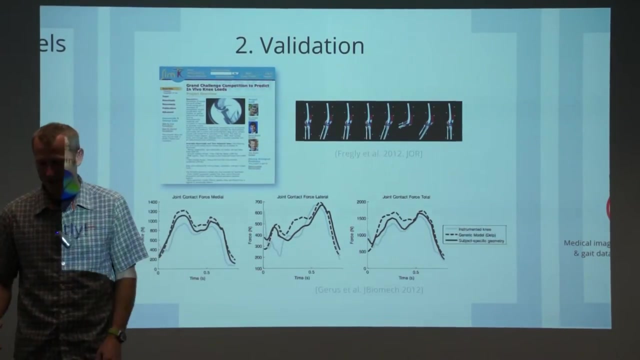 generic model which is in dash- the instrumented knee data is the gray- and then one which has subject specific geometry, and you can see the one with subject specific geometry does a little bit better. but the other thing that we've found from this exercise is that you know we we're kind of crappy predicting. 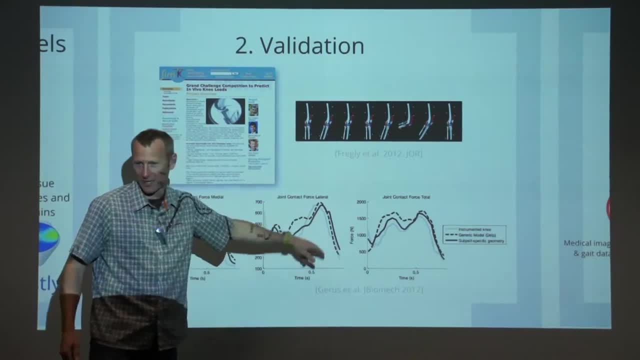 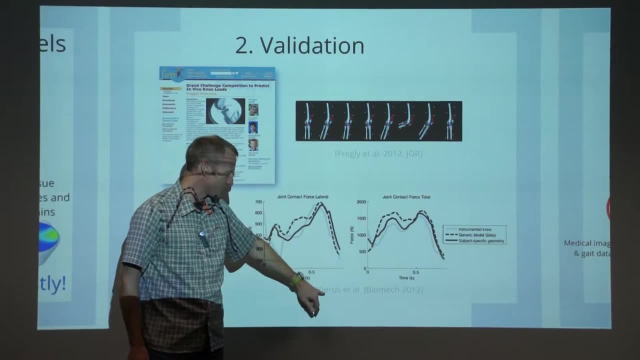 what the internal forces are. you know these are not exact predictions by any stretch of the imagination and the ones that we're showing here actually pretty good. this is from work that colleague- she was a postdoc, Pauline Juris with a colleague of mine in Griffith University and Pauline was. 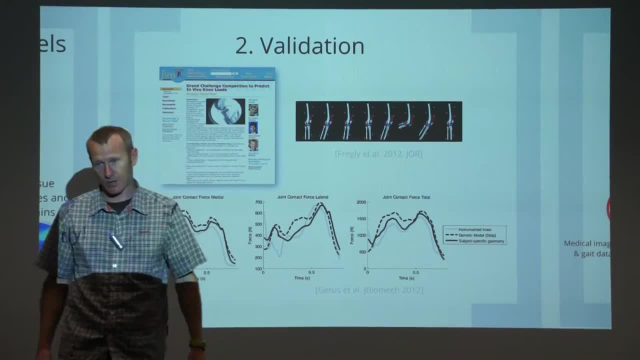 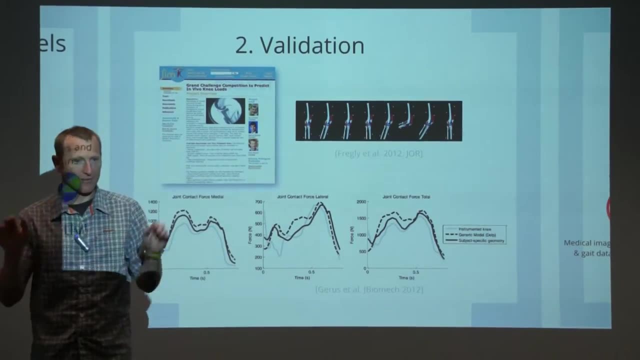 doing these simulations and these were pretty much, at the time, the best that anyone had ever done on predicting the contact forces, and already you can see well, a little bit off here, but nonetheless this is required because we want to test our ability of our models to predict the internal forces. okay, and 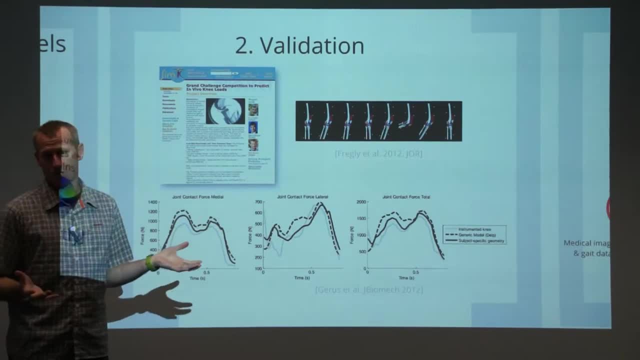 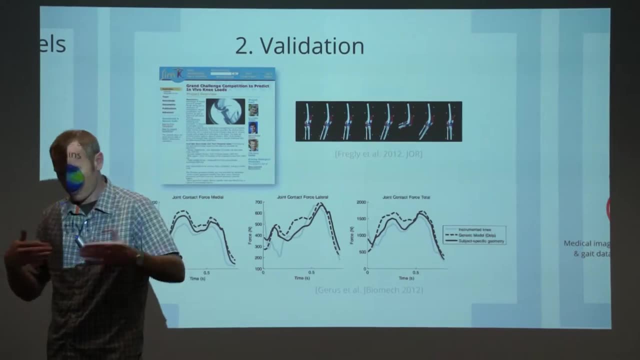 if we can't do that, then the use of our models is questionable. So there's been quite a lot of effort since then. this was published already four years ago and we're building on top of that, and it's only because we've made all this data. 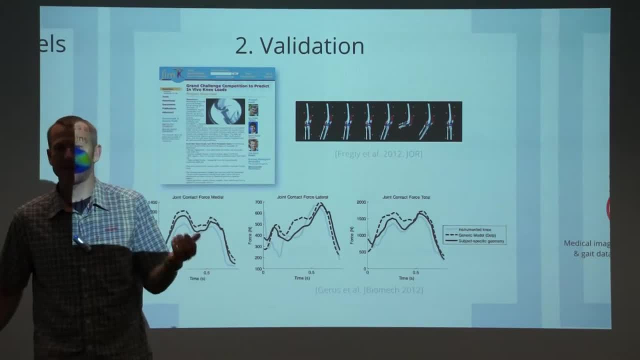 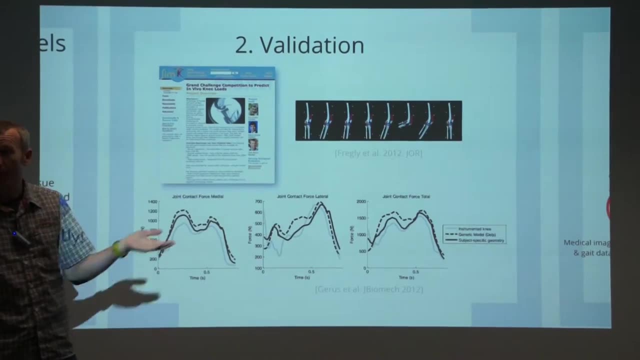 we had a competition, by the way, so you could win a prize at the end of it, and it's led to thousands of downloads of a unique data set, and we had this competition for five years in a row. every year, we'd have a new patient and a new data set. 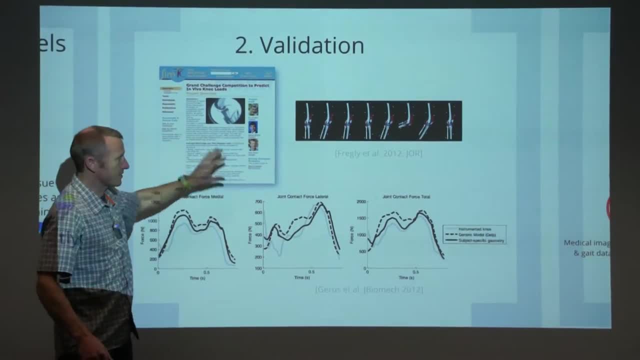 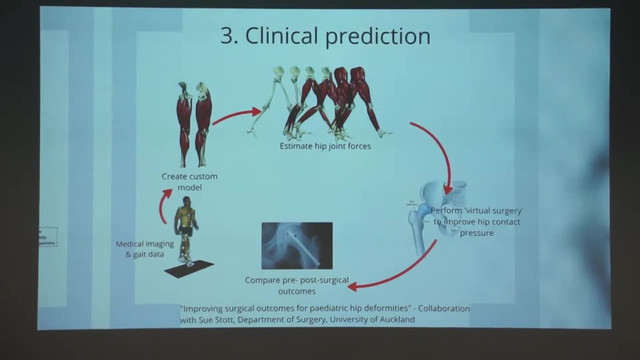 So that's been a really for the community, that's been a really good thing for us to be able to test our models Okay. so the final challenge is to then prove some sort of clinical utility of the model. This is a workflow, again, that you'll kind of be familiar with, and I'll get to that in. 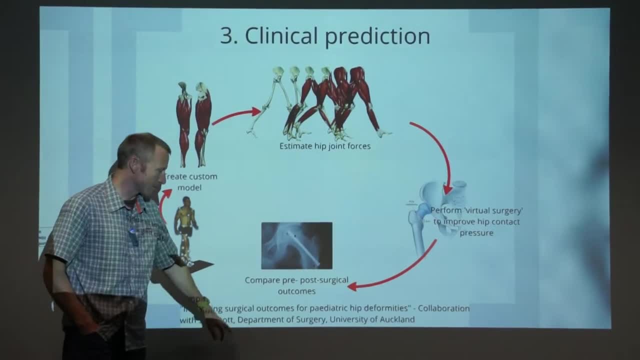 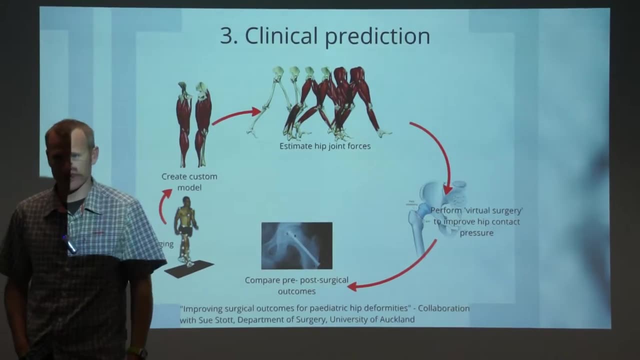 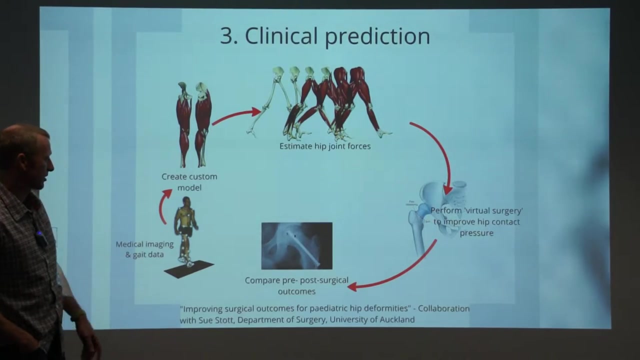 the next slide, But this is work that we're doing with Sue Stott, the Department of Surgery, and it's dealing with patients, Patients who have what's called slipcapital femoral epiphysis, and you'll have to remember that by the end of today I'm going to ask you on what that term is, but it's a condition. 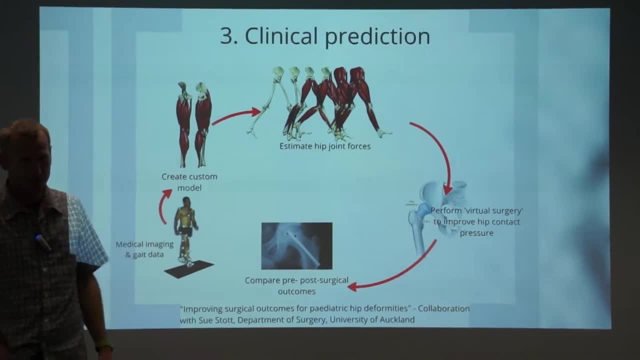 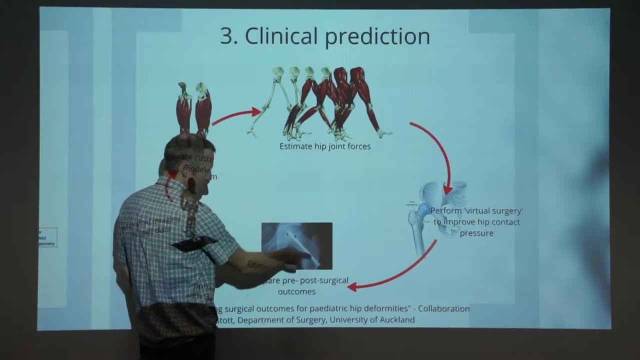 that affects young individuals whose growth plates have not fully developed, fully matured. and what happens is the growth plate here, this is the femur, this is the top of the thigh as it articulates into the hip joint, the ball and socket joint. and what happens? 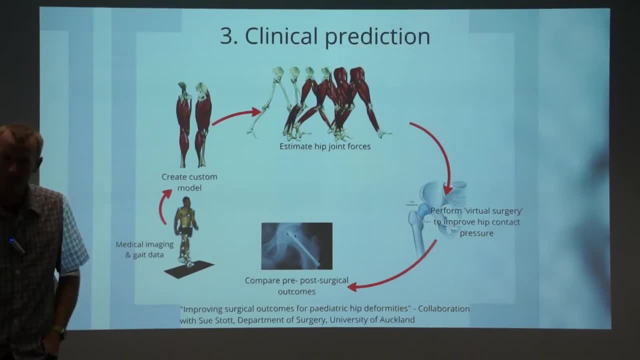 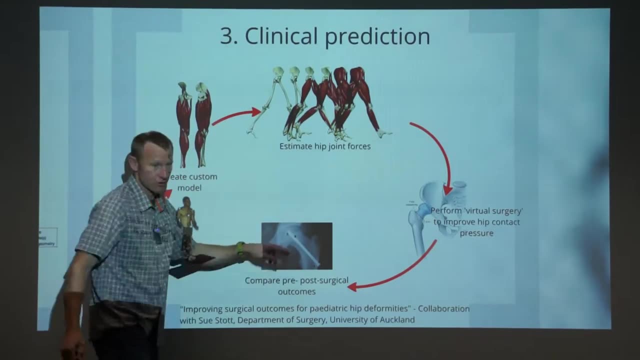 is in these patients, these young children who are typically overweight. obese children, experience really large loads and it causes this thing to slip. The surgeon says it's like an ice cream falling off: an ice cream cone just slips to one side. But, as you can imagine, this is a terrible thing for a 10-year-old to have, because there 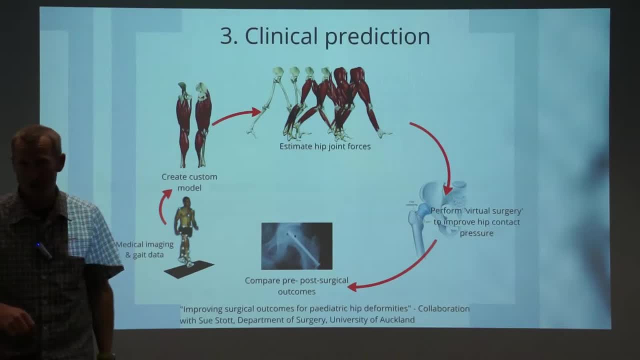 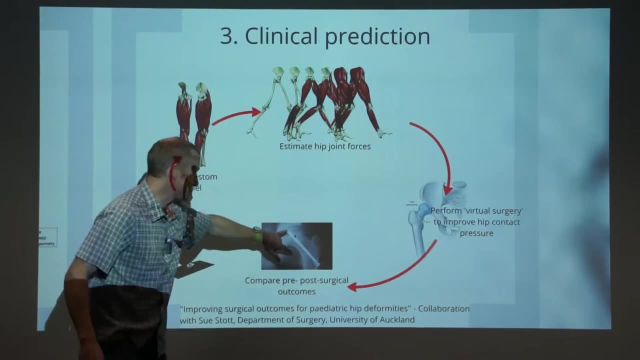 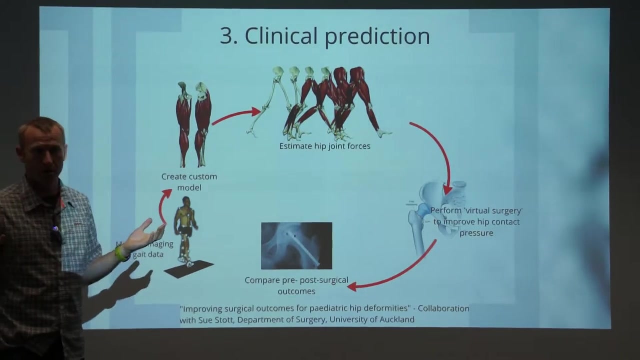 is nothing you can do to bring the joint back to its normal health. What the surgeon will typically do is grab this dirty, great big screw and go right through the bone and prevent it from slipping any further. But in terms of whether or not that surgeon has done the right thing, who knows? 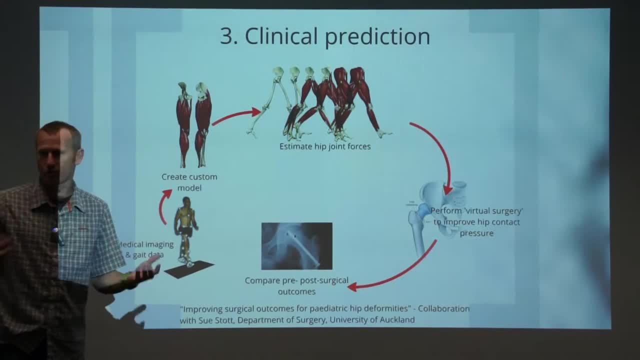 They're just using their intuition to say, well, we think we've done the right thing, But you only get one shot at this. this is a child, 10 years old, and you're doing orthopaedic surgery on them. So what we said is: look, why don't we take some medical imaging data and some gait data? 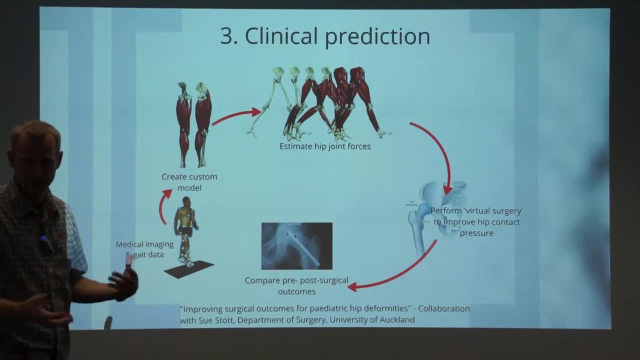 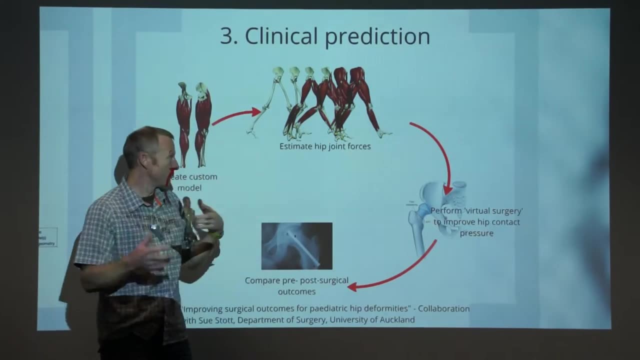 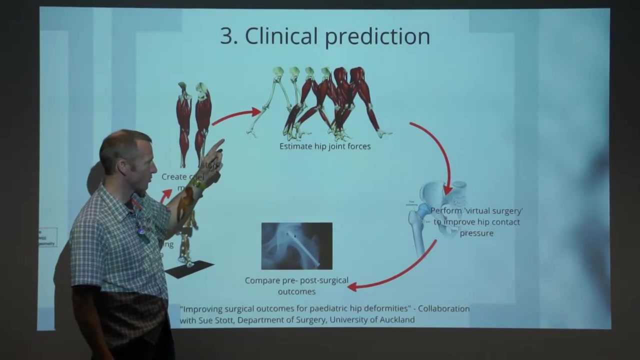 get these patients to walk around inside a lab where we can measure the way they move. We can customise a model And we can then Have a model that predicts the movement and estimate what the forces are in this joint. And if we can reconstruct the anatomy of the joint and provide forces, we can do a virtual 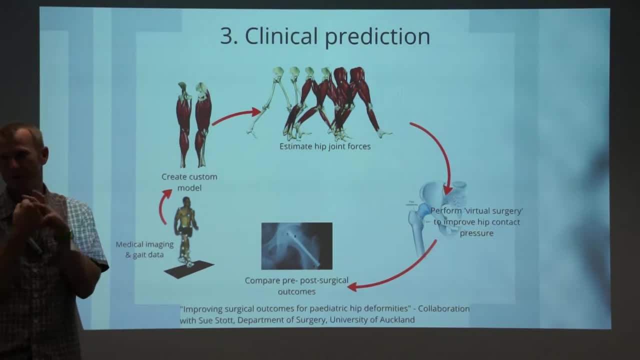 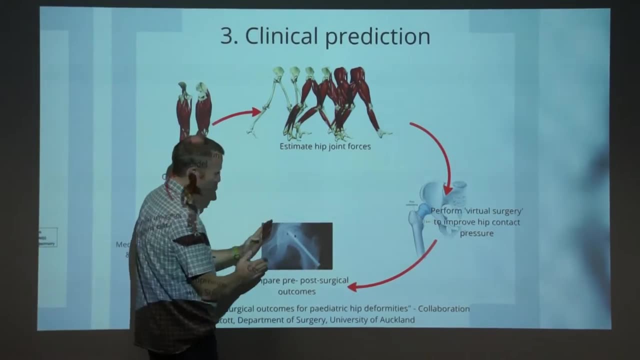 surgery We can actually in silico put the joint into different positions and orientations and see what the stress distributions are, See if there's a risk of further slipping. Rather than just pin this joint, should the surgeon maybe cut a wedge and do an osteotomy. 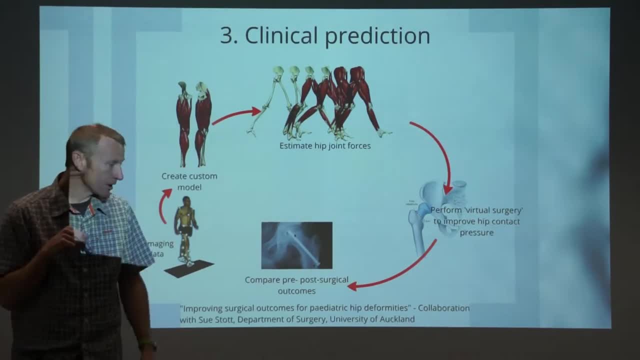 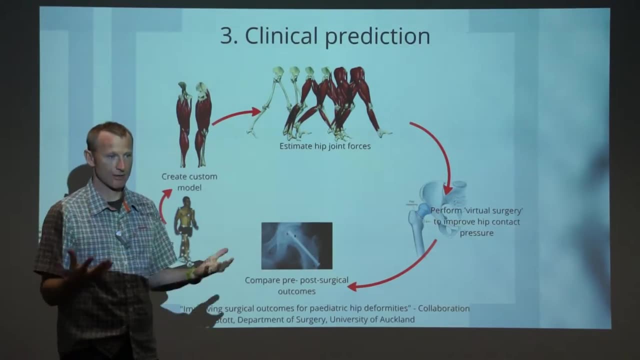 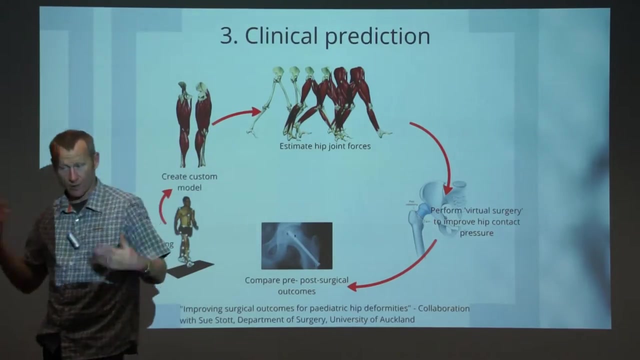 and rotate the joint to try and realign it, And these are questions the clinical community has no way of solving right now. And this is really where a model becomes critically useful, And this process, of course- because it's all in silico- can be done iteratively. 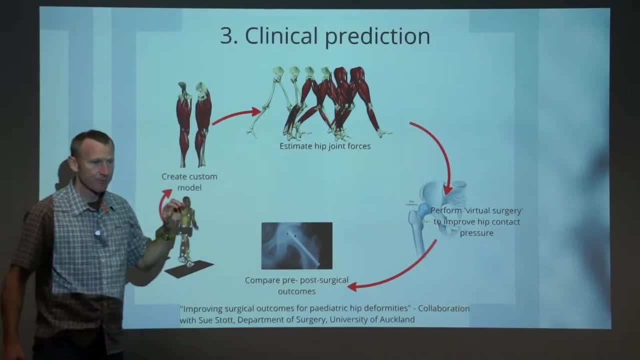 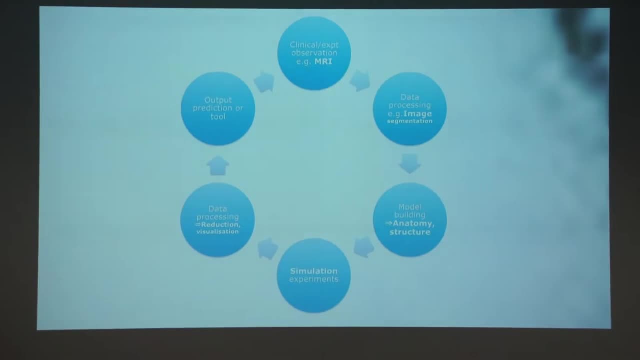 You can do design, optimisation and you can try and find the best outcome on a virtual patient before you actually go and do the real deal. So that's just a kind of a snapshot and an example. So this is a slide you've seen before. 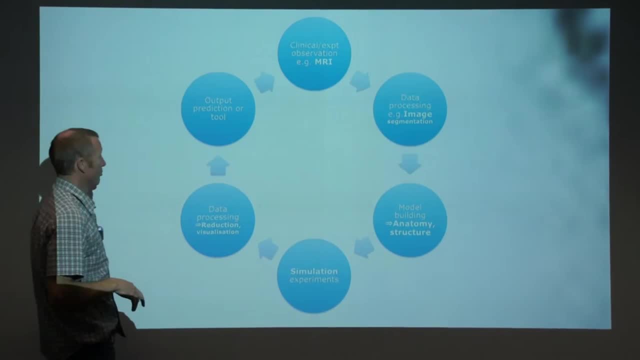 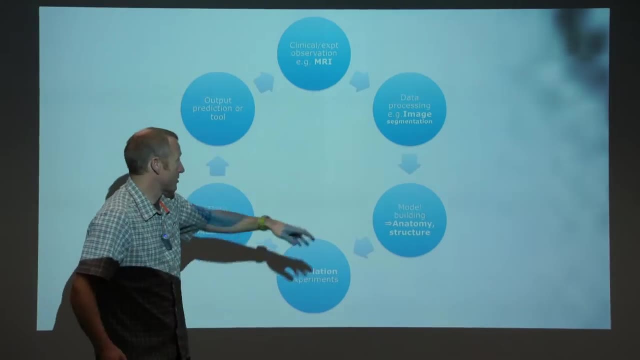 And this is all the same stuff, right? We're basically doing some observation, doing some sort of processing on the data that we've got. It might be segmenting out the data. it might be processing motion capture, movement, kinematic data. 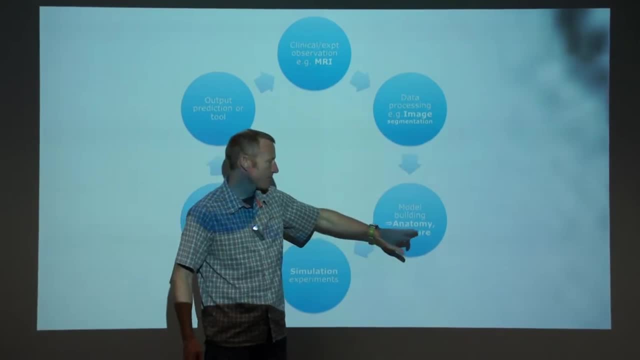 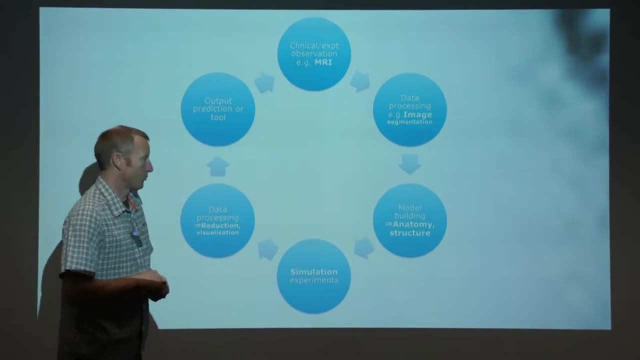 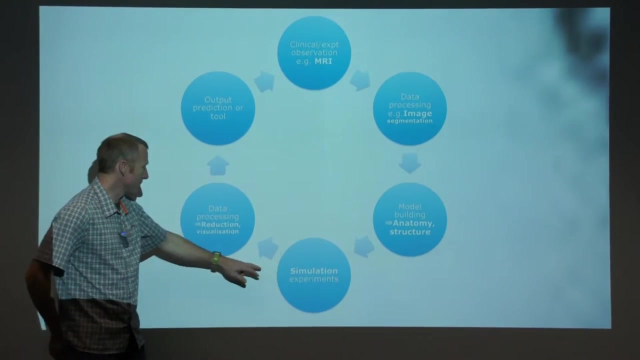 You build up a model, and that model includes the anatomy, the structure, as well as the critical components like the material properties, whatever's important to characterise in that model. You perform some experiments, and these could be in silico, then simulations. You might then visualise the data. 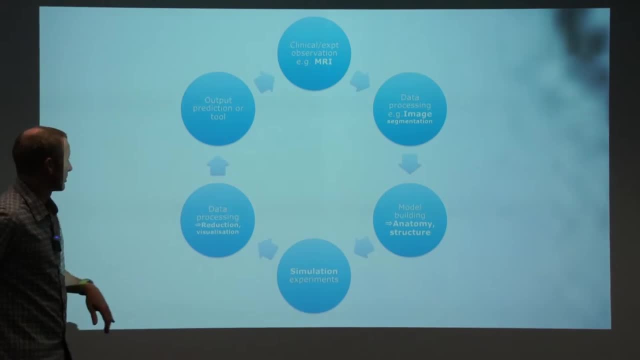 You might do some data reduction- and I'll talk about that as well a little bit later- And do some prediction and go around again. So it's exactly the same process and you've already seen that, so you're kind of familiar with what's going on here. 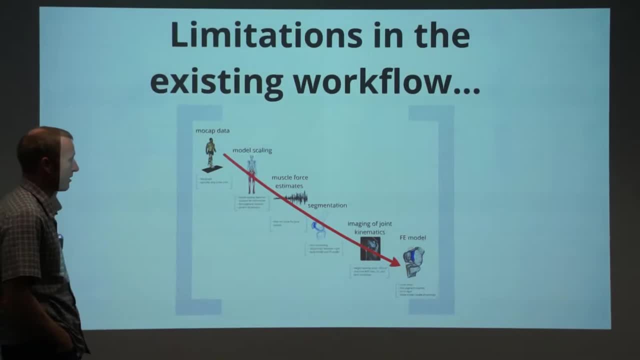 So there are some limitations to the current workflow that we have, and I thought it'd be nice to talk about them, Because this is setting the scene, then, for our group and what we're doing to address these limitations and move forward. So here's our workflow, right. 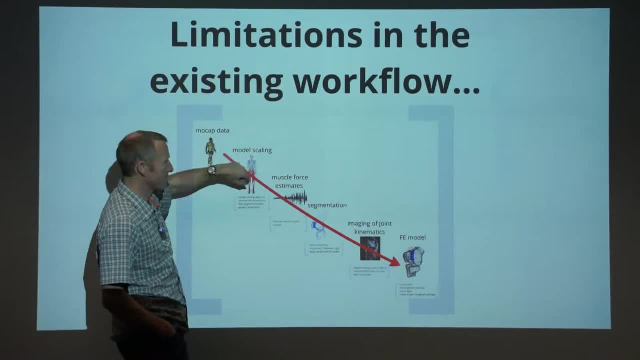 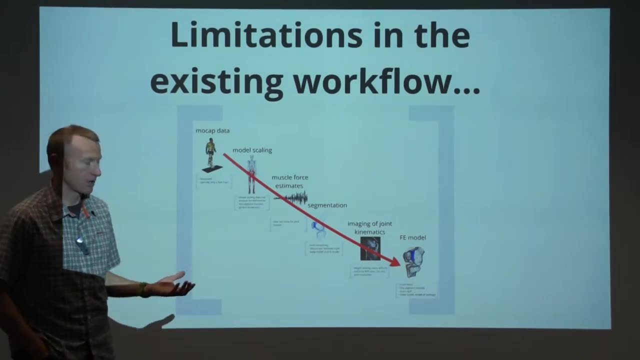 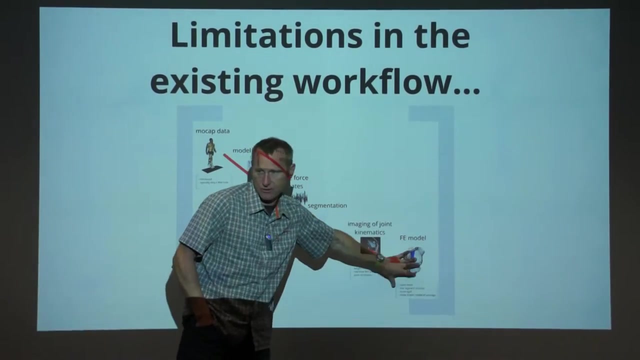 In terms of getting from some experimental data to creating models, to estimating loads and boundary conditions, down to creating a model of the tissue. And, of course, we're now in the finite element domain. We're using continuum mechanics to solve tissue related stress strain. Okay, 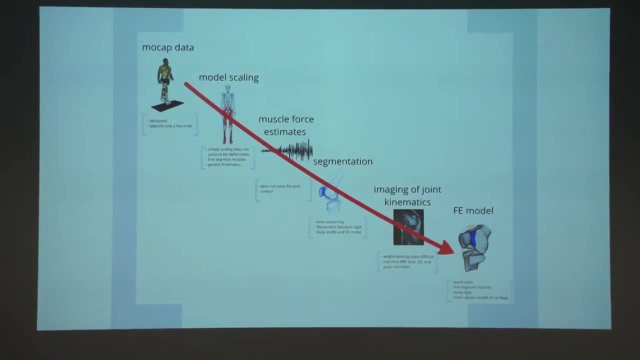 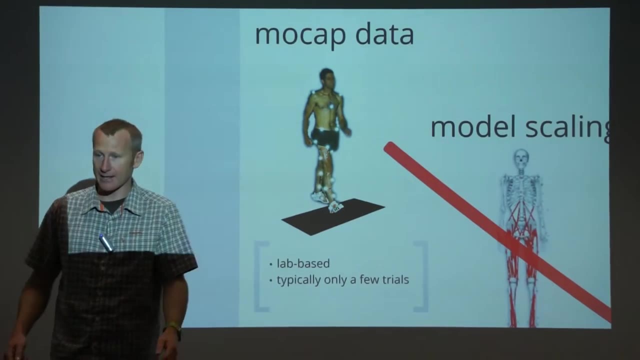 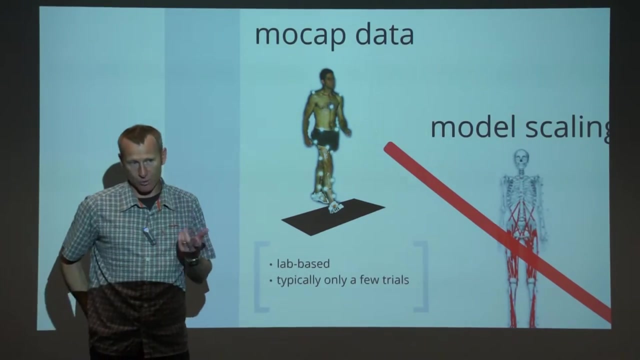 So here are the limitations. First of all, we typically get information from our subjects from motion capture, So we've got little markers that we do optical tracking with in a gait lab. You're constrained to be within a lab, So we might get children with cerebral palsy and this has happened. 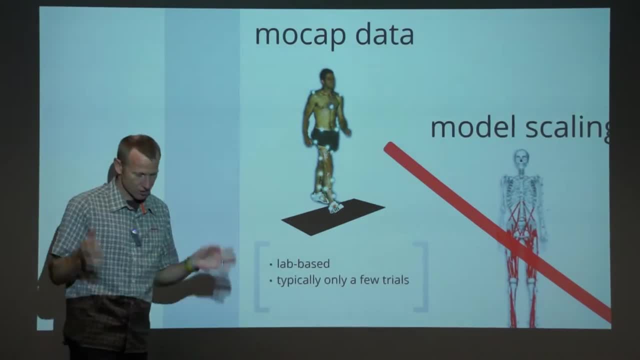 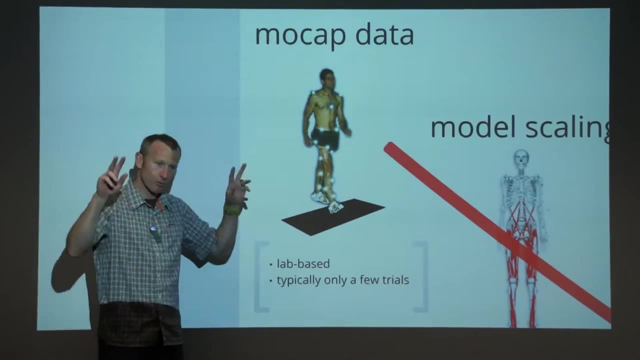 This is, you know, real life scenario. We ask the child with cerebral palsy. it's a neurological condition and these kids have trouble walking normally. So we take the child as small as they can in the lab and they walk across some force. 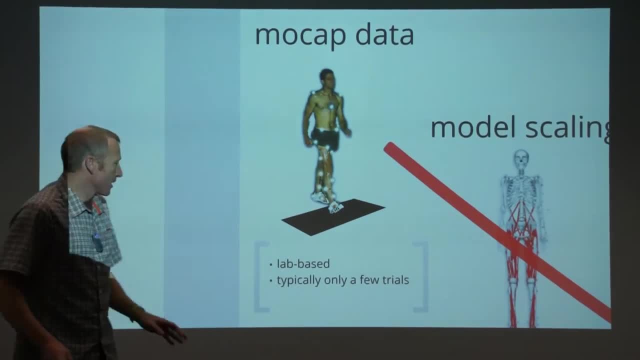 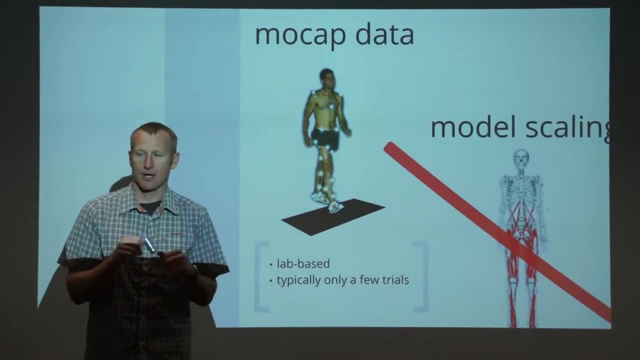 plates, We measure the forces, We capture their 3D movement And we take that snapshot from, say, three or five trials and we say this is how this child walks. And we say to the child: thanks very much, That's great. 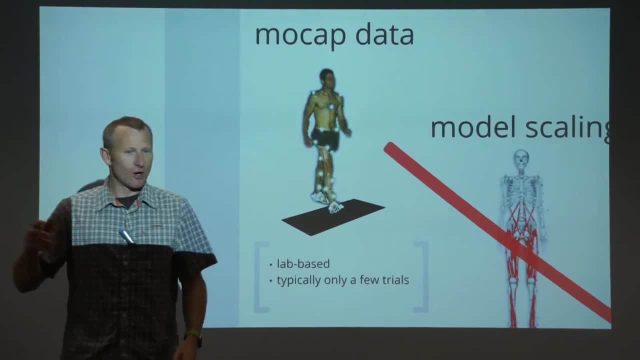 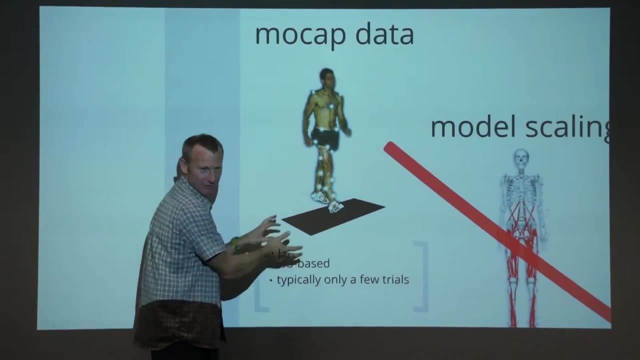 We've captured our data, Then they're free to go. The child kind of hops and runs outside and goes and plays basketball. I mean, this is a child with CP and we're characterizing them from a lab trial. that's very synthetic, It's not real. 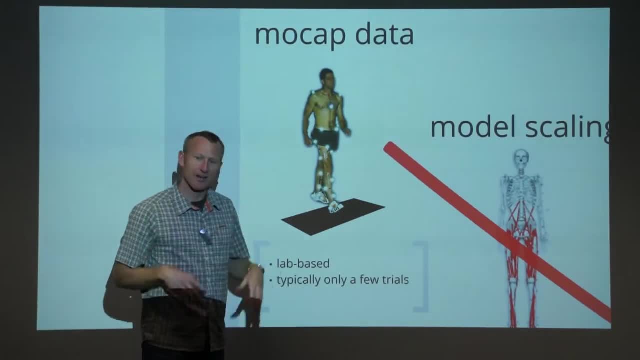 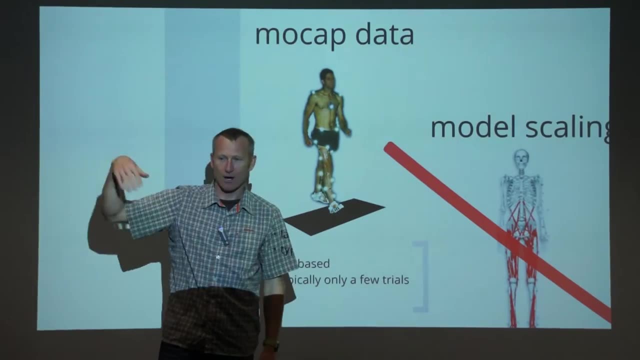 It's a real world And we're extrapolating this information to say, yeah, this is, in general, the loads and boundary conditions on this subject. What they do in the real world. they run upstairs, they go, hop curbs, they do all kinds of different. 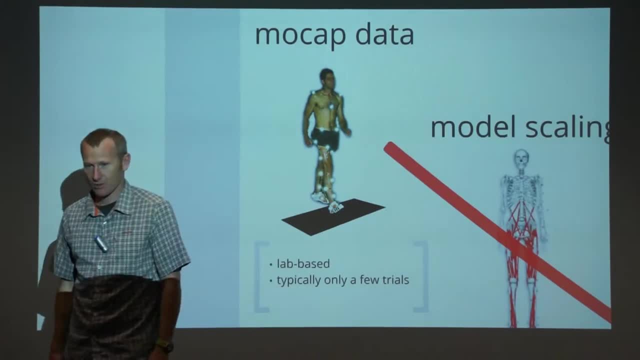 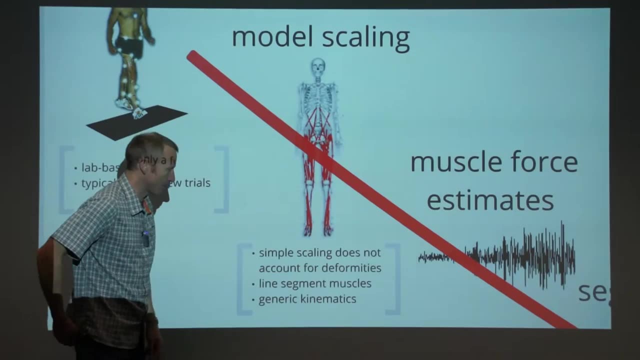 things that have nothing to do with what we've measured in the lab. So this is a problem and we need to address this problem. The second problem or issue that we've- this is more of a problem with the rest of the world, because they do it wrong. 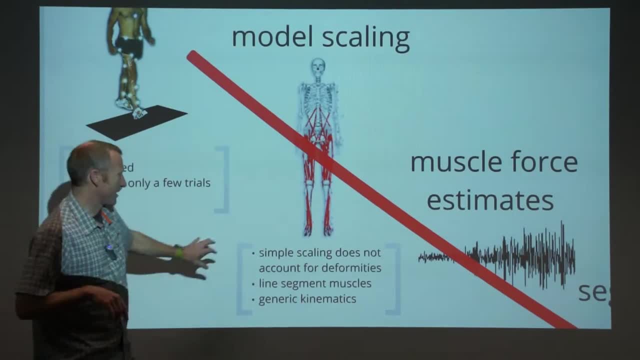 But we do it much better. here Is the rest of the world currently have these models. These are rigid body dynamic models. They make assumptions that the bones are treated as rigid bodies so they don't deform. That simplifies computational modeling a lot. if we've just got rigid bodies. 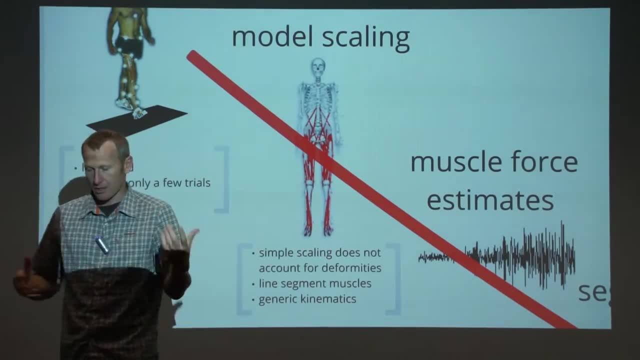 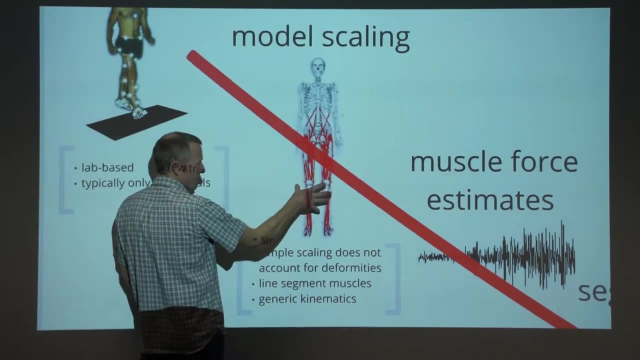 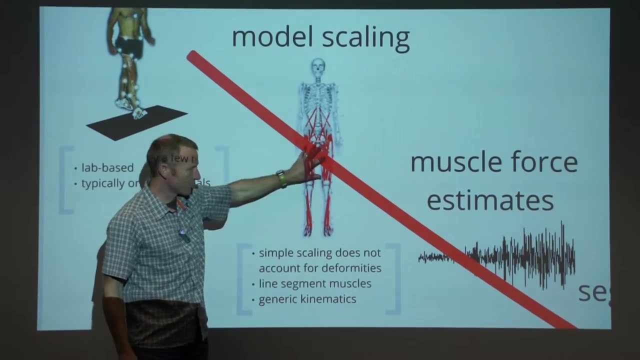 And the question here is: well, these line segments that represent muscles are going to give us our forces and boundary conditions And the way that we get to our new job. Yeah, New geometry here you know 90, 99% of the population of biomechanics researchers who 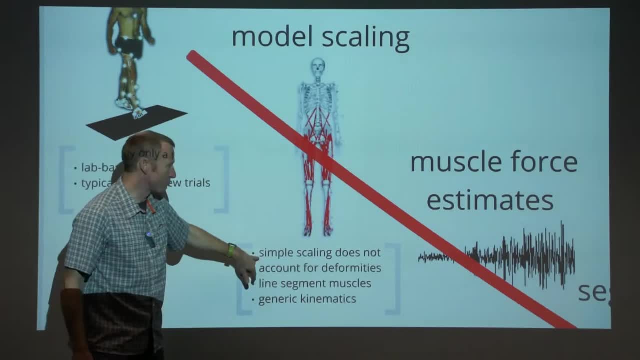 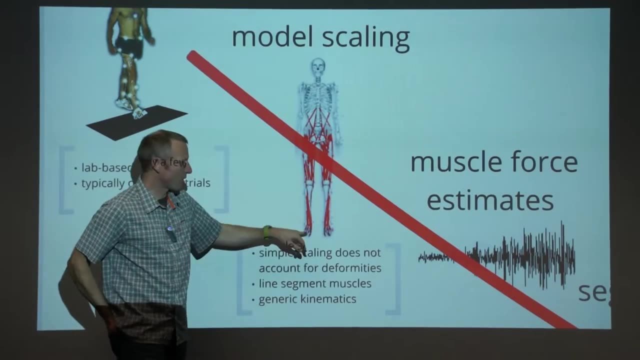 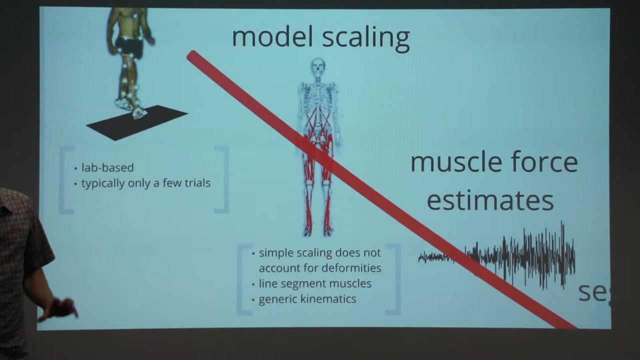 do these type of simulations will do some simple linear scaling to fit the geometry. Okay, So there's a software that's very popular. It's called OpenSim. It's developed by colleagues of mine at Stanford and it's about 10 years on now. 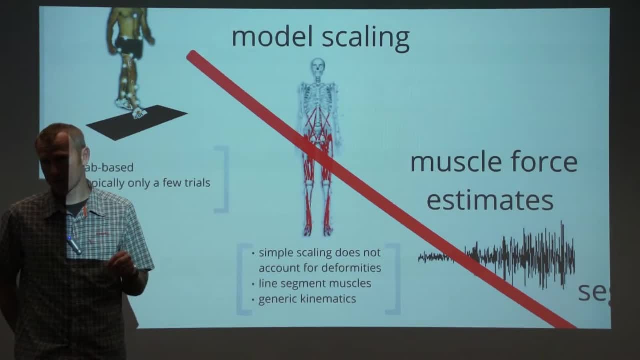 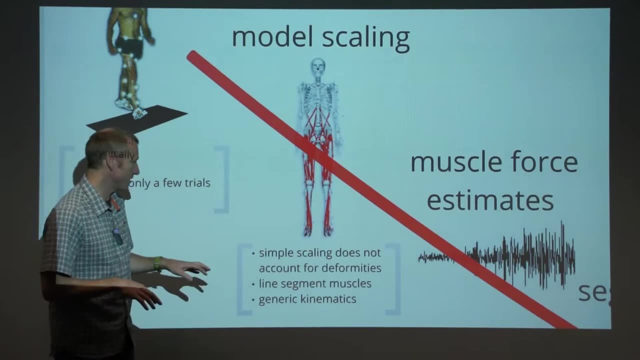 And there's about a community of three and a half thousand users worldwide. So there's, It's been well adopted by the community. That may not sound like a lot, but in terms of you know other like-minded geeks around the world, there's quite a few of them. 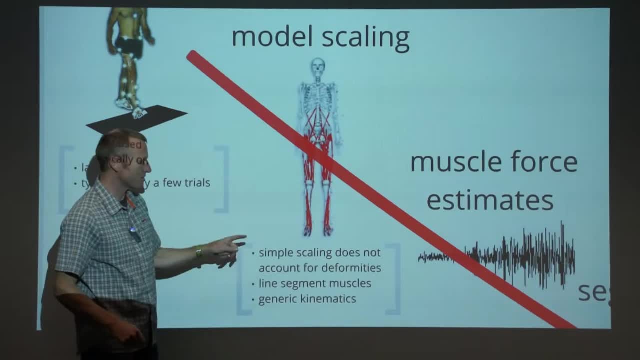 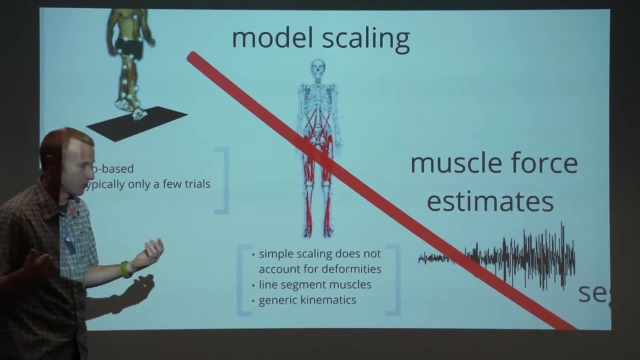 And they're doing this simple scaling. The problem is that simple scaling does not account for any of the normal variations you get in bone shape and structure. Okay, If you linearly scale your pelvis in all three dimensions, you're not capturing the fact. 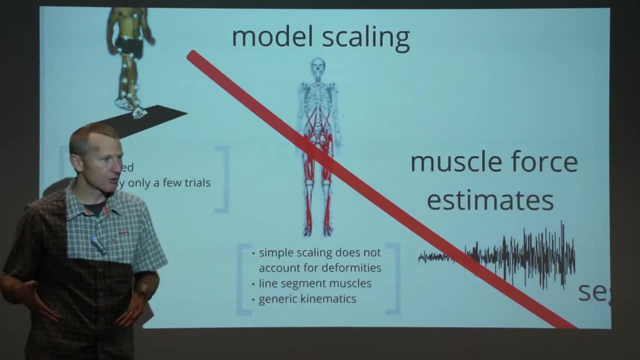 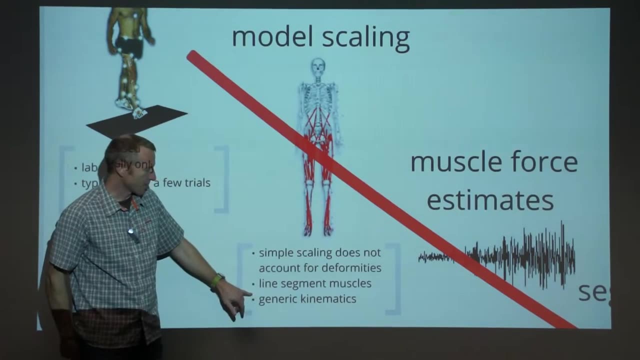 that. well, you've got a female pelvis that's quite different looking than a male pelvis. Okay, None of that's captured in there. So the other thing that's interesting is- and I'm guilty of doing this too, Don't get me wrong- 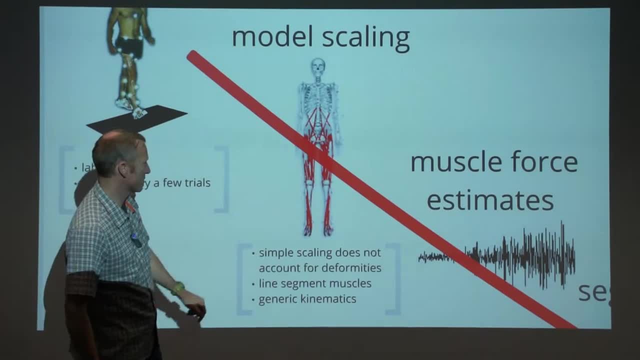 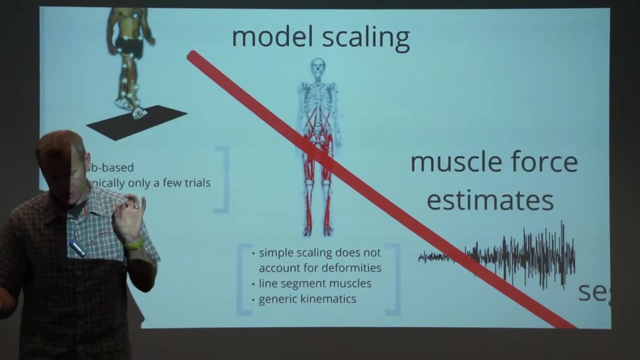 I mean, it's only up until recently that we're getting tools to kind of address this and do a better job. But the line segment muscles are kind of treated to show the line of action of force of the muscle And we all know our muscles are volumetric. 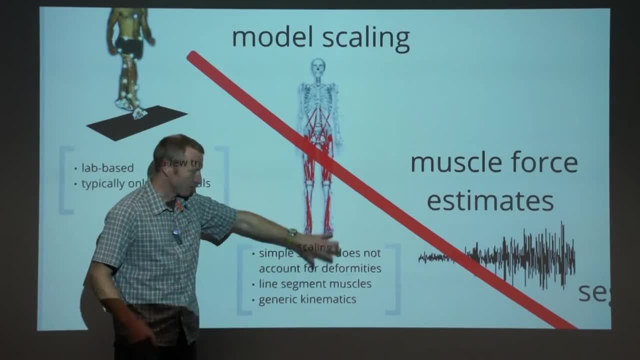 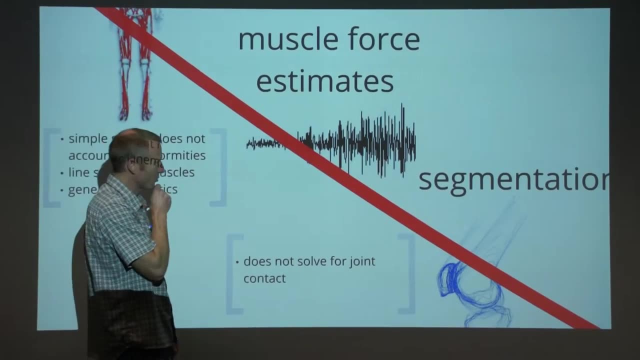 It's much more complicated than that, But you know, for now that's gone. Okay, That's kind of been the de facto standard and it's an issue we need to address When we solve for our muscle forces. often. again, this has only changed in the last five. 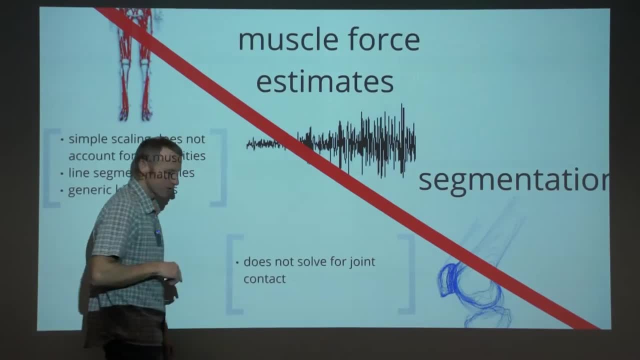 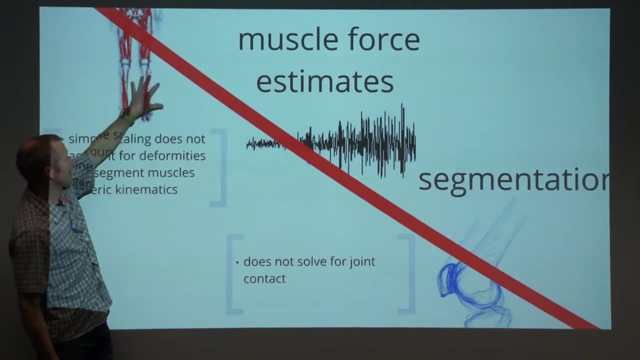 years or so. often we don't solve for things like joint contact And I'll give you an example around the knee joint To simplify the modeling of the knee joint. in this kind of domain, in rigid body domain, you might treat this as a mechanical hinge joint. 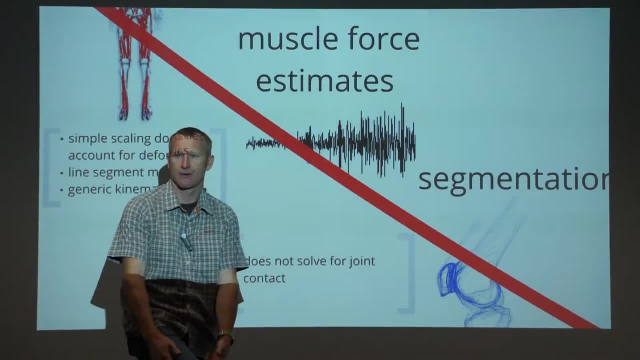 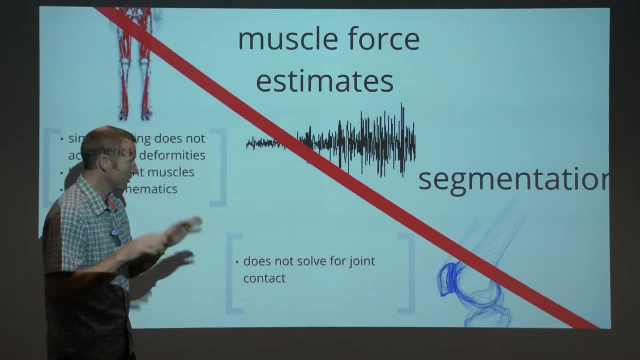 You might say it has one degree of freedom. It can only flex and extend. The real joint has all six degrees of freedom. It can translate, It can rotate in all three directions. But for simplification we're just going to treat it as a hinge joint. 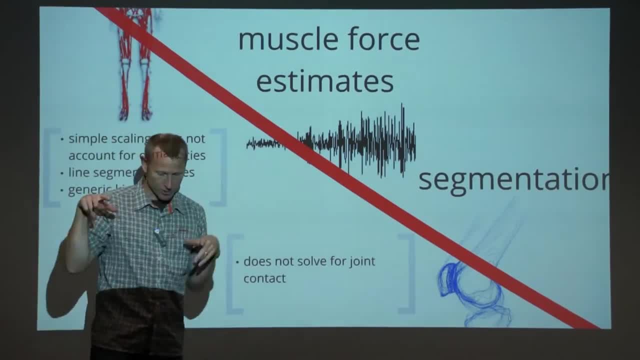 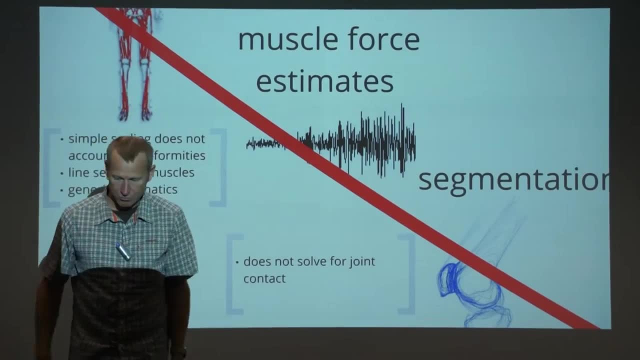 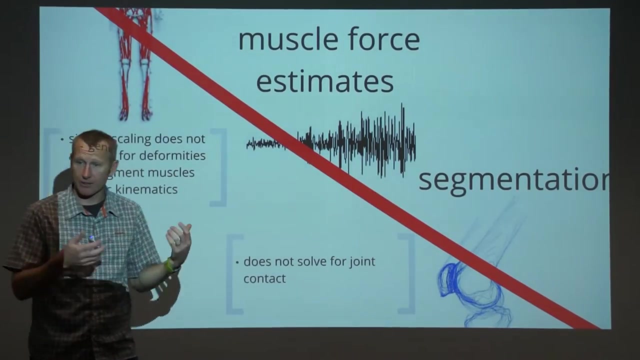 If we model it as a hinge joint and we say, well, these muscle forces have to produce this movement, we can derive equations of motion. okay, and we can be consistent with Newton so that he doesn't turn in his grave. so F equals MA. we can calculate these forces. 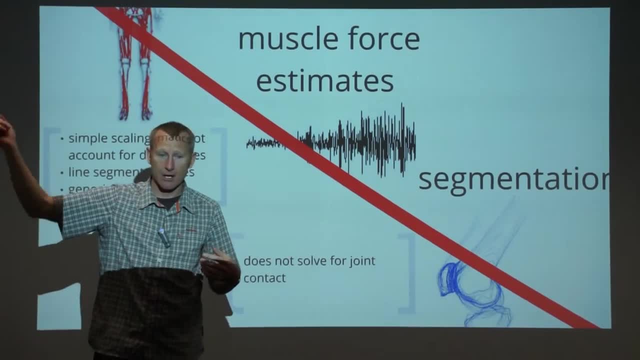 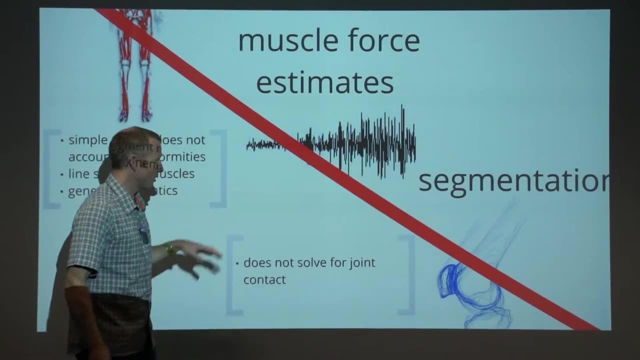 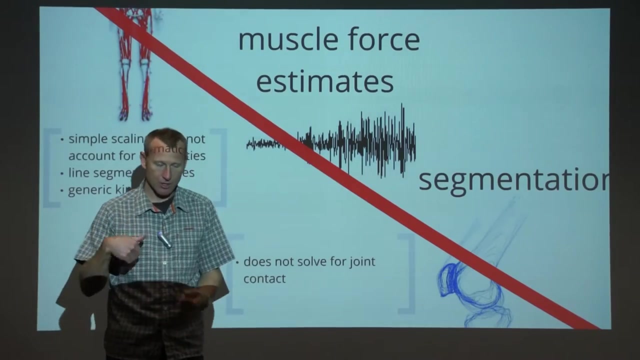 we can calculate the segmental accelerations, we can integrate forward in time and do a dynamic simulation that predicts the movement forward in time And we can say: well, we predict these forces give rise to this movement. Now you could imagine if you've got a pin joint here, you can imagine a variety of muscle. 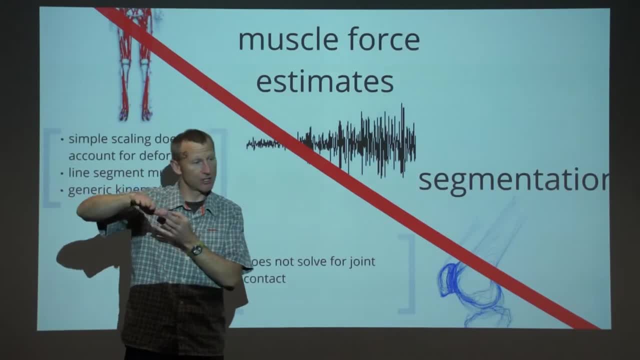 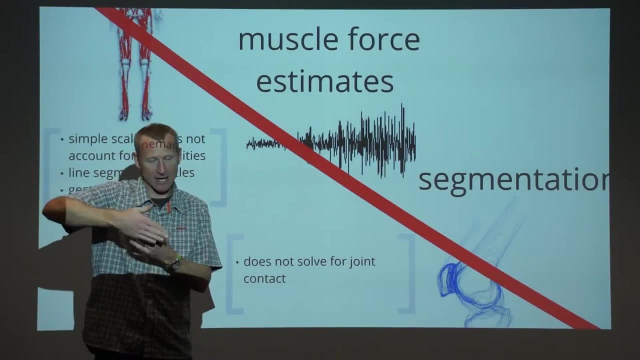 forces that give you the same net flexion extension movement. But if you suddenly had a different degree of freedom in there, if the knee could suddenly abduct and adduct, the same set of muscle forces that you could derive for flexion extension suddenly now cause the knee to spin sideways right. 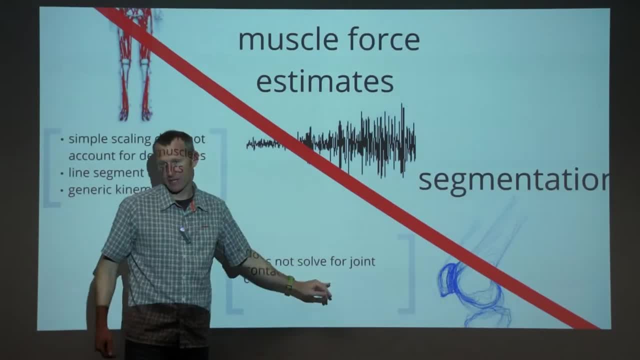 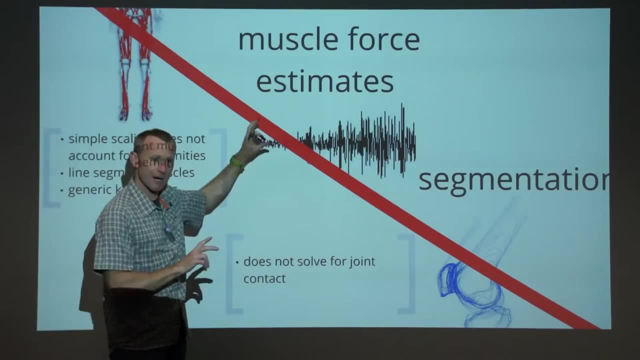 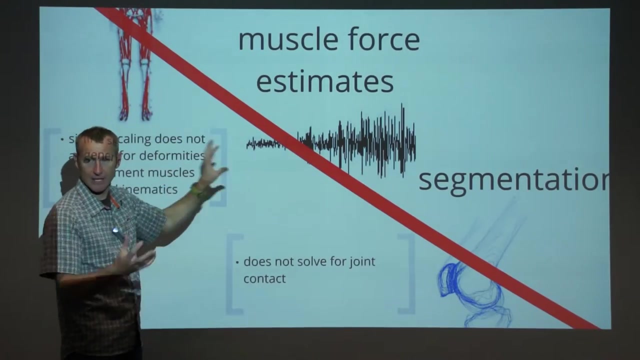 So if you provide these degrees of freedom, you very much constrain the possible set of muscle forces that you can get. But right now we don't do this. We don't couple between a contact simulation and a rigid body dynamic simulation. We typically have these decoupled. 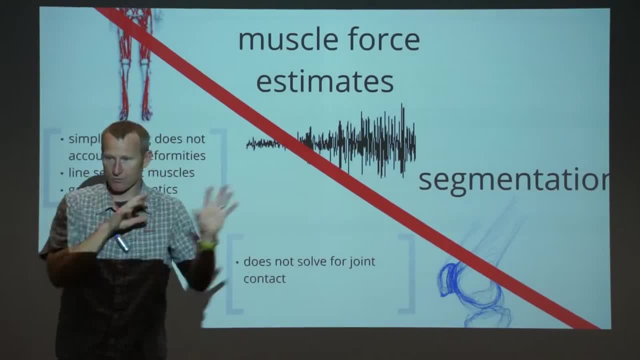 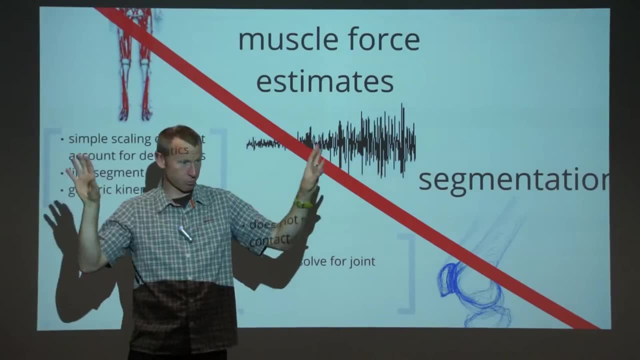 We solve this in one domain over here. Here we take these forces and results and we put them into another domain over here. So you might have joint contact and continual mechanics here and rigid body dynamics there. But this is a problem. If we can join the two together, we're more likely to get better estimates of muscle forces. 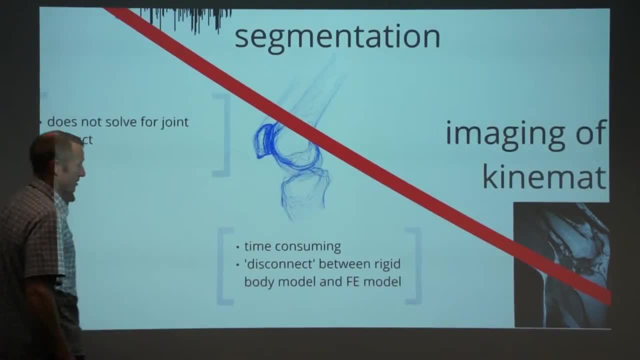 So that's something that we need to address. Segmentation is always an issue. This is time consuming and it's retarded. We don't need to all be segmenting the same bones over and over again, And you'd be surprised. I mean, this is usually the first six months of a patient. 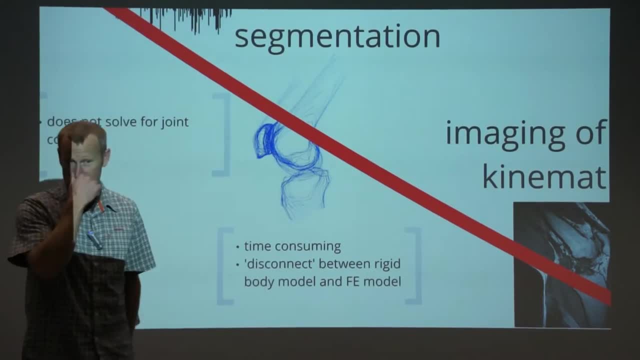 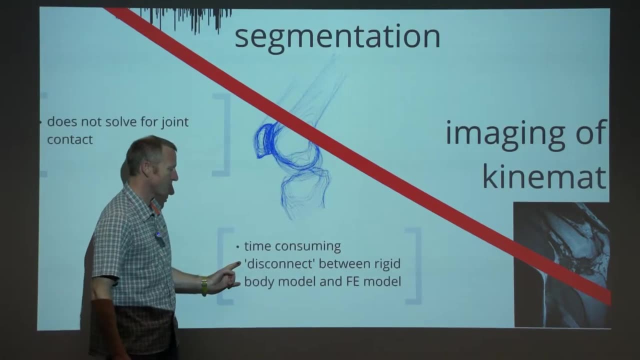 This is the first six months of a PhD's life here at the ABI. Okay, Here's some medical imaging data. Go ahead and segment. Okay, There's smarter ways of getting around that and I'll talk about those in a minute. And here's the issue I just mentioned before. 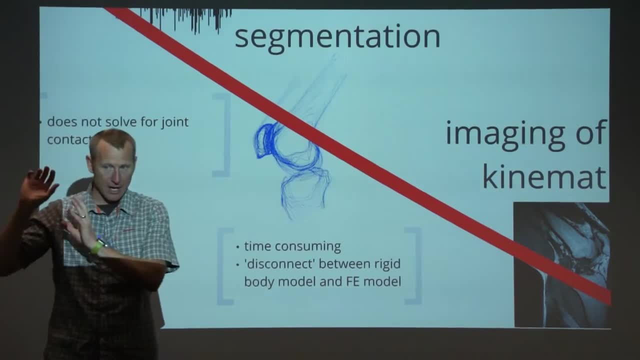 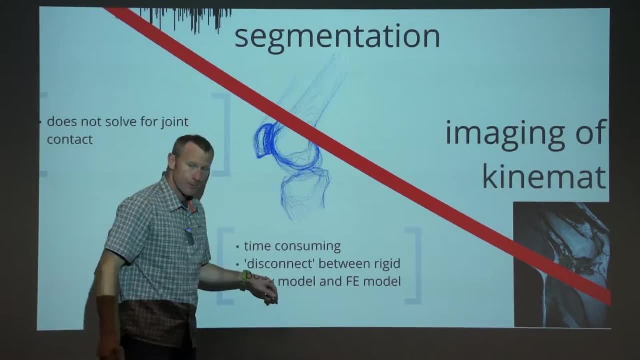 There's a disconnect between the two domains: the rigid body dynamics and the finite element model. The finite element model is typically from segmented imaging data, whereas our rigid body dynamic model comes from our simple scaling back up here. Here's our rigid body dynamic. 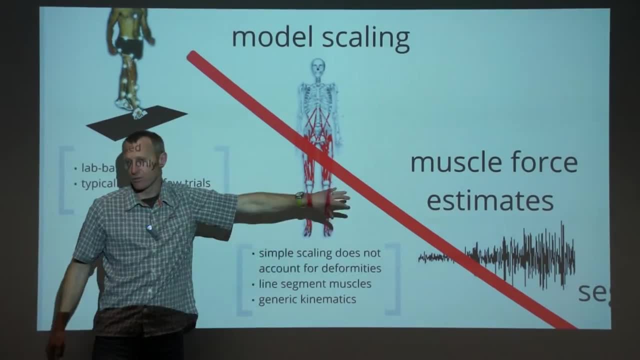 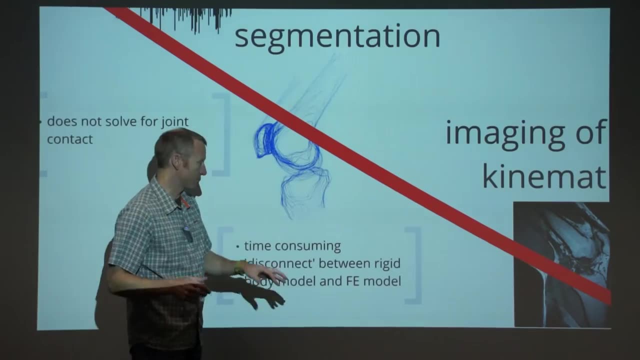 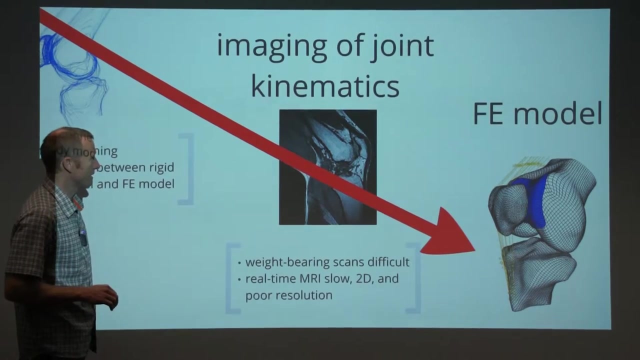 So we've done some linear scaling and this does not match your medical imaging data. So we're already. our geometry is not even consistent right between the two domains, So that's a problem. If I'd known about all these problems, I would never have accepted half of my publications. 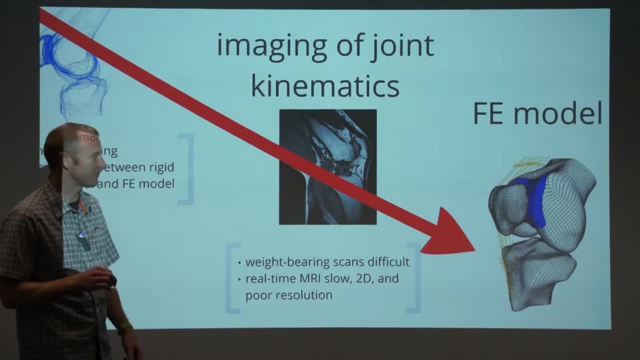 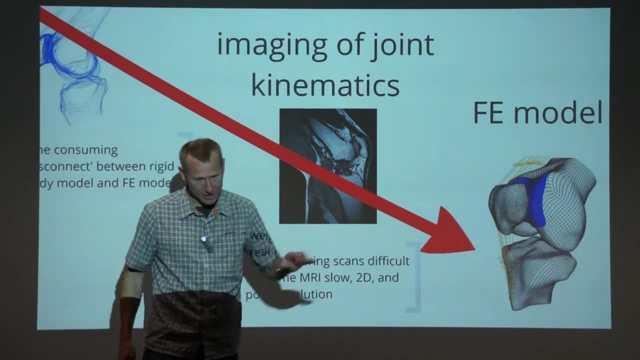 that I've got so far, But anyway, thankfully somebody else reviewed them and not myself. Imaging of joints, Imaging of joints. So, imaging of joints. Imaging of joints, Imaging of joints. This is basically done in a static position: You're lying down in a scanner. 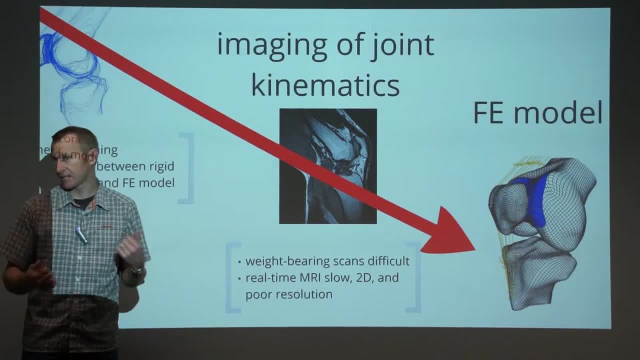 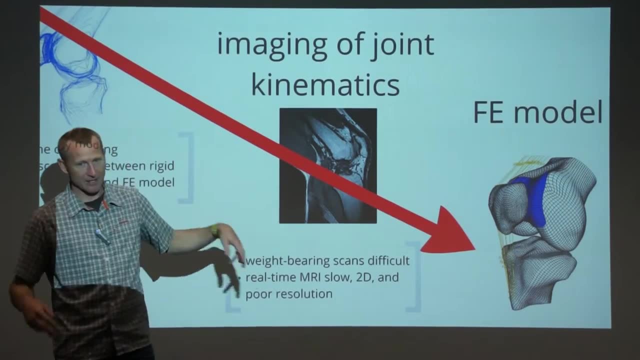 That might be an MR scanner, it might be CT. Ultrasound is kind of nice because you can get some dynamics, But ultimately a lot of these imaging modalities are done in non functional postures. Okay, They're static, They're non-weight bearing. 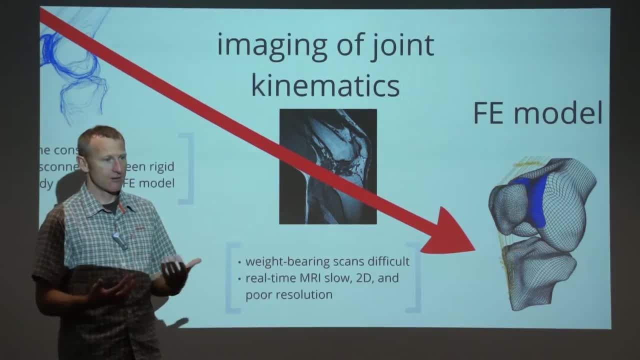 So this is an issue because if we want to characterise the deformations of tissues and other things in a dynamic sense, or the dynamic movement of a tissue, And so if we want to characterize the deformations of tissues and other things in a dynamic sense, 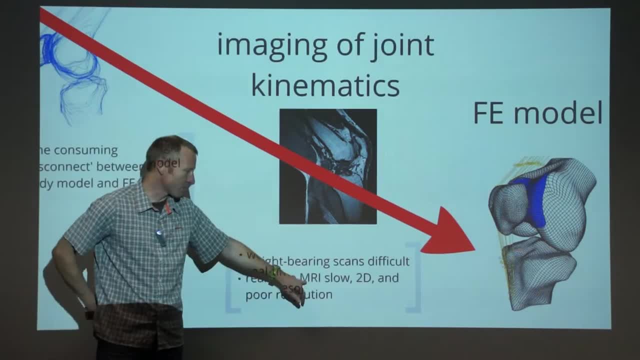 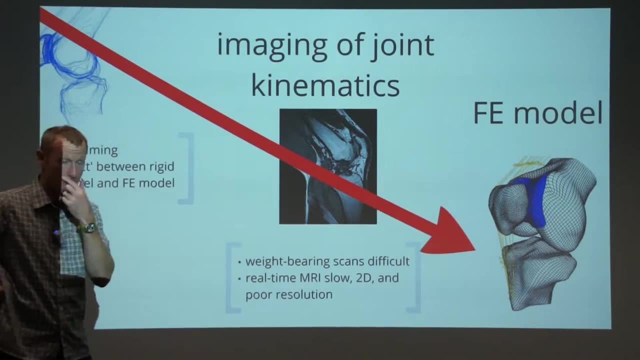 of a joint. this will not do. We've done some work in real-time MR. before I came back to New Zealand five years ago, we were doing real-time MR in an open magnet, so this, the MR, actually kind of looked like two halves of a donut you. 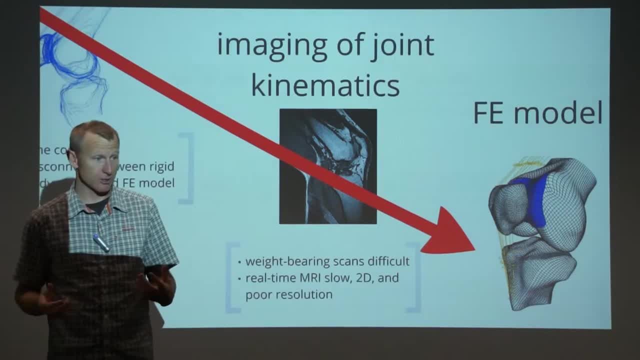 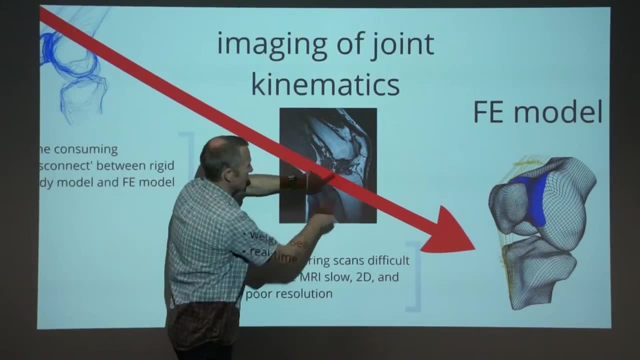 could stand inside and do weight-bearing squats, which was pretty cool, and this is one of those images. this is my knee joint, actually in a weight-bearing loaded posture. you can see, these are my ligaments, my cruciate ligaments, which thankfully, I have them still intact. here is your patella, your kneecap, and 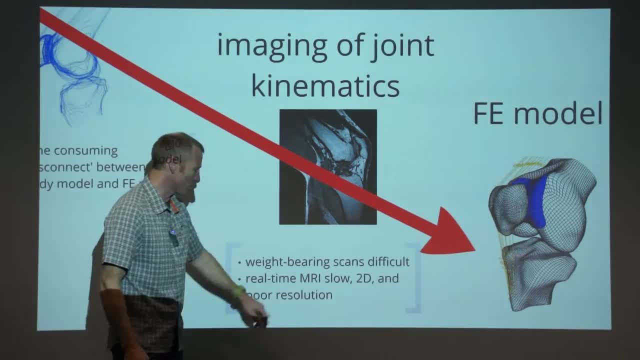 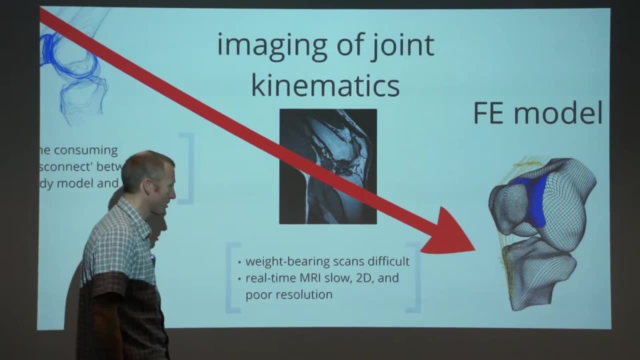 this is cartilage just here, so we were looking at using real-time. the problem is, this is really slow. this is about three to four frames per second, so you can only go very slowly and it's only giving you a single slice. the resolution wasn't great. you know there's limitations there that we need to. 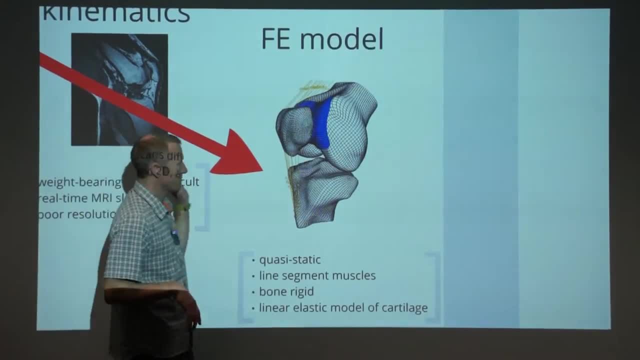 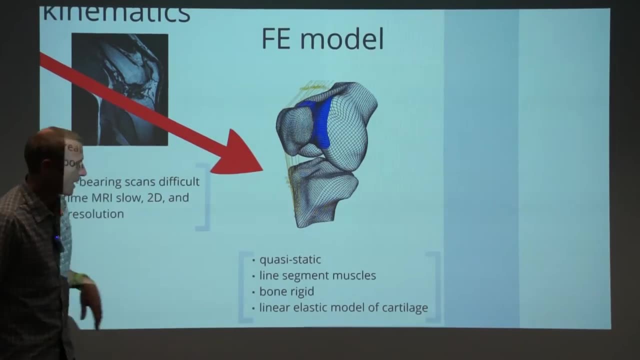 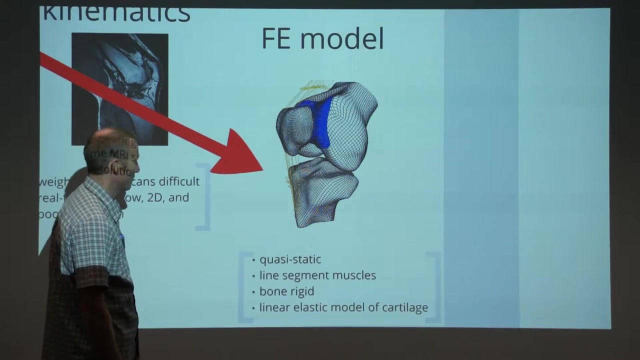 address. and finally then, when we get to our FE domain, this is just a model, the, that I was using to look at patellofemoral contact, And there's a whole bunch of issues with this model, And you could again tear it apart and critique it. 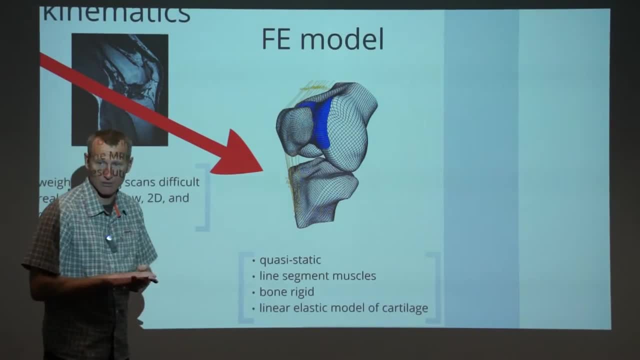 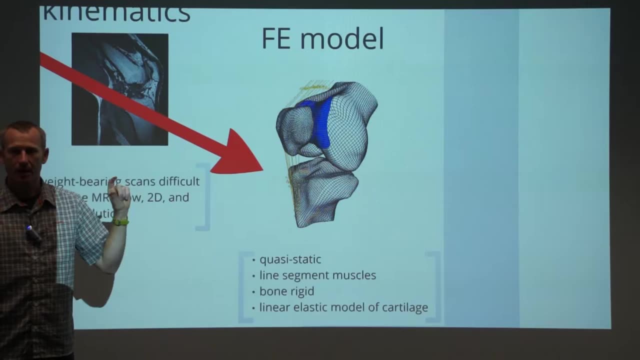 But for its purpose at the time it was suitable for answering the research questions that I had. That's the key thing when you develop your model is be clear about your research questions and make sure your model is adapted to answering those research questions and within those research questions. 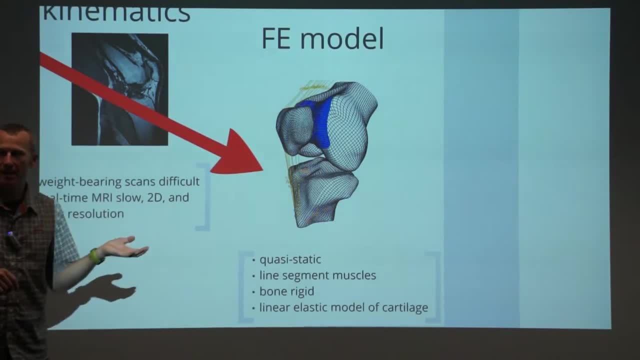 Because there's always more you can add to a model. There's always limitations of a model. Just know what they are and be clear about it, especially when you're presenting your work. Anyway, our models here, they were quasi-static, They weren't dynamic. 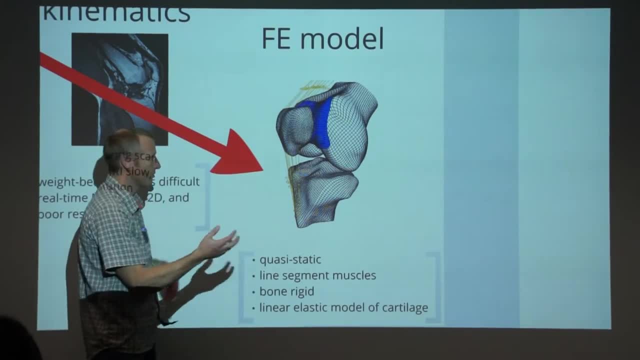 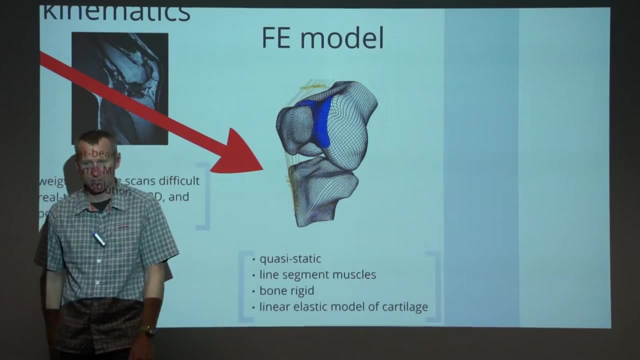 They involved again line segment of muscles. The bones were rigid so we weren't looking at deformations, stress, strain in the bone tissue And we had some simplifications of our material properties of cartilage. We know cartilage under dynamic 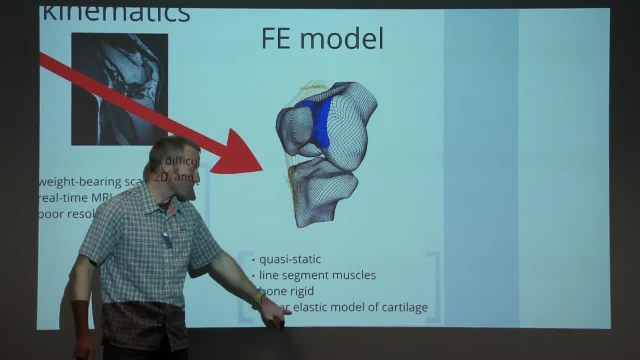 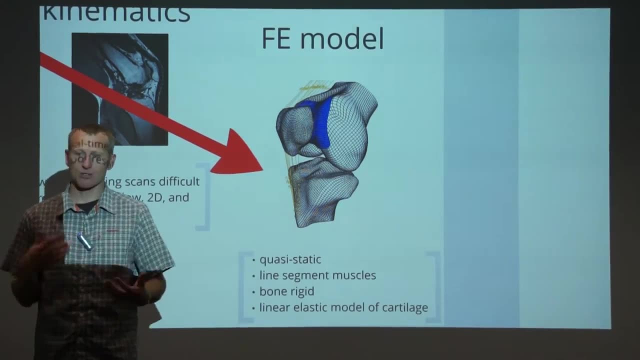 Activity, dynamic load. it behaves pretty close to a linear elastic solid. So you can make this gross assumption if you're interested just in kind of gait or dynamic type behaviors, If you're interested in how fluid flows through the tissue, this is obviously not going to work for you. 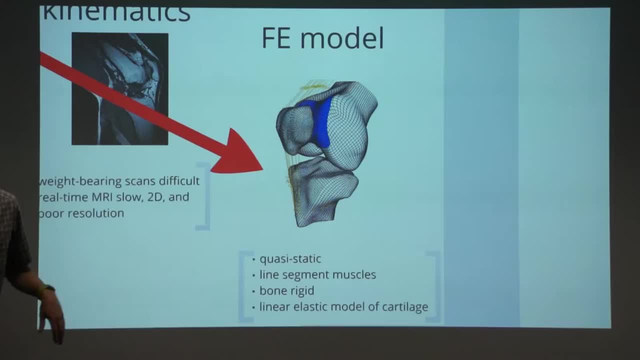 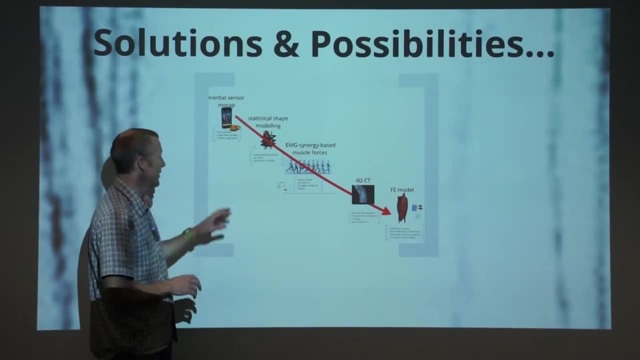 You need to do something a little bit more sophisticated. But anyway, those are some limitations of our current approach. Now, of course, I'm not going to leave you with limitations. I'm going to leave you with solutions and possibilities. And here is then. 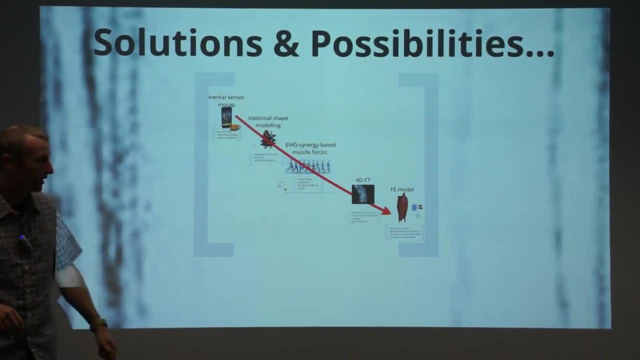 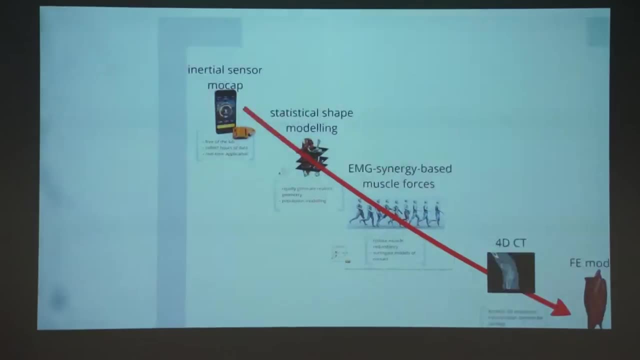 Here is, then, some of the work that we're doing to address these challenges, And it's the same workflow. This time we've got some different tools, So one of the things we're really quite keen on is to measure people outside the lab. 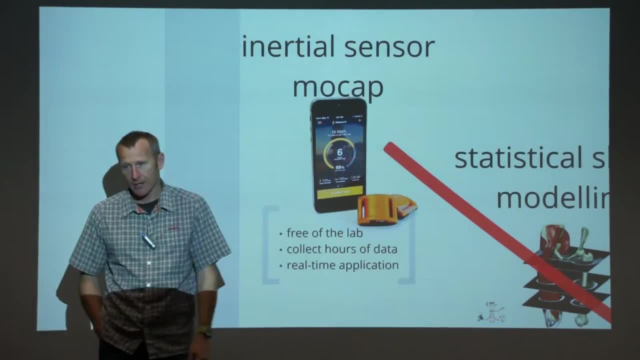 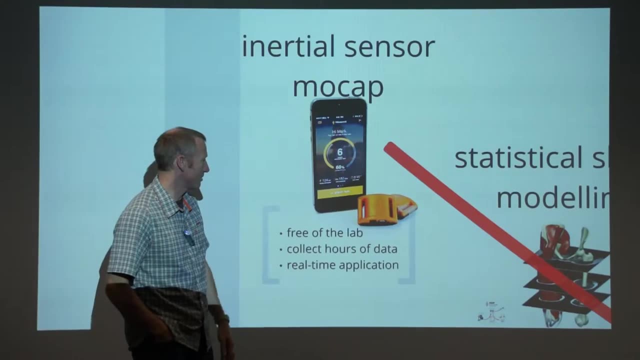 And one approach is wearables. Wearable sensors are now everywhere. They're ubiquitous Inertial sensors. this is just one from a startup company that I just happen to be involved in and I declare conflict. I said conflict of interest. 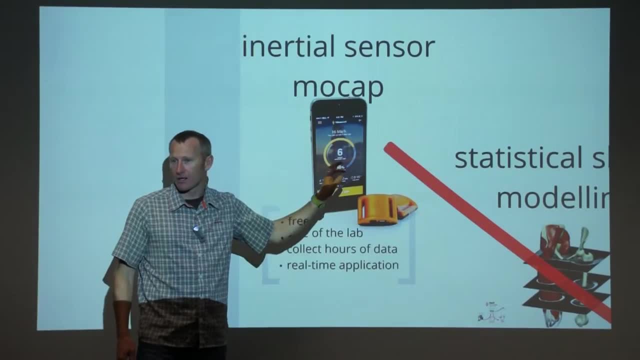 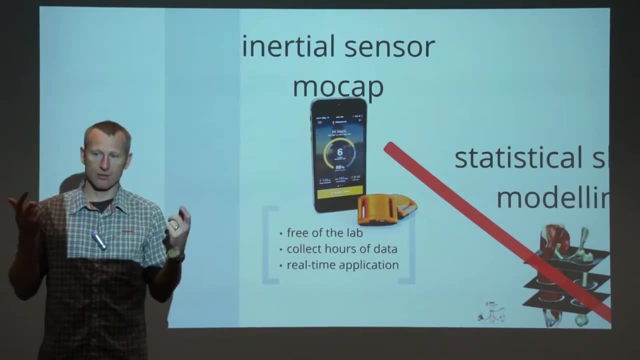 But these are ubiquitous. They're in everybody's cell phones nowadays, inertial sensors. But can we then create a model that predicts the movement? that is then matched to the experimental data you get from these inertial sensors, So you're matching linear accelerations. 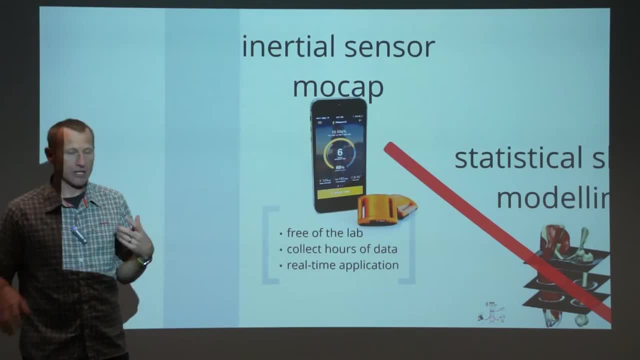 from the accelerometer and angular velocities from a gyroscope. And yes, we should be able to do this, We should be able to construct a model that, on the one hand, this is a more structured model, on the other hand, 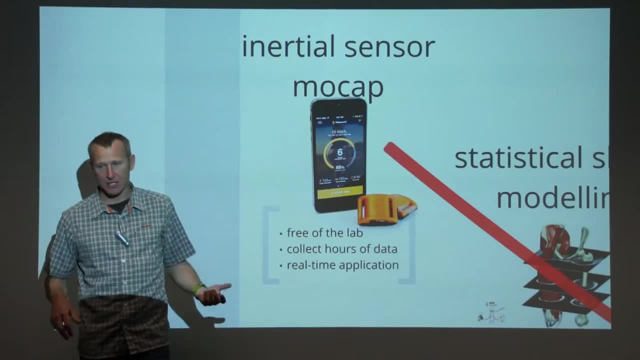 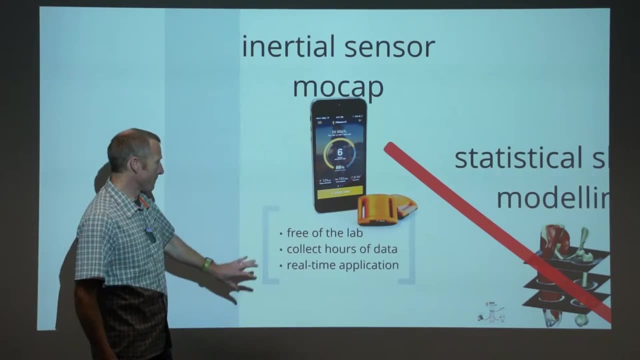 that has the certain degrees of freedom we want, with enough sensors that we can reconstruct motion- And we're not the first people to do this, there's other groups in the world that are leading the charge on this- but it would enable us to get outside the lab to put sensors on. 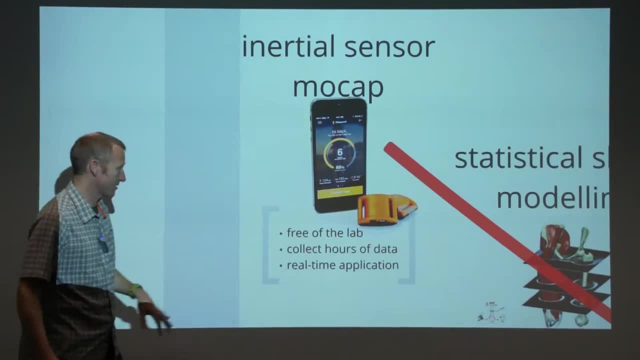 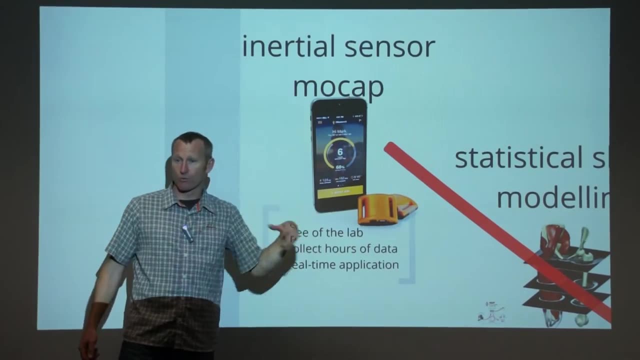 our patients and characterise their movements in real world settings, And I think that's very important. and it also opens the door because you can start connecting these guys with these guys for real time feedback, And I'll talk about some of the real time feedback we're doing. 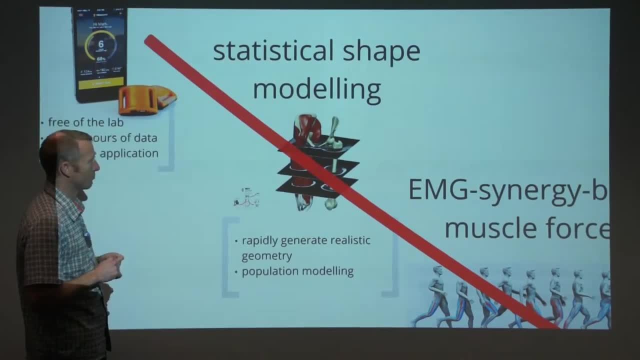 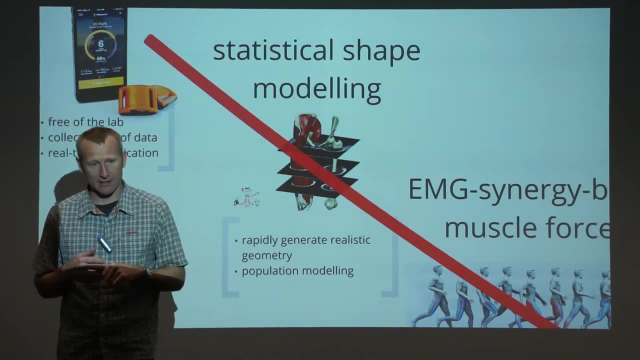 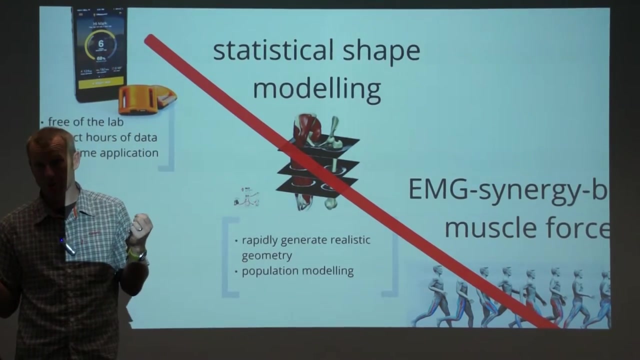 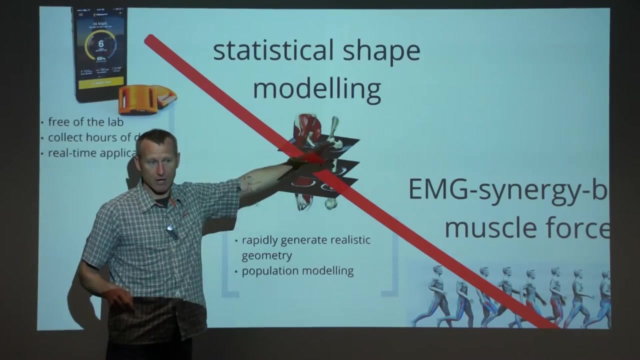 Statistical shape. modelling has, and will be, an important aspect of our workflow in years to come, And so this idea is that if you have enough data and you can perform some statistical analysis on this data, you can characterise the variability of that data. Now, whether that data is time series data or, in this case, it might be nodes on a mesh. 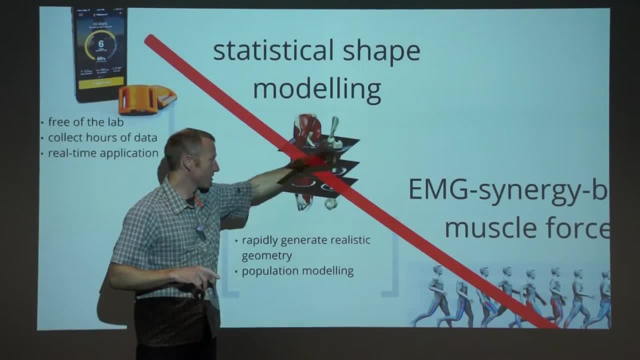 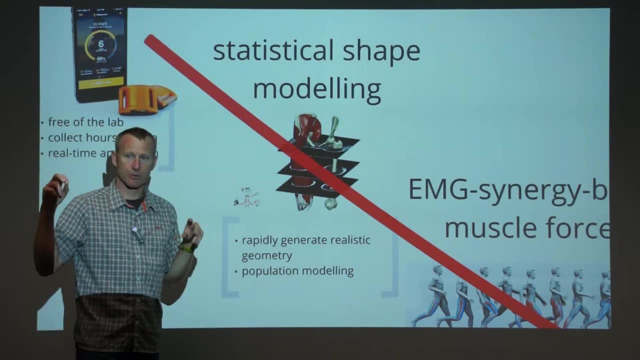 the variability And shape right the x, y, z coordinates of these nodes, you can perform some data reduction methods and very efficiently characterise the variation in geometry. And this is really nice because then you can do some interesting population type modelling. 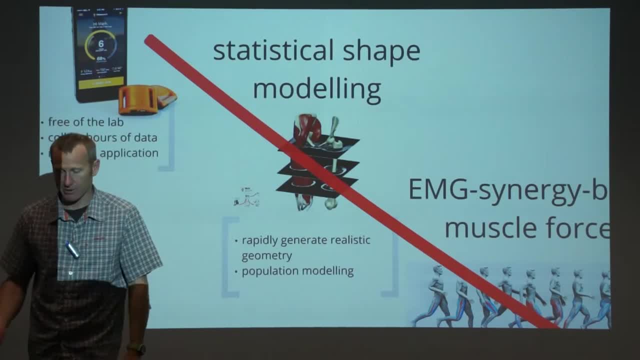 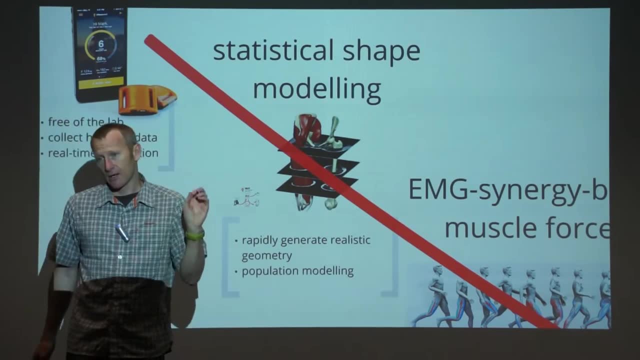 If your data set. for example, we use a data set from Melbourne, from the Victorian Institute of Forensic Medicine, and they do post-mortem CT- whole body CT- So we get access to those data, we segment them out and we make models that can characterise. 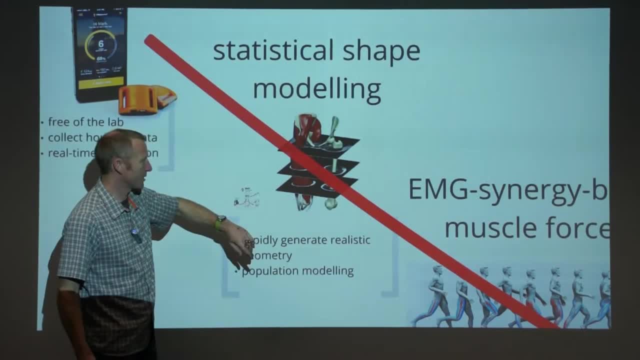 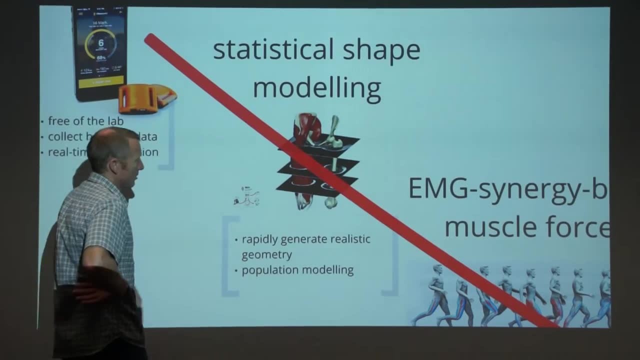 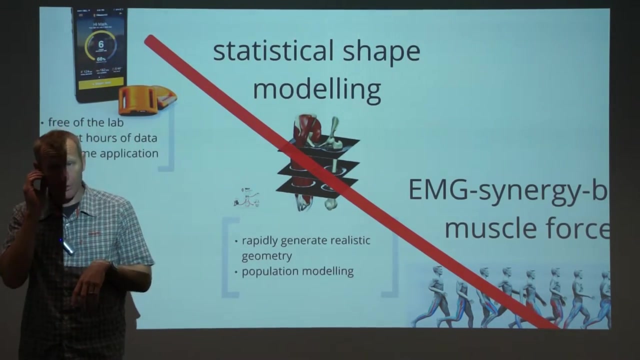 the femur, for example. This was Zhu Zhang's PhD thesis. He did that with Paul Nielsen here at the Institute And the idea is that you could accurately characterise all of the different shape variations of the femur with very few modes of variation. 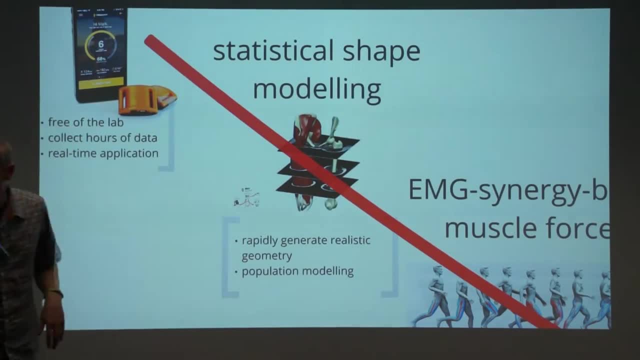 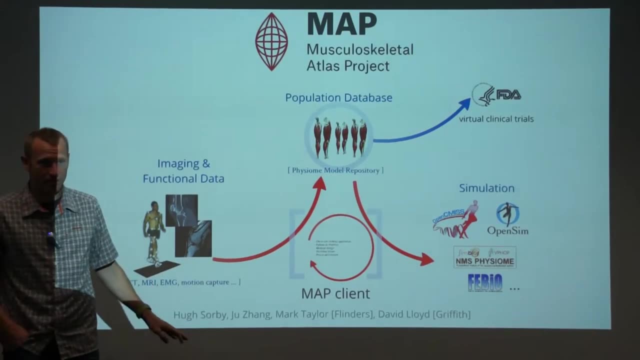 So this was from a principal component analysis looking at the different modes of shape. So, using this idea, what we've done is, with help of some of the software team who are sitting in the room right now, generated or created a workflow manager- And you guys know already, you've heard about this right- the MAP client. 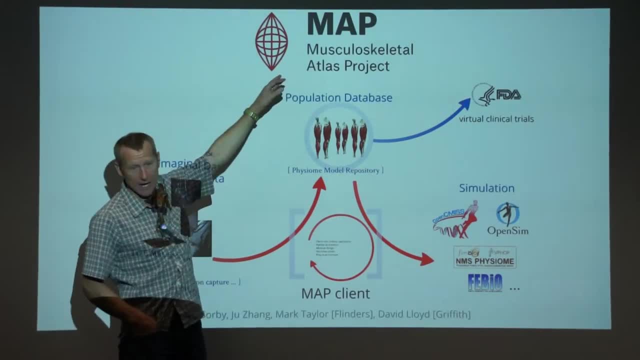 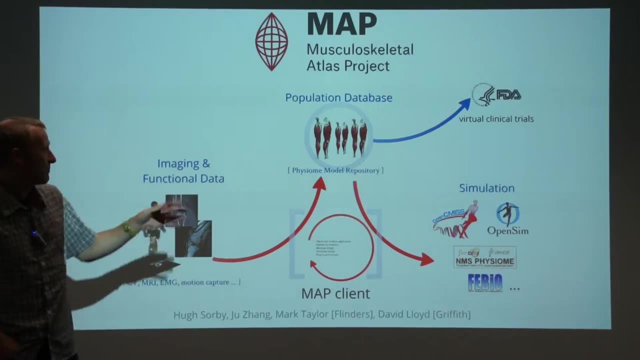 And it came from this concept. I actually stole the acronym MAP. I stole it from Alistair Young, who previously had CAP, which was the Cardiac Atlas Project. but MAP is a much better acronym because it has so many other meanings and connotations, right, so it's much cleverer. 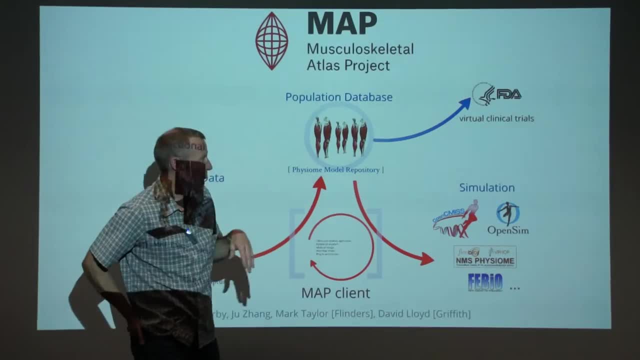 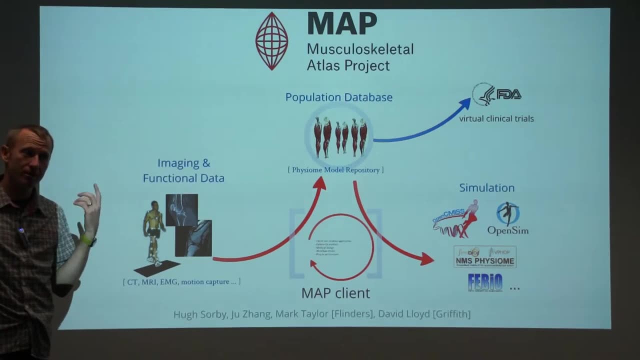 I thought Anyway. So I stole the acronym, called it the Musculoskeletal Atlas Project, and I got some funding from the FDA to do this. Now, why on earth would the FDA give us money to develop this? Well, they're interested in silico virtual trials of medical devices. 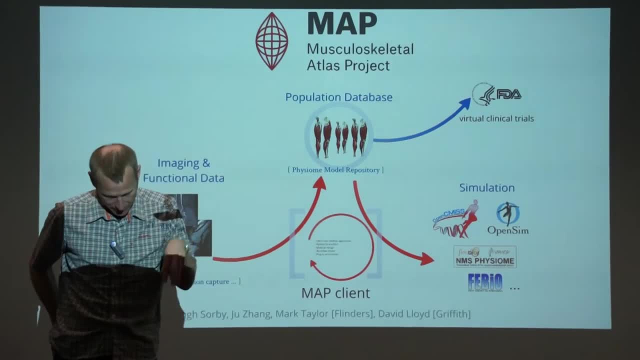 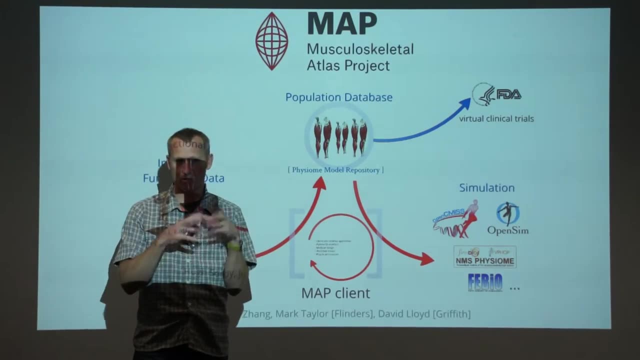 So if you have a new orthopaedic implant and that implant is for a hip joint and it needs to go down the stem of a femur, well, wouldn't it be nice if you had this population model of the femur that characterises all of the geometry of not only the outer cortex, 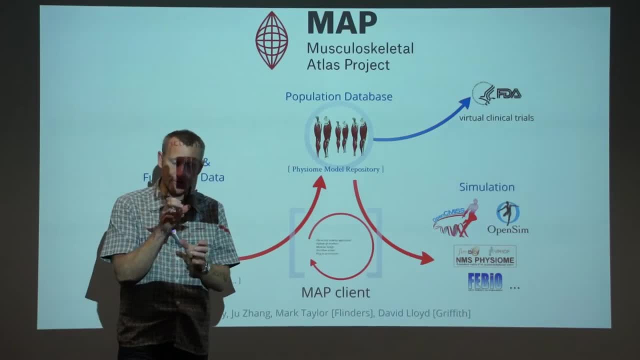 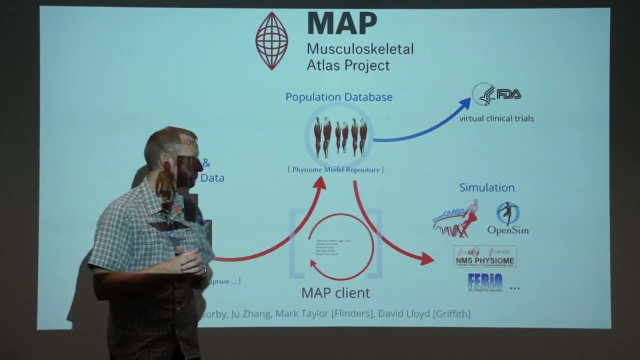 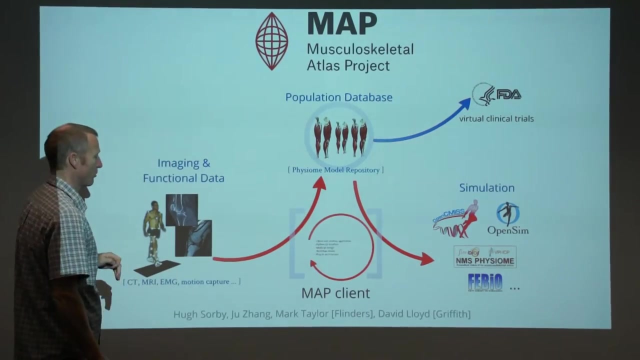 the outside geometry of the femur, But also the inner cortex, because then you could accurately characterise how well this new device fits in this population of 300 individuals. That would be very useful. So anyway, we got some funding from them and we put together this concept where we would 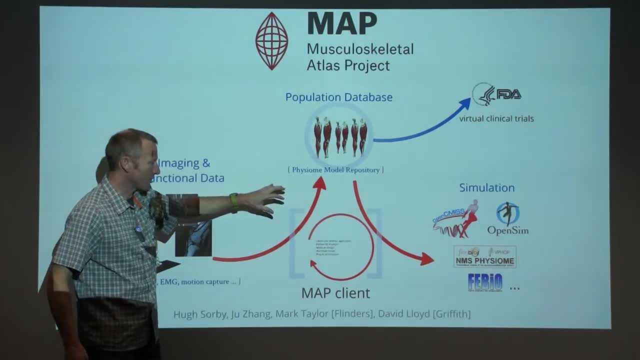 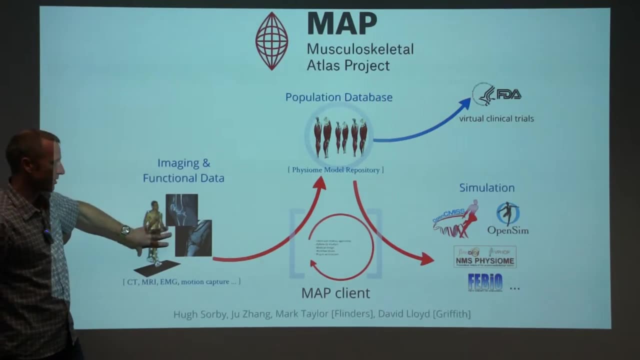 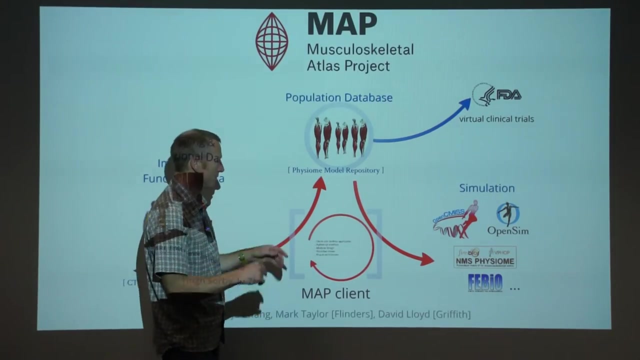 have some sort of client application and the client could receive information of medical imaging data, motion capture, EMG, any functional data you might have. you can use the client then, So you bring this data in. you can create workflows within here to do some modelling. 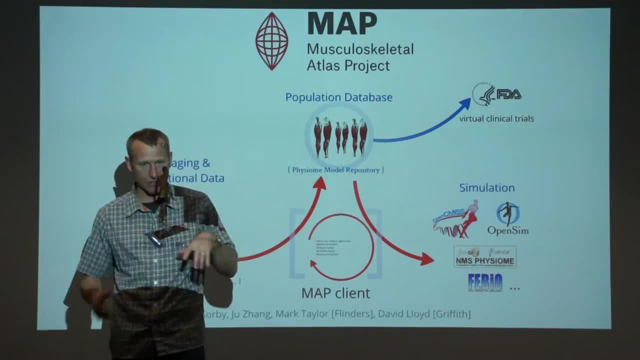 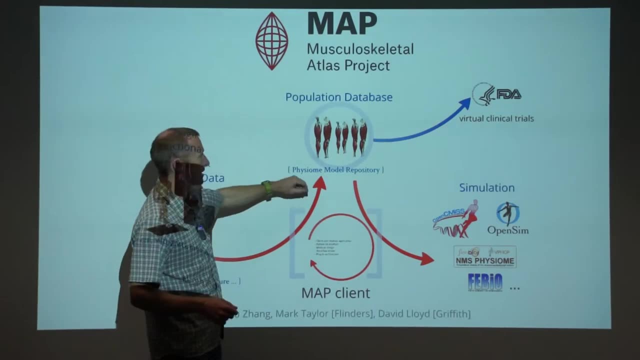 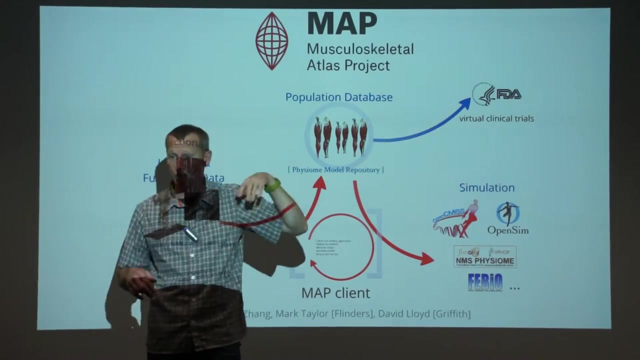 you could also link the data to a repository, and the repository would have this super set of information that's being collected from people all around the world- data models and other things that could eventually be linked to FDA for regulatory approval. it could also be linked to journals to test out your ideas and for review purposes. 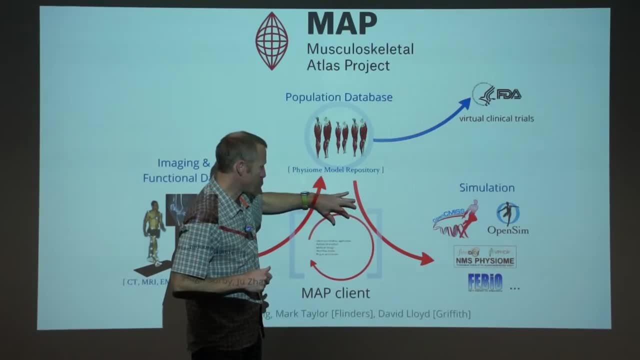 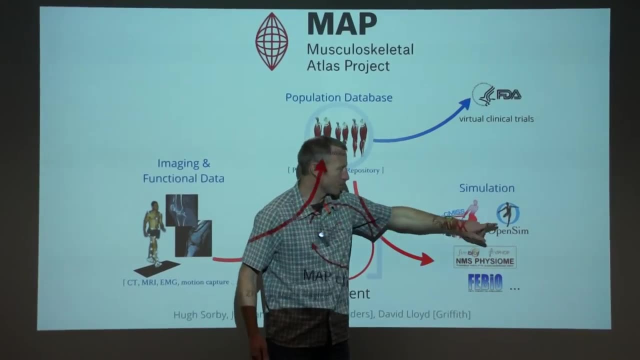 So it kind of has lots of functions, And ultimately you could spit out a model from this client as well, and that model might be useful for OpenCMIS, it might be useful for OpenSim, which is our rigid body dynamics, and there's a couple of other packages that we're kind of linking to as well. 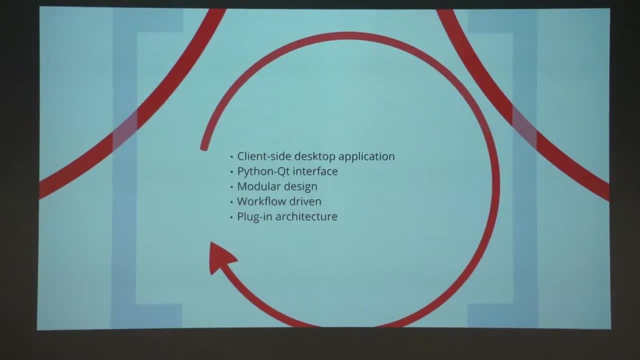 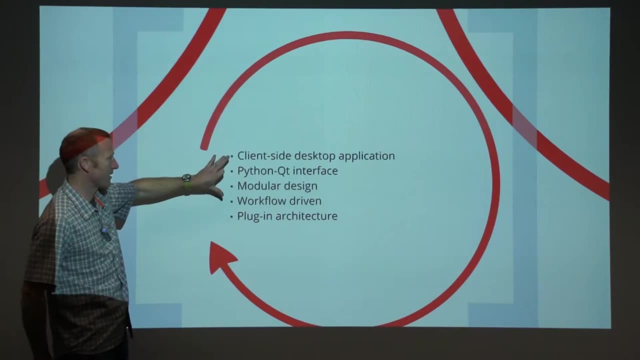 And so this was the concept. just briefly, because you guys will probably know more about the MAP client than I will by the end of this, But this was our criteria. We wanted to have a client-side application designed in a way that was accessible to the. 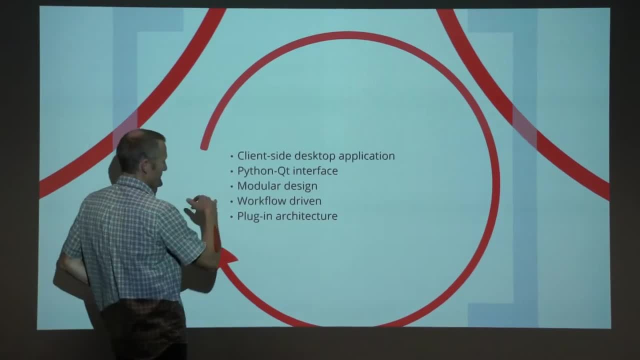 client And easy to use and common language. and Python, of course, was the language of choice here, because it's free, open source and it's the language of choice for a lot of science and it's growing in popularity. 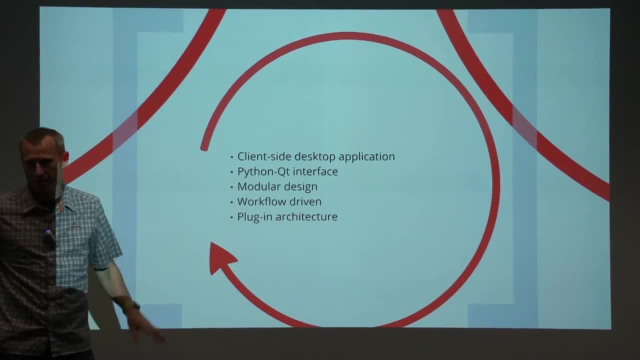 We wanted to have modular designs. It's workflow-driven because, again, regardless of whether it's the heart or the lungs or whatever musculoskeletal system, you're kind of doing the same thing, right, You're doing the same workflows. 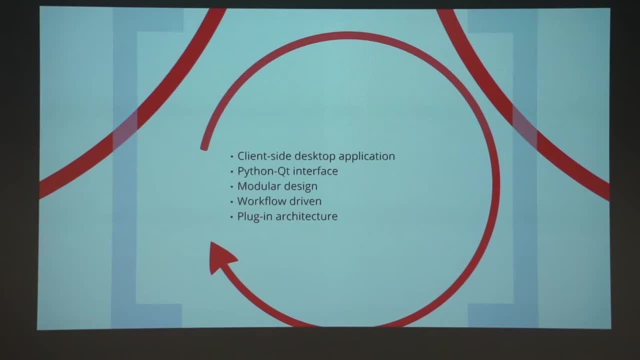 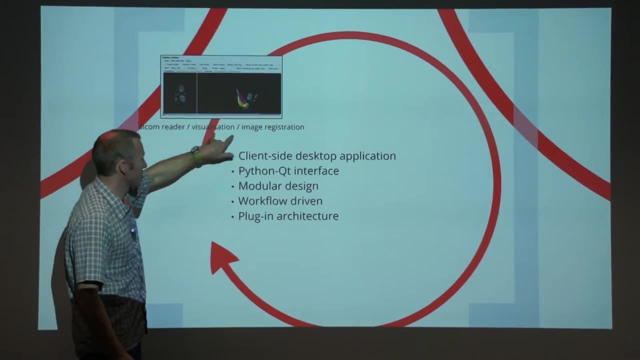 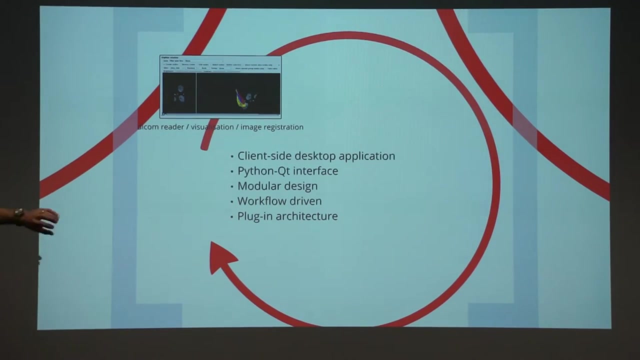 And the idea too is we have this plugin architecture So embedded in this idea was that you could read some DICOM files, so standard imaging, You could do some visualization, You could do some standard segmentation and registration. These are just basic set of plugins. essentially that would create workflows. 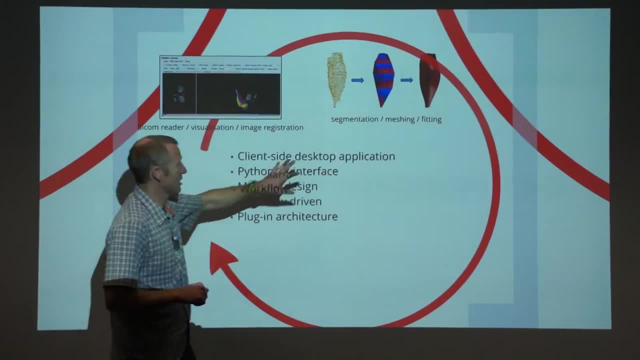 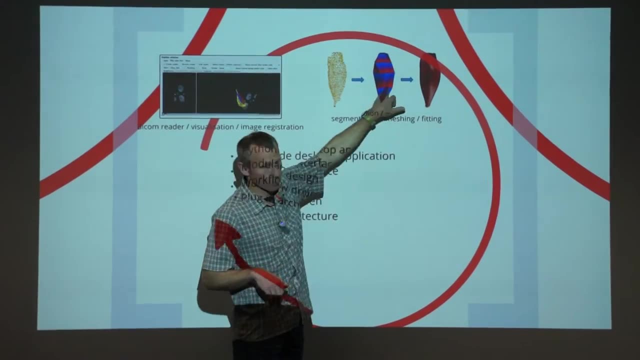 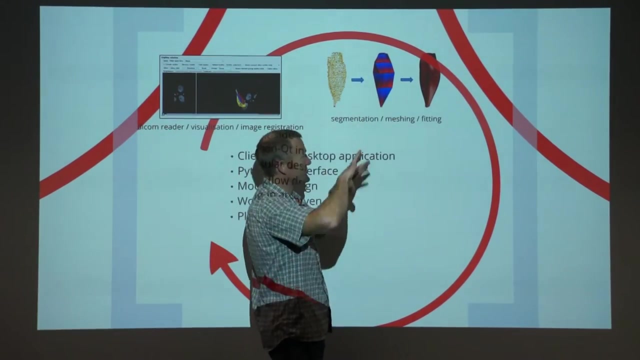 And we call the plugins steps, of course, The segmentation to mesh fitting. you know, this has really come from the ABI: the idea that you would have these higher-order elements that capture cubic variability between nodes instead of just linear variability. So you need far fewer elements to capture the geometry of the tissue. 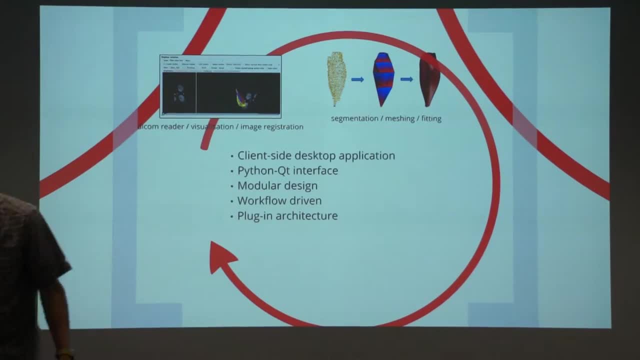 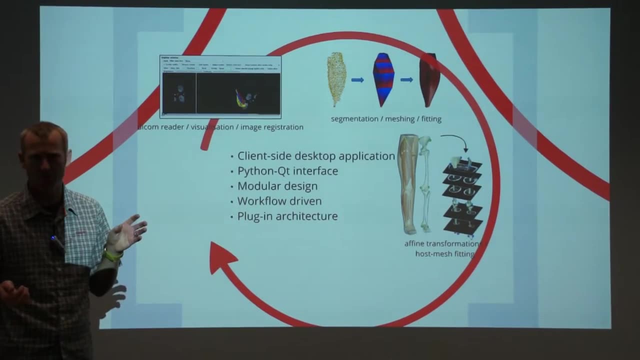 And so we threw those tools in there as well. We said, well, we want to be able to do some host mesh fitting. I don't know if you guys dealt with or talked about that at all. I don't know if you will get to that. 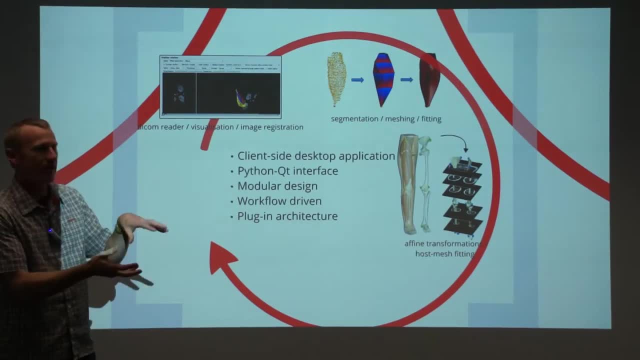 The idea that you start off with a template mesh and you can embed that template in a host And that might be just a cube, and you deform the cube such that your mesh that fits within that now suddenly fits your new data set And you can apply these kind of methods as well for doing non-linear scaling. 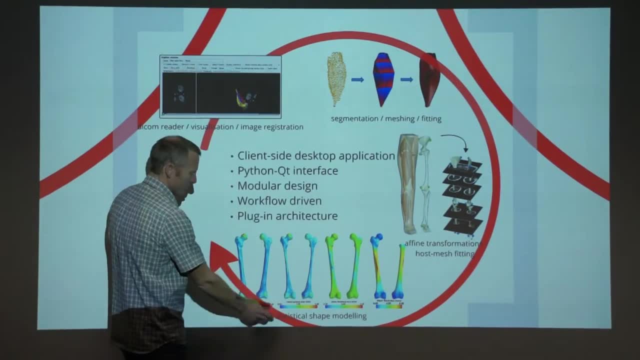 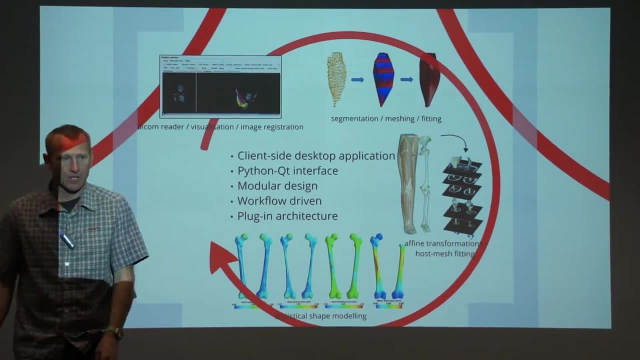 And really at the heart of all of this, too, was this idea that you could drive your segmentation fitting model generation with underlying shape models, And so, again, this was the work of Ju Zhang from his PhD, And he stayed on. He's been a postdoc for the last couple of years now. 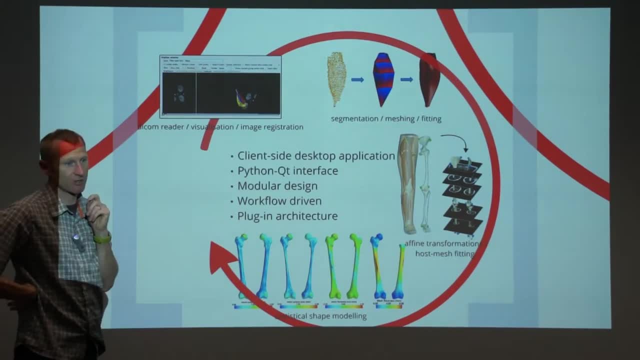 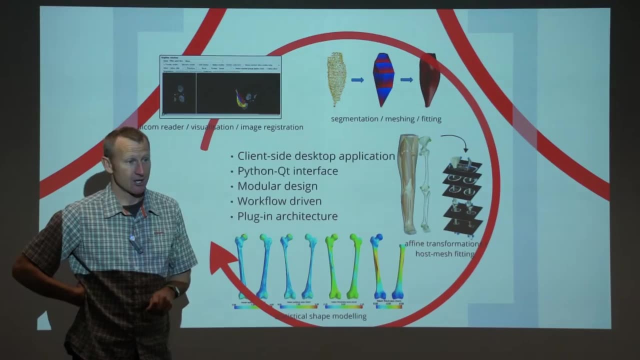 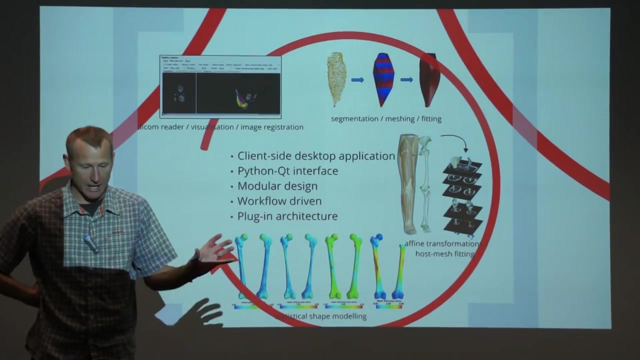 And unfortunately he's leaving us in September. but he's not going far because he's starting his own company that's going to be using shape models to design orthopedic implants, And we're working with OSIS, who are in Christchurch, and helping them with a workflow that automatically 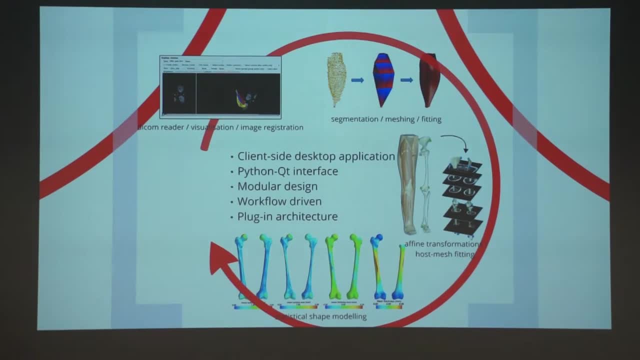 generates implants for revision hip joint surgery. But anyway, Ju's kind of been the main driver of putting all of these plug-ins together, Yeah, And ultimately we'd also want the client to run your simulations. So you make your model, You can spit it out to OpenCMIS and call it back. 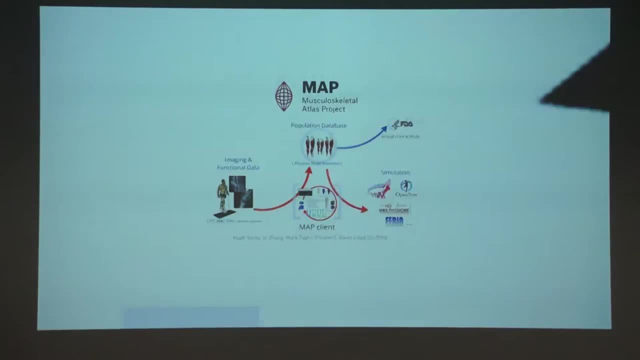 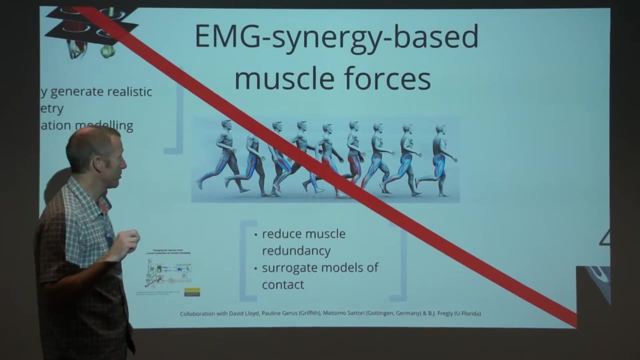 That's kind of the ultimate goal, Anyway. so that's the overview of how to address that problem. Pablo is quite familiar with this stuff, But for the rest of you, there's an idea here that the way that muscles are activated muscle 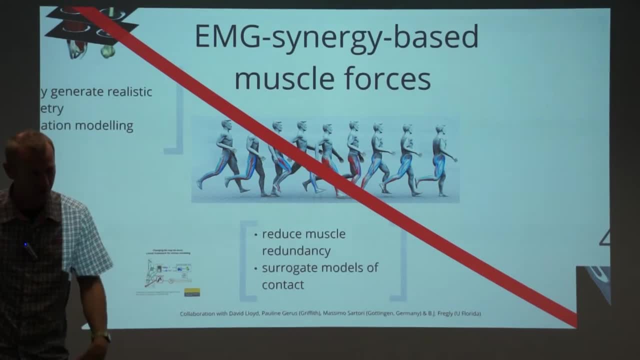 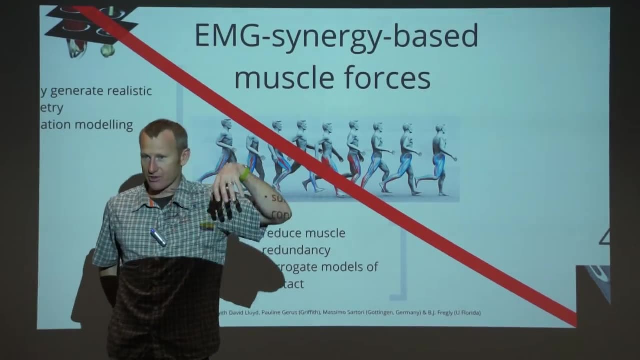 forces are critical. Yeah, And that's what we're looking for in determining what the loads are on the musculoskeletal system. And muscles are activated, of course, by virtue of the central nervous system. Everyone has brain, or most of us have a brain. 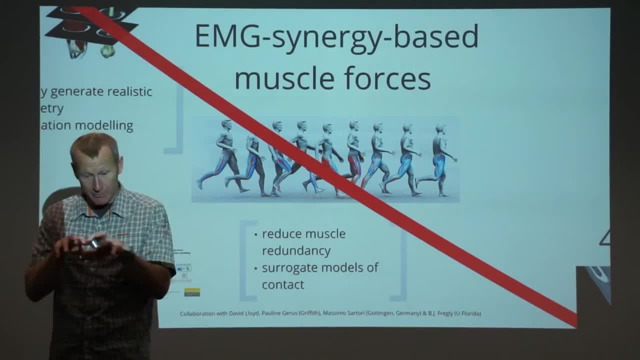 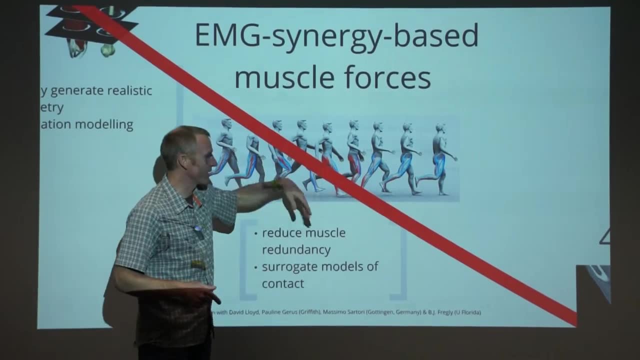 And it's connected to a spinal cord And there's a cerebellum that's connected there. that's driving lots of different activation patterns of our muscles that cause us to move And these are modulated at different levels. It can be modulated at very high levels or it could be modulated at spinal cord level. 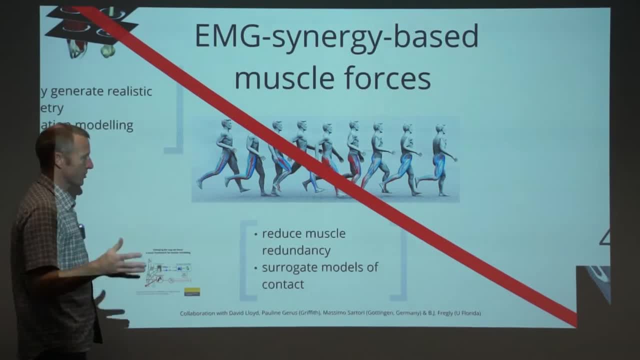 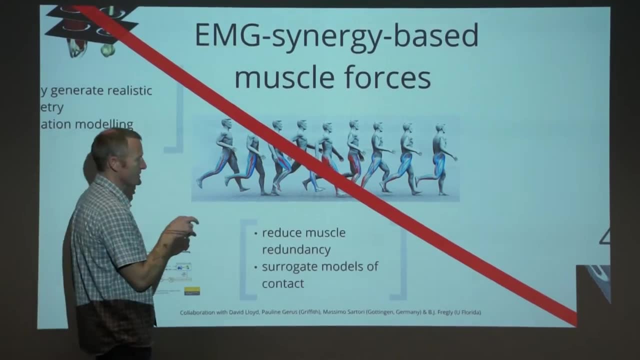 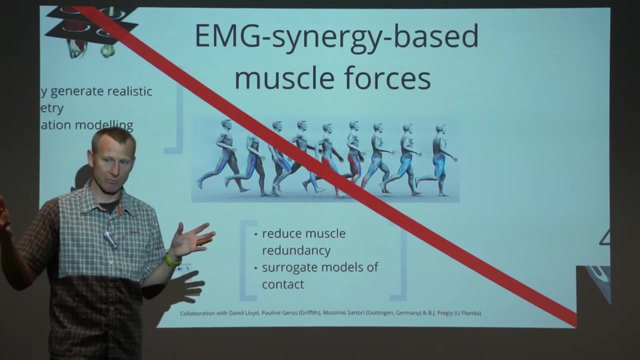 You know low-level modulation as well. But what the neuroscience literature have been doing quietly over the last decade is developing models of this to show that you can, in the same way that you can characterize the variability and shape of a bone, you can characterize the variability and the synergies. 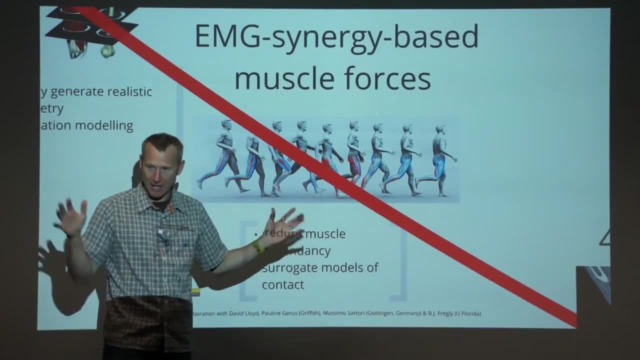 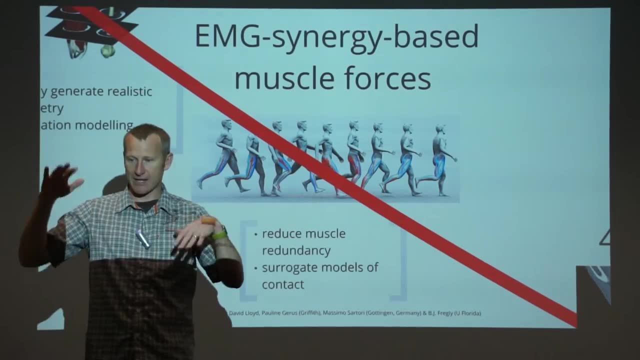 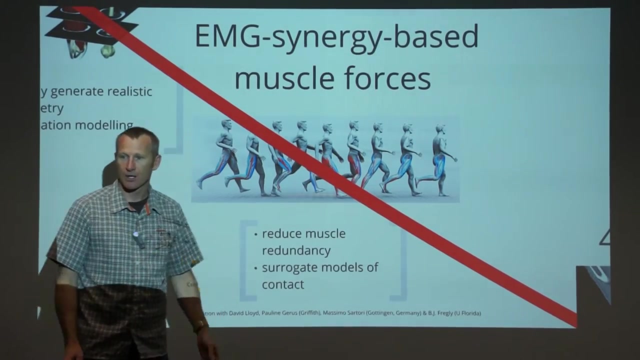 the way that muscles are activated together and do some mathematical data reduction And it turns out that you can get, say, five principal models. Yeah, Five principal modes that can modulate the activation patterns that correspond to 95% of the EMG that you see in your low limb muscles during walking. 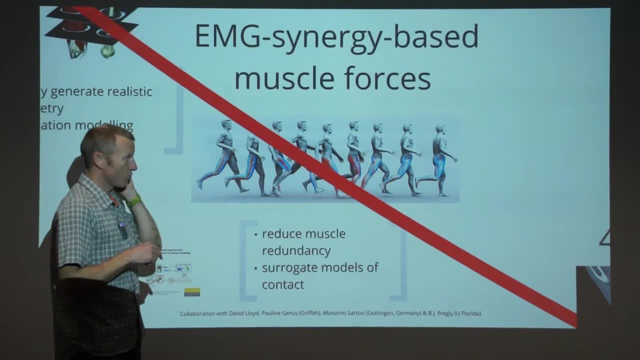 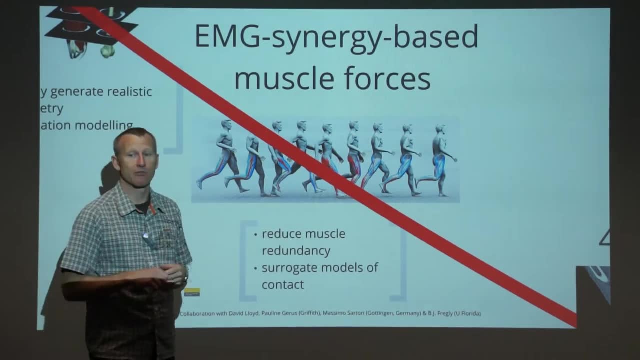 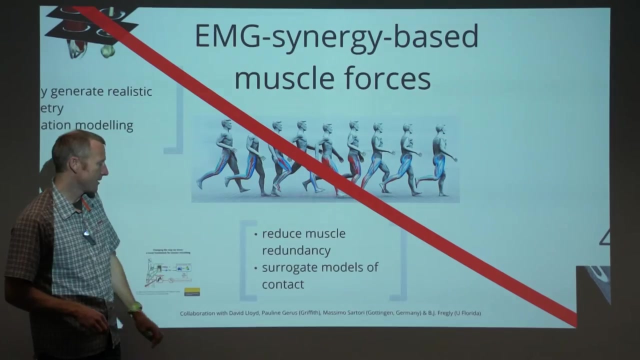 So this is pretty interesting because now we can say: well, OK, perhaps we can get a better representation of all of these muscle activations by only measuring a subset, a few number of key muscles, and using this idea of synergies. So this is a way of reducing the redundancy of muscle activations. 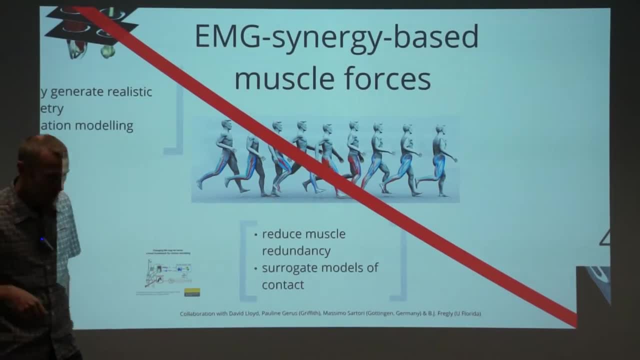 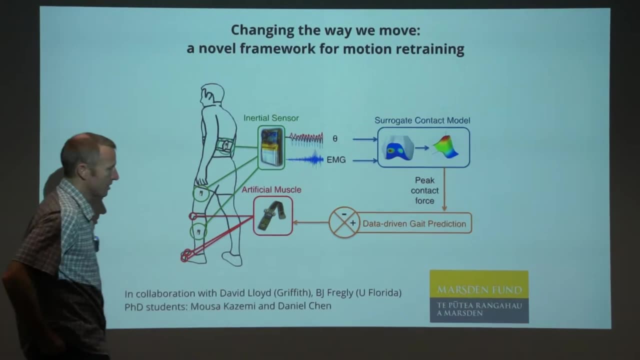 The other thing that we're working on is surrogate models, Surrogate models of contact. So that's crossing the domain between the kinematics and joint contact. So this is a project that was funded from Marsden. It's now reaching an end. 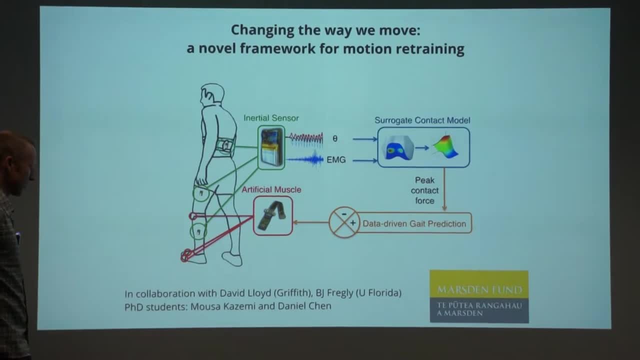 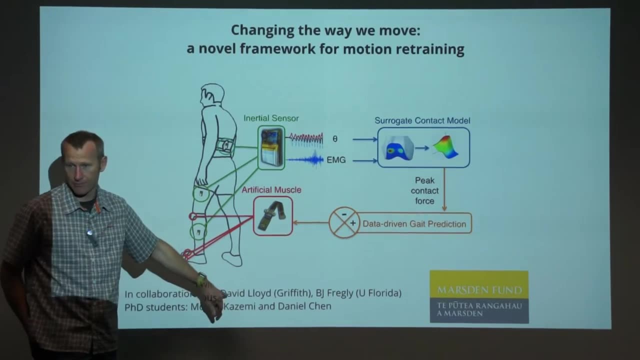 And in the next four months or so we've got left And I've had a couple of PhD students working on this. I've been collaborating with David who's at Griffith. He was my PhD advisor years ago, back in the late 90s, and working again with my colleague 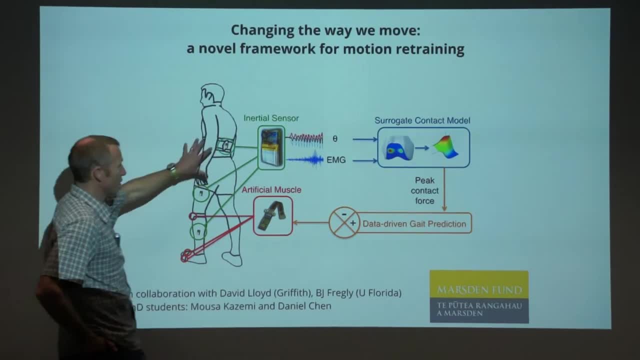 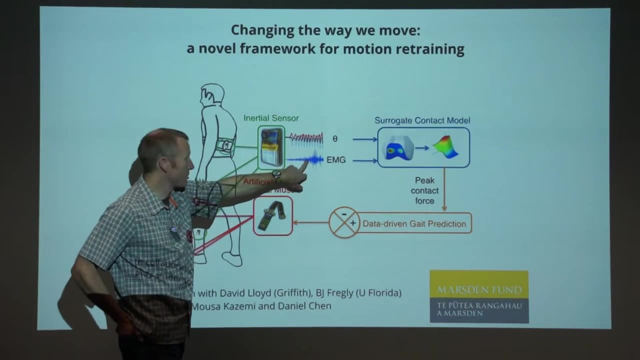 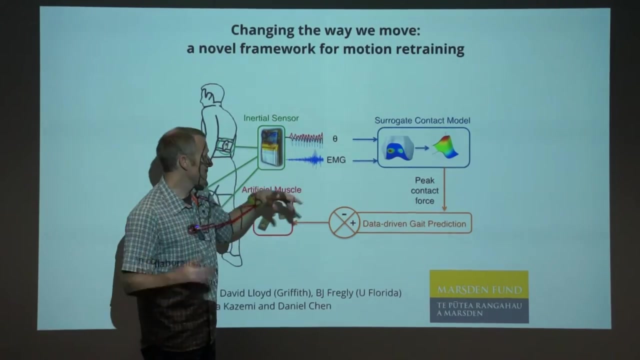 from the University of Florida. The idea here is we've got wearable sensors, inertial sensors, strategically placed on the limbs. These can also measure muscle activity by EMG electromyography. So we can get these kind of measurements of the joint angles, the joint movements as 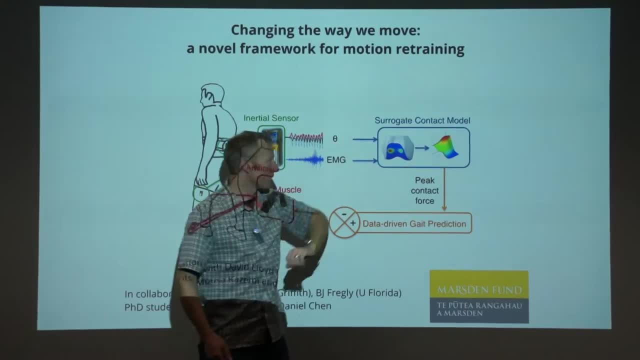 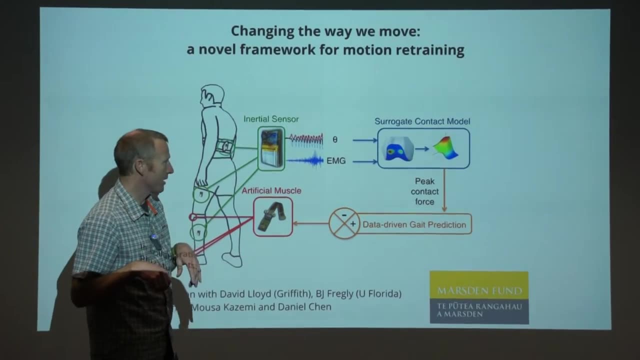 well as the muscle activity, And we develop a surrogate model of joint contact. So we've got a finite element model. That finite element model has all the muscles that we care about, And what you can do is you can probe this model offline. 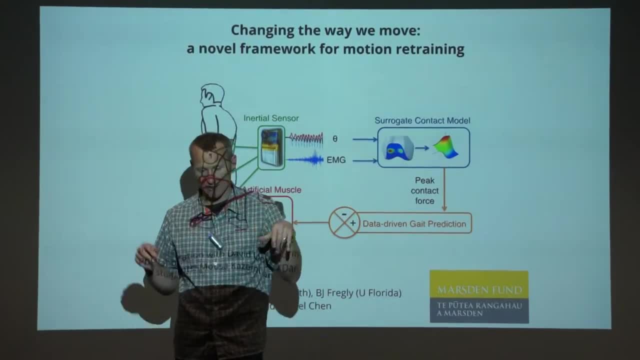 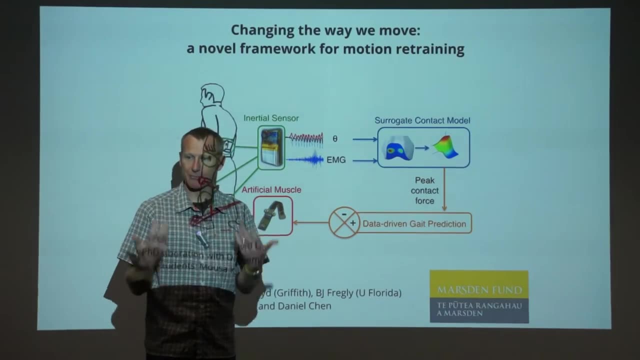 You build this model offline. You basically say: here's a combination of synergies that I would get during walking, all these possible combinations. Now give me as an output what the stress distribution is of this tissue, And what you do then is you build up this internal model. 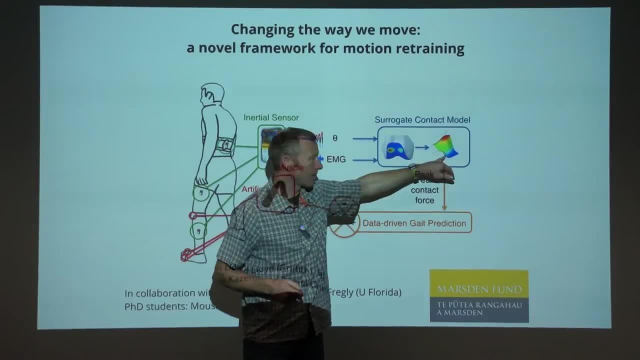 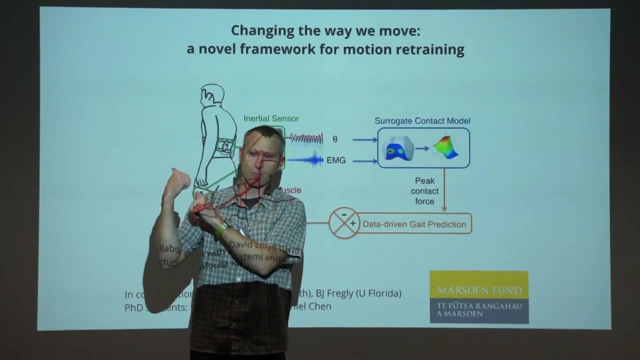 And we use partial least squares regression. for this You could use an artificial neural network or something similar, And you're basically saying: here's a response surface for these inputs. This is my output, And once you've done that, this becomes very quick to compute. 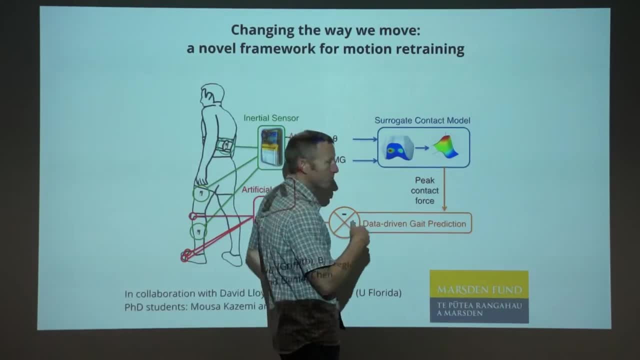 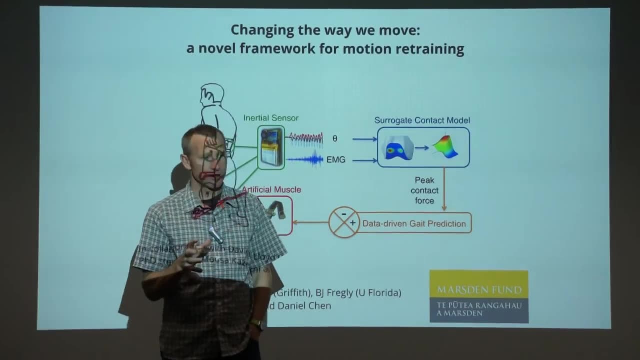 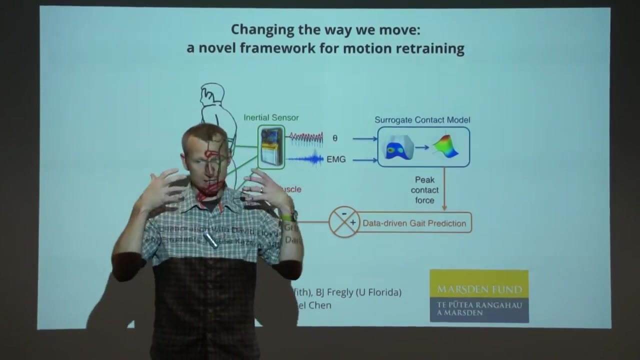 You can compute this in real time. And Tim Wu, who works now with Mark Sagar, did his PhD with Kumar Mutharatne And they did a really nice presentation of a nice paper that showed this method, using partial least squares- regression- to characterize the deformations of the face for animation. 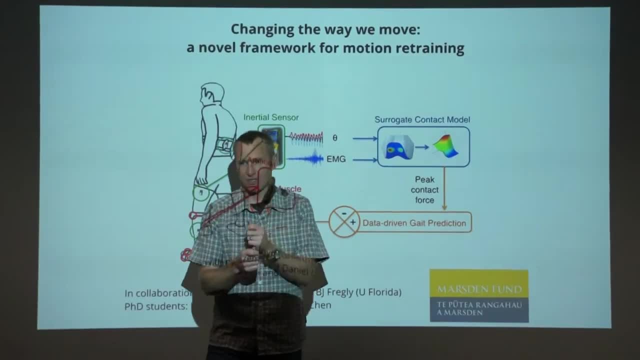 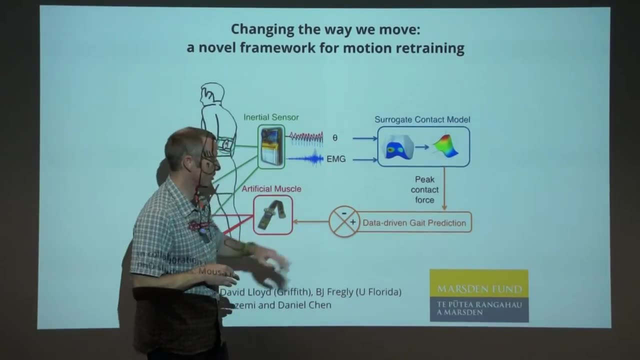 So they can use some very quick then little sliders, essentially to characterize all the different movements of the face and get very accurate deformations of the soft tissue and the skin of the face. So we're just using exactly the same method, but we're now predicting what the contact 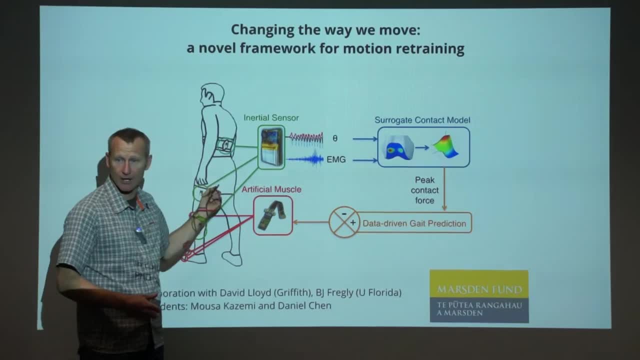 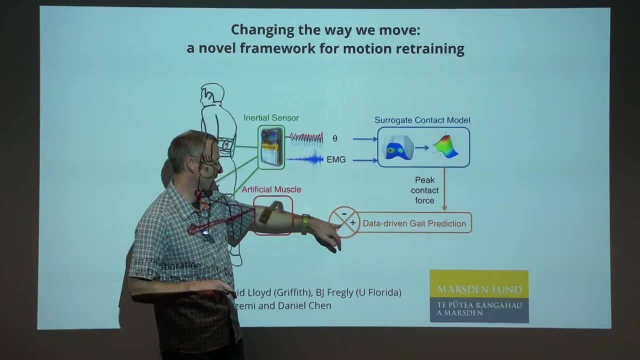 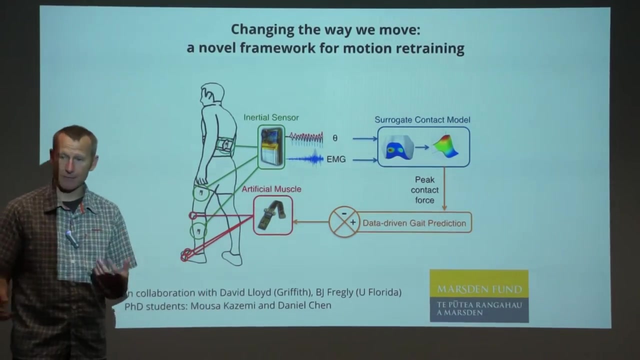 forces are, And this will work in real time. so we can plug that into our rigid body dynamic framework. We do something called data-driven gait prediction. I don't have time to go into that today, But this is a way that we can, for an individual, prescribe a new gait pattern, a new way of 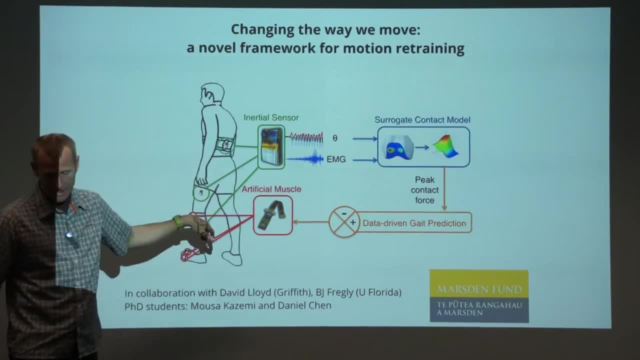 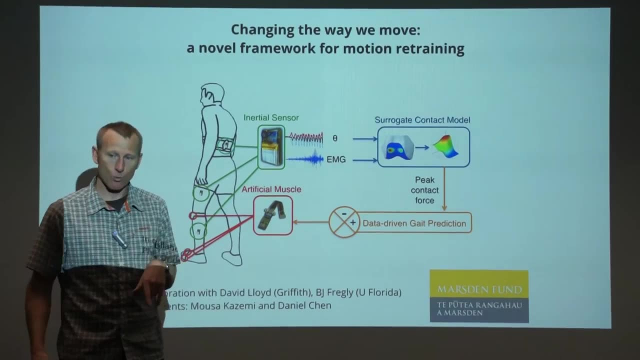 walking And the concept here is that you have someone with knee osteoarthritis which mostly occurs on the inside of the joint. What you're going to do is you're going to tell this person how to walk to alter the joint loads. 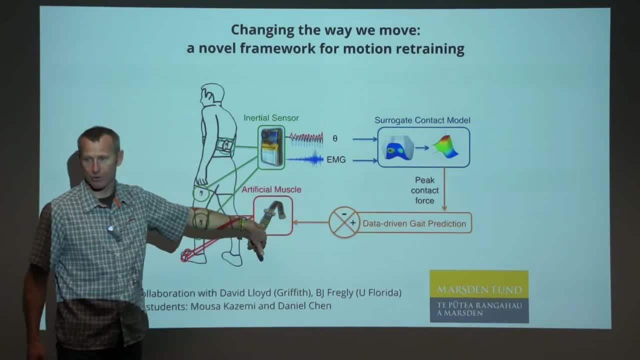 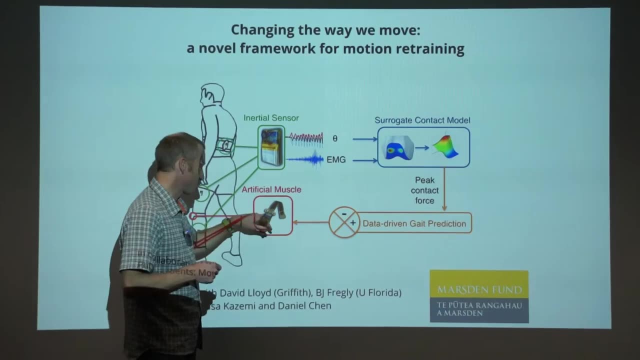 And you can measure those joint loads in real time and you give feedback to the person. The initial idea we were starting playing around with artificial muscle. so Ian Anderson, on level five, We started playing around and Daniel Chen was a PhD student with us doing this. where? 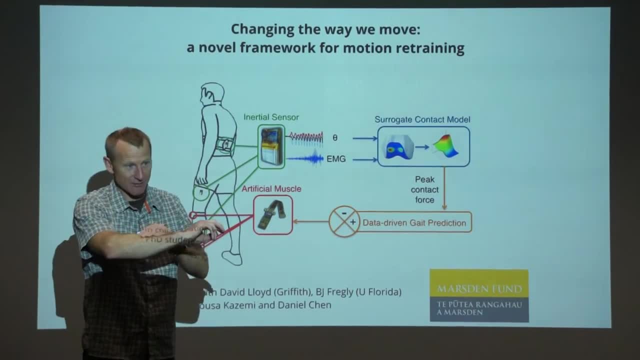 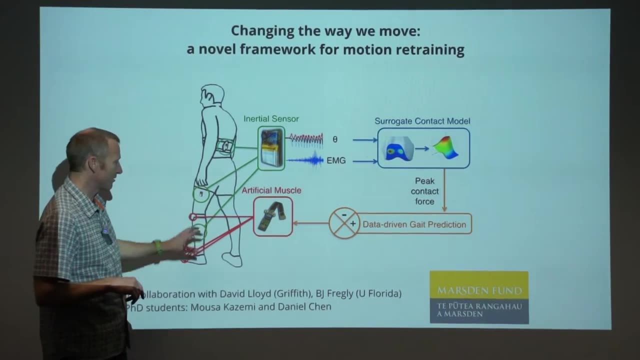 you could put the artificial muscle in your skin And then it would stretch your skin And via the skin stretch you can get this intuitive feedback about where you should be and how you should move. We've done quite a lot of experiments on that and we've since kind of moved away from the 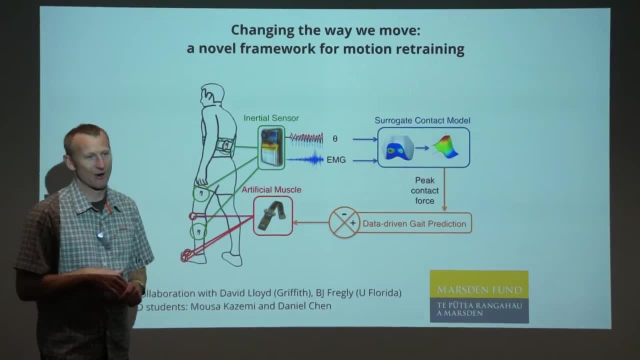 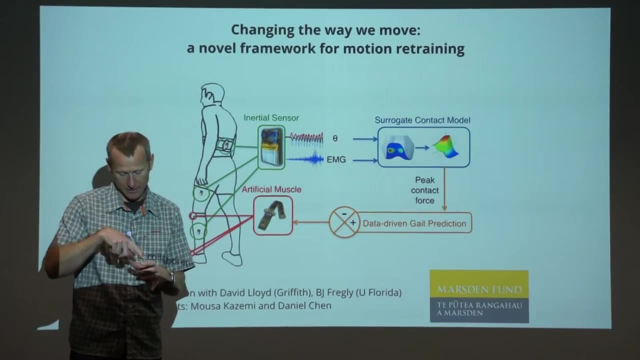 artificial muscle, mostly because it's quite dangerous, because you need very high voltages to operate these things, actuate them. We're using vibrating motors and putting them in a spatial arrangement so that you can get them and you activate them in a sequence and you can get this intuitive sense of roadway. 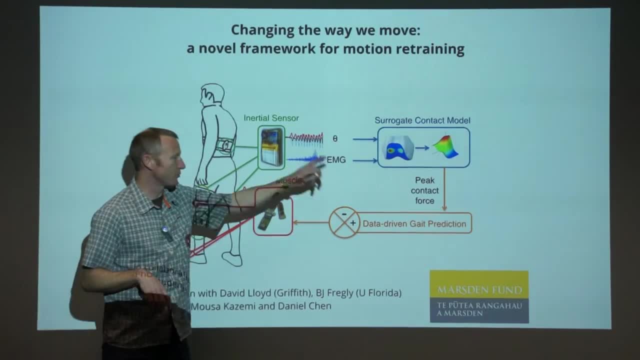 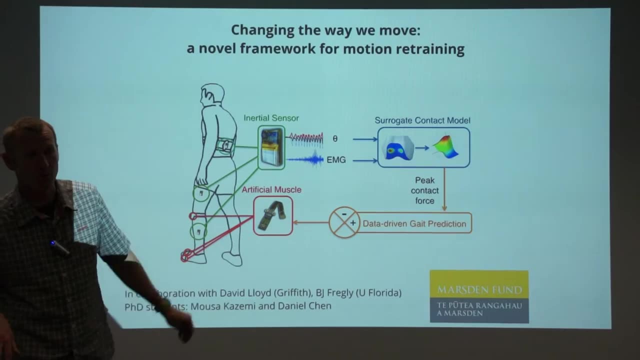 Okay, So we've got the rotation and movement And we then close the loop and we can do this in real time And we can reduce someone's knee joint loads by about 30 to 40 percent in about two minutes, And that's equivalent to what a surgeon would do, which is cut away a big wedge of bone. 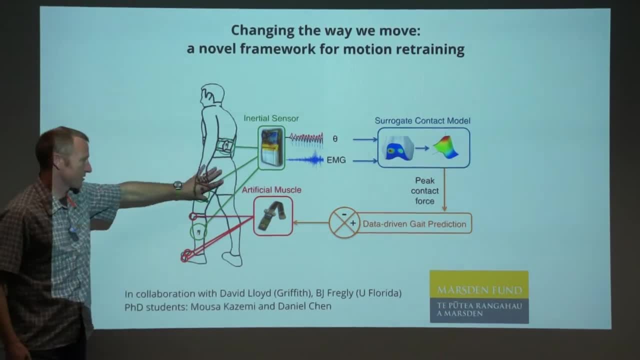 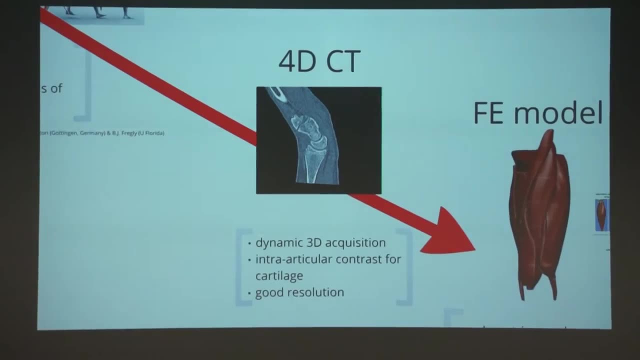 and realign the joint, So we're pretty stoked. That's a great outcome for us. The next thing would be: well, how do we get this to the clinic? Okay, Just briefly. then The imaging. Let's talk about the limitations of imaging. 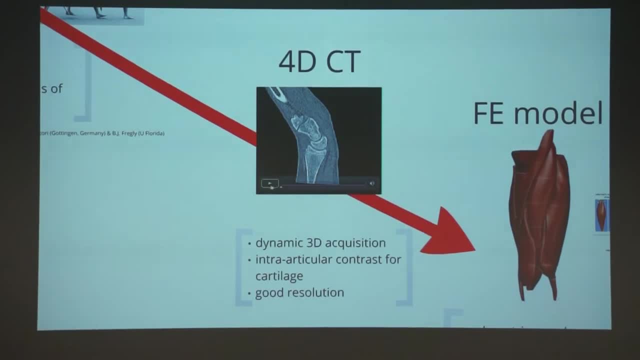 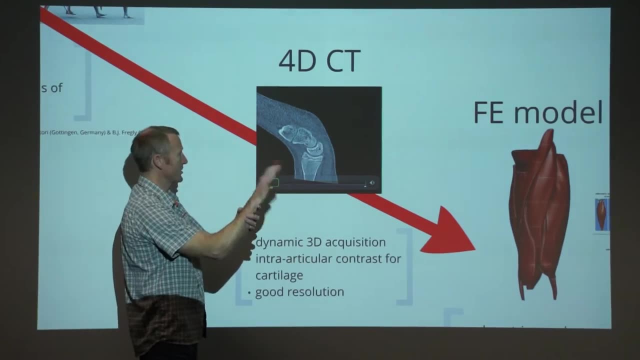 This is 4D CT. This is about six to eight frames per second now, But this is full. With every frame you get a full 3D reconstruction. This is the wrist, So this is flexion extension of the wrist. 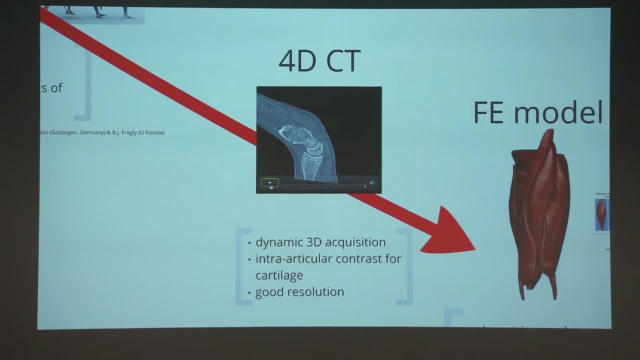 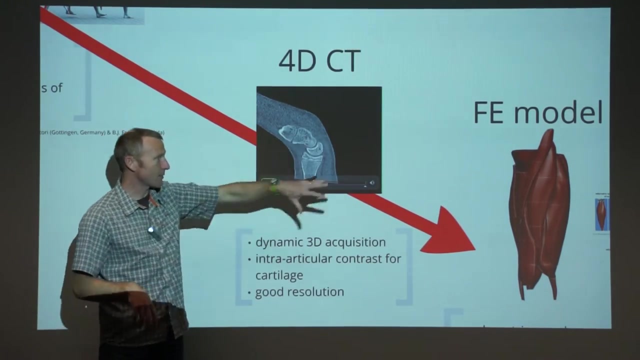 This is the radius and the carpal bones, And so this is with a colleague who's now with Toshiba, And the idea is that you could have a dynamic acquisition and you could accurately characterize the dynamics of the bone And then couple that in, say, with a final model and look at the stress distributions. 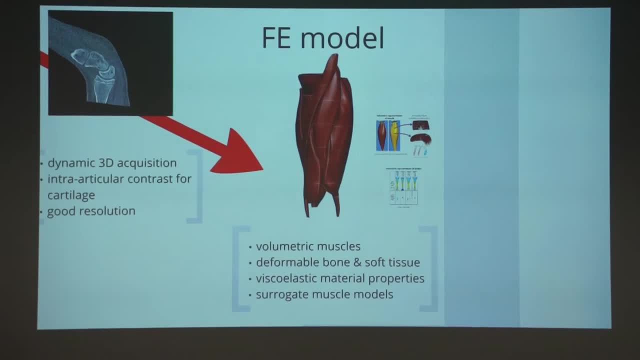 We're moving away from these line segments and again building surrogates that represent the volumetric muscle, And this was work from Justin Fernandez in his PhD, which he did here at the Institute. Then he went to Melbourne, did a postdoc and now he's back. 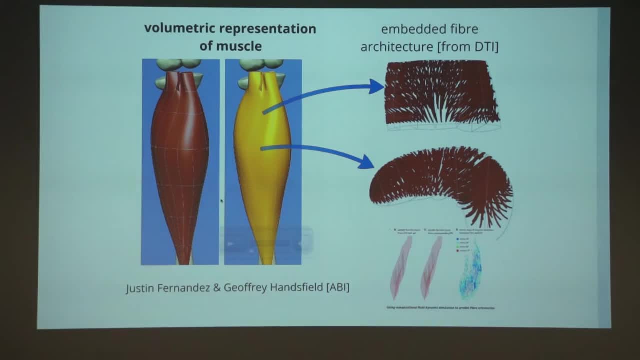 And Justin and Kumar have done quite a lot of work in this domain. These are some simulations of a gastrocnemius. Okay, And this gastrocnemius. we've assumed that all the fibers run parallel And you can probably guess what that's going to look like when you activate the muscles. 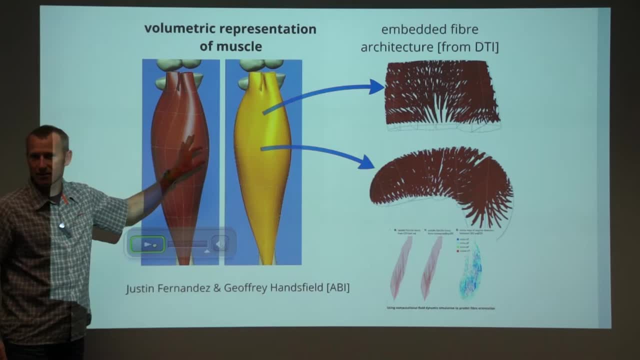 You get a pretty uniform contraction. Is this what a real muscle? does Any guess If you kind of looked at your calf muscle and did that? No, it's not. The reason why is if you look at the real architecture. now, this is from diffusion-tensure. 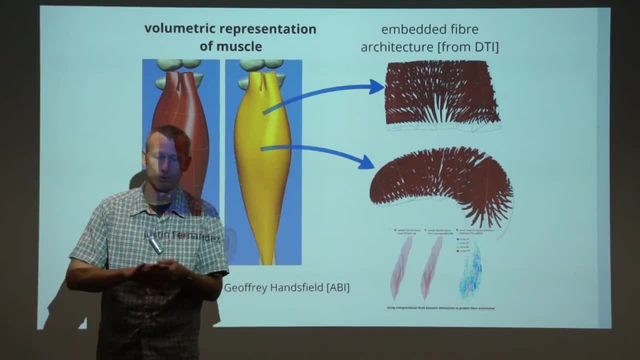 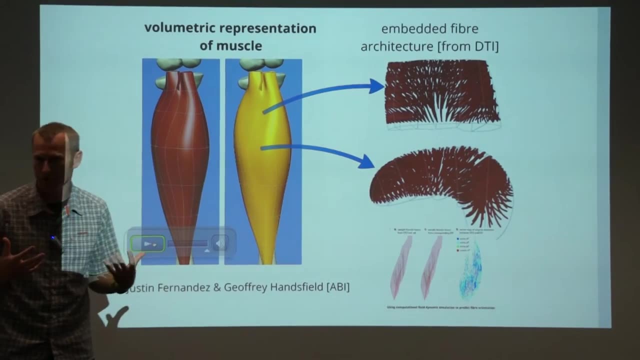 imaging- Again, same tools as what the heart group does. But if you look at the fiber orientations, These are highly complex fiber orientations. The architecture is not very simple. But if you embed that fiber architecture into the muscle and then you stimulate those, then 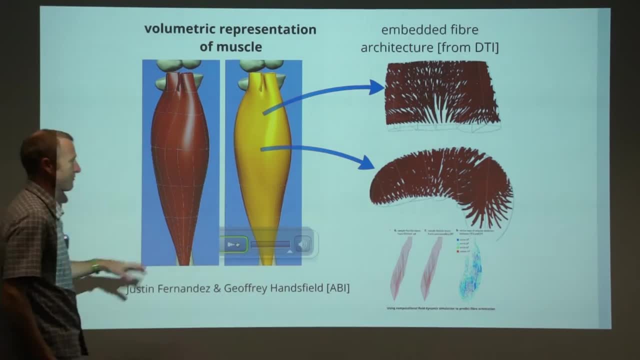 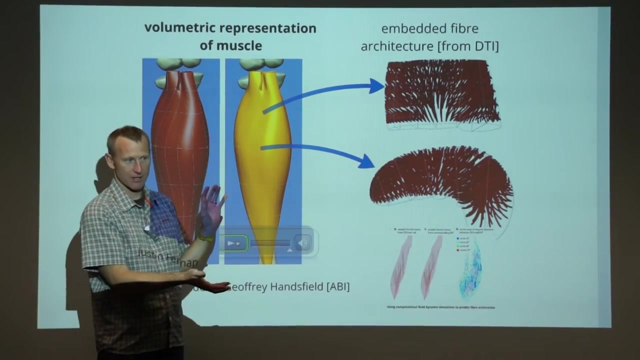 you get quite a different deformation. You get something that's actually far more realistic, actually, And it changes the mechanical behavior of the muscle. The idea here, then, is that we can again build a surrogate. This time instead of doing a joint contact simulation. we have 3D volumetric FE models. 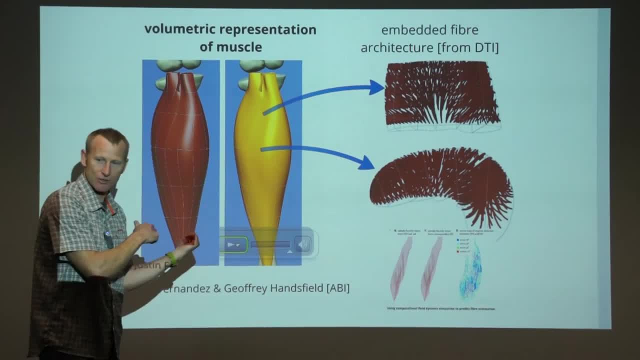 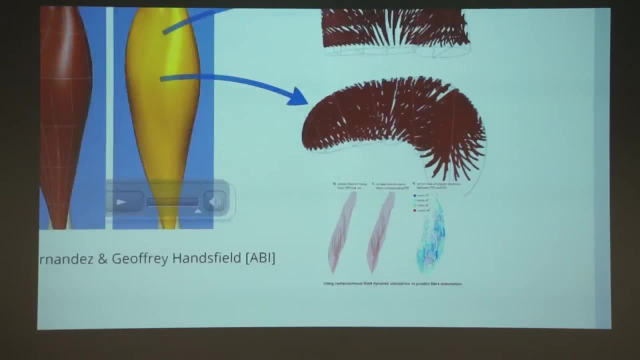 of muscle And you create a lookup table. then that goes back into your rigid body dynamics. So then you can characterize the complicated fiber architecture and wrapping. And this is work. actually that's been extended by Jeff Hansfield, who's a postdoc in our 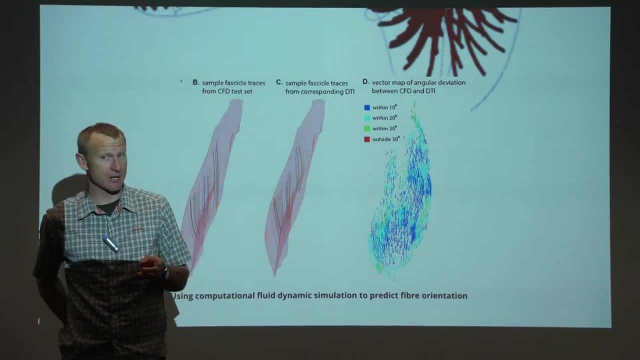 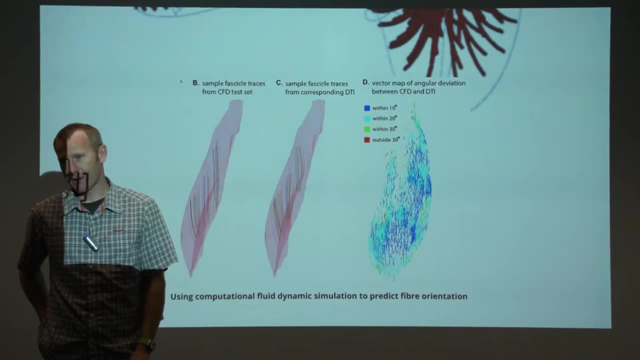 lab And Jeff's doing some computational fluid dynamics And what he's doing is says: well, we're not going to get diffusion-tensor imaging on every subject that walks into the lab, But what if we could get a proxy for those fiber architecture by doing a fluid dynamic? 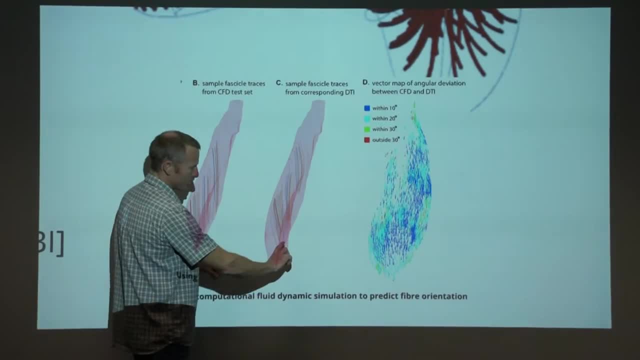 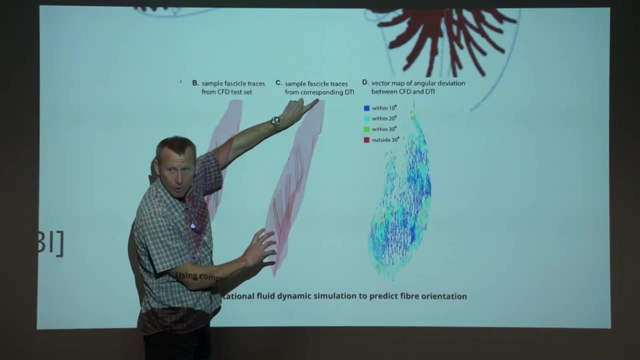 And what he does. he sets boundary conditions where the aponeurosis is, where the tendon attaches at the proximal and distal ends, And he solves a fluid problem and says: well, if fluid was coming in here and exiting there. 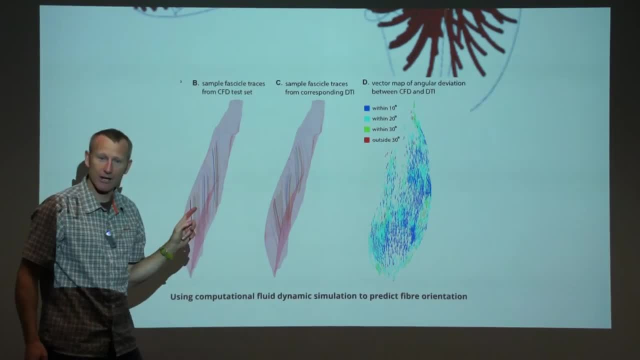 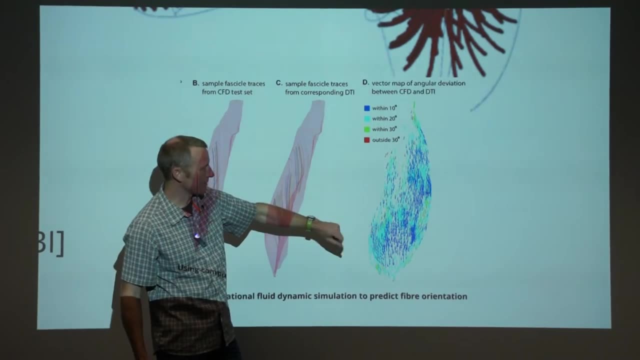 how would it flow? And it turns out it flows pretty much in line with the fiber architecture. And so these errors, these errors between the computational fluid simulation and those fiber directions. It's measured from diffusion-tensor imaging And you can see, the majority of these vectors are within 10 degrees. 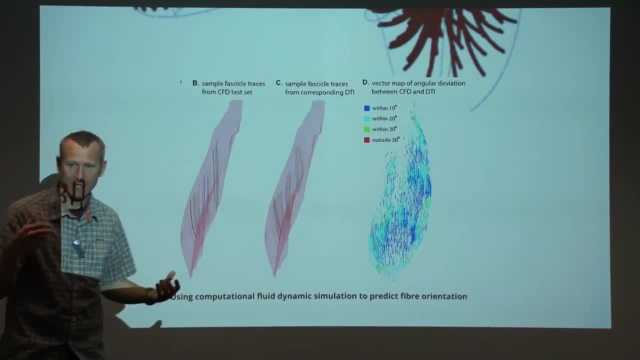 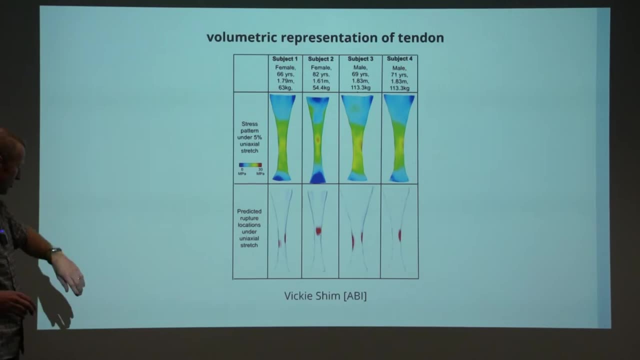 So this is now a method that you could use to predict what the fiber architecture is without having DTI. So again, it's all about clinical translation, And this is some work. I've just only got a couple of slides left. Vicky Shim treating then the tendon. 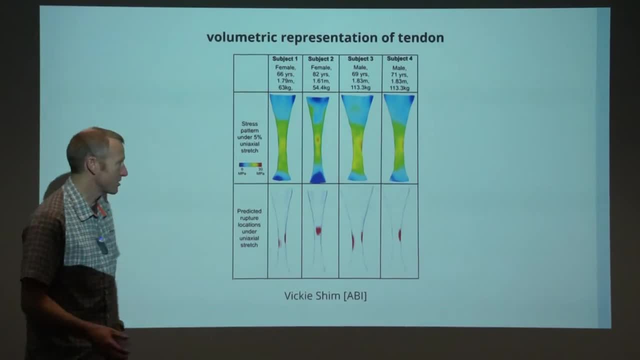 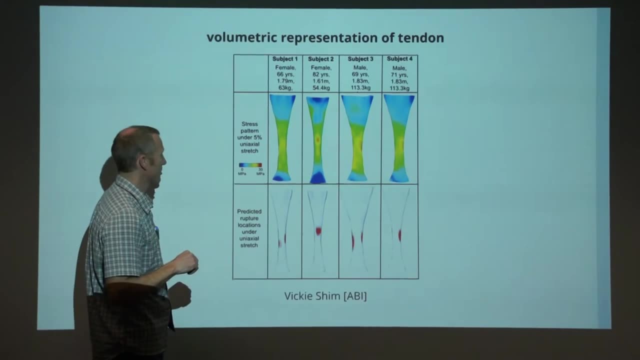 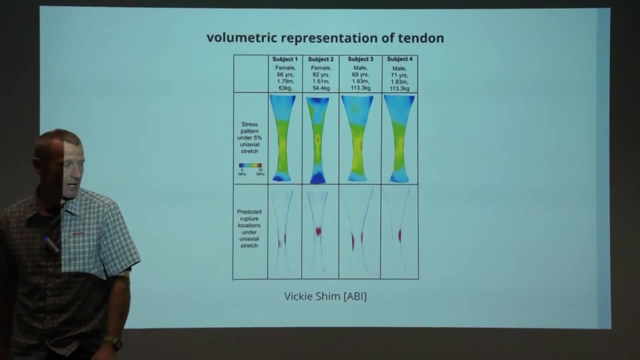 This is the Achilles tendon as a volumetric representation as opposed to a line segment, And what you can see. with different patients, You get different stress distributions And you can characterize different loads and boundary conditions. You could predict the regions of rupture under these different load conditions. 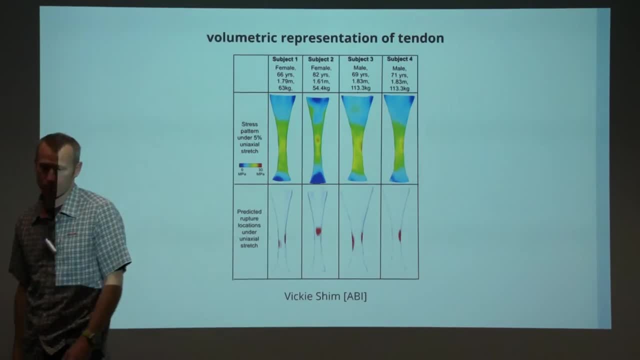 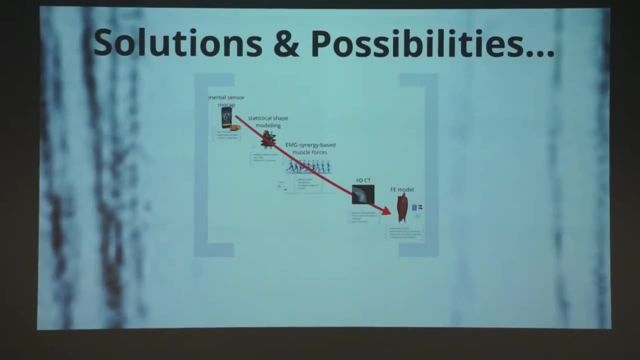 And a lot of this is dictated by the geometry as well as the material properties. So we're kind of working in the space of getting away from the line segment representations. So that's it. I'm going to end there and thank, of course, people involved. 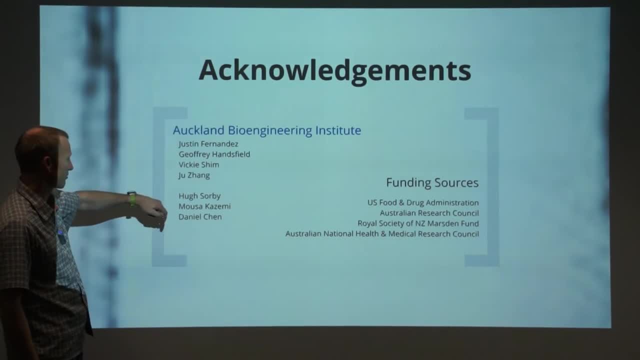 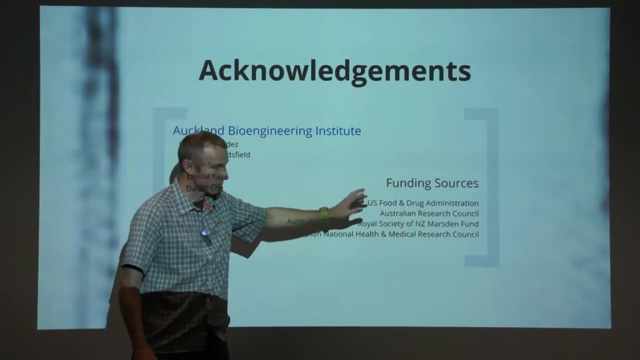 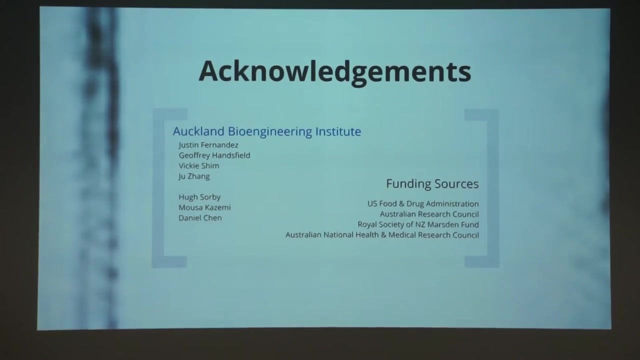 There's probably a few more people that I've missed out on here. Kumar was one. He's done some work with Justin on the deformations of muscle architecture. There's been a number of people who have funded this work over the years But critically it's been done by the students that have been involved. 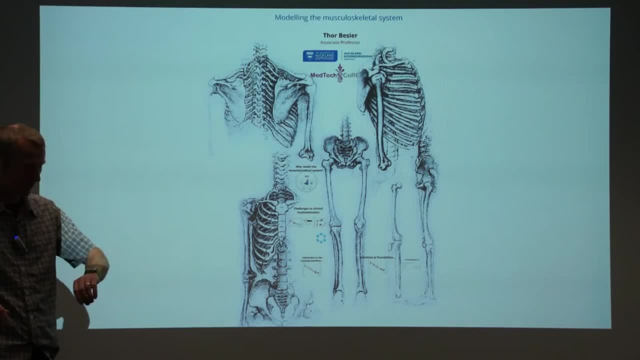 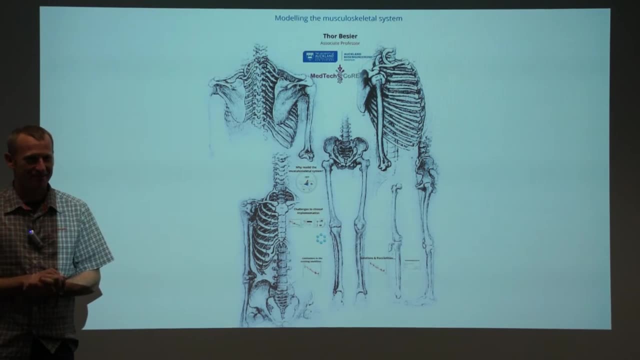 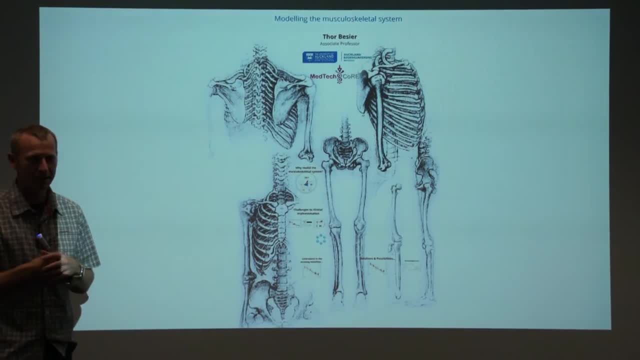 of workflows, And is there anything new, Any new ideas here that have kind of sparked your interest about? oh, maybe that's something I could use in my own research. No, Excellent. OK, Andre and Hugh, do you have any points or comments? 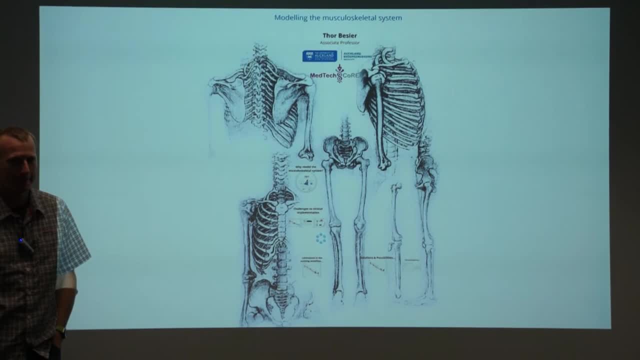 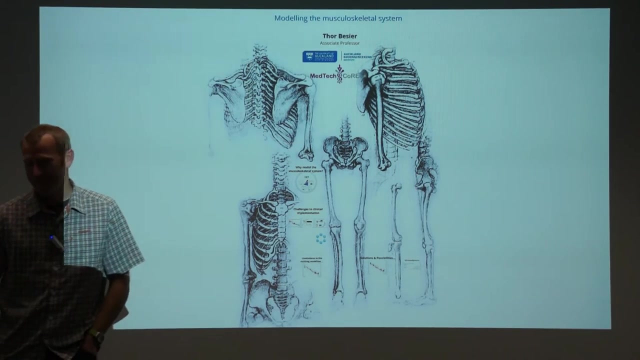 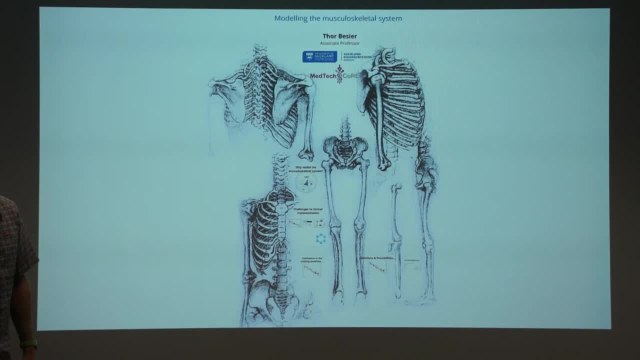 Maybe things that I don't know. I covered a lot, so maybe there is a lot there. I did have a question from earlier on, but It's good, That was the purpose: Smoke Screw, so exactly, Okay, This. 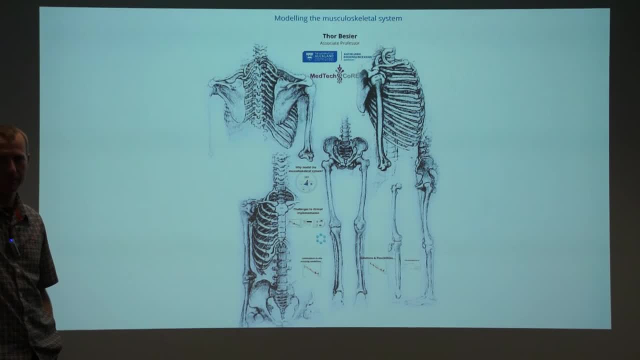 It's all the same sort of. it's very different applications, but very similar. in a sense, It's a lot about pretty much what they're going to go through next in terms of what they're going to play around with themselves. So it should lead on very nicely in the next part of this day. 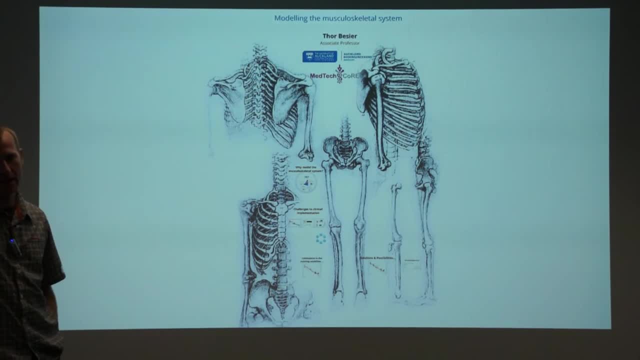 Yeah, great. Yeah, I mean it's been a shame in some ways that we haven't worked more closely in the past. If you think about even us at the Institute, you know we span five office floors here and you think, well, surely you're sharing all the code, right? 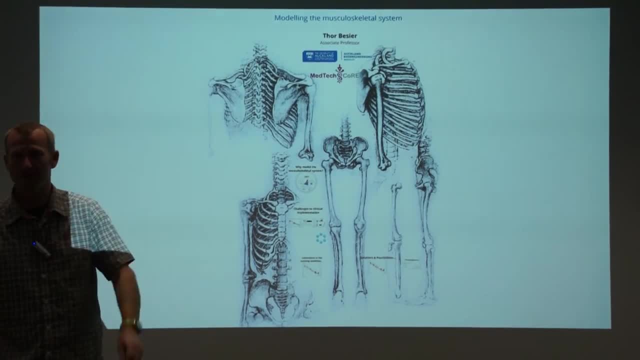 You're all doing these surrogate models or you're all doing some segmentation. you're all doing parts of the puzzle And it's remarkable how little we actually share, I think, given that we're doing the same stuff just with a different application. 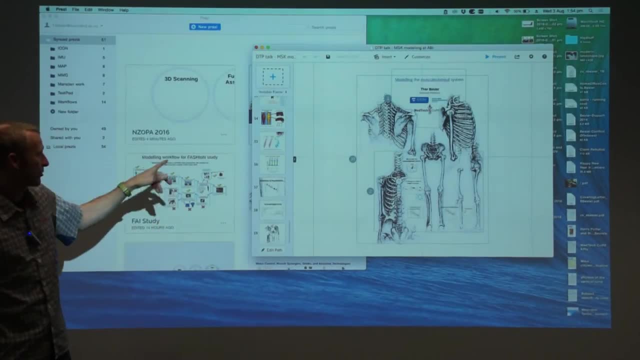 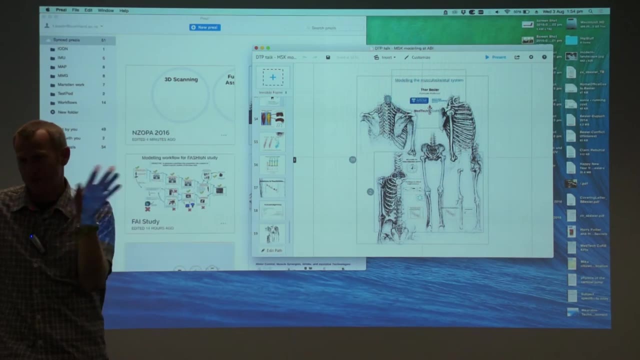 And that was really one of the driving factors When I first started. when I wrote the grant to get funded for this musculoskeletal atlas project, I did an invitation to the Institute to see if anyone else was interested, and pretty much the whole Institute turned up. 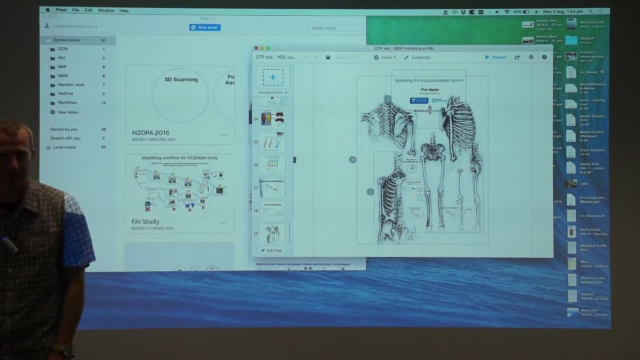 Because everyone's got a vested interest in this. And so then I realised: okay, this is much bigger than just the musculoskeletal group. Even though it's maintained the name MAP client, which is kind of nice, We've stamped our authority on it and said it's musculoskeletal atlas project. 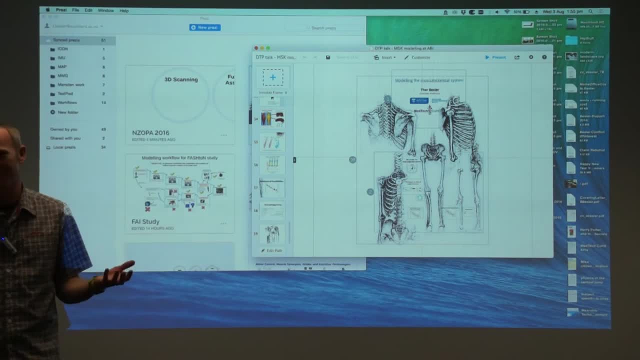 You know it's. yeah, the end result is really a generic workflow. It's a workflow manager and you'll experience it And, yeah, I'm slowly being taken over by everybody else, But we'll see. We'll see where that ends up. 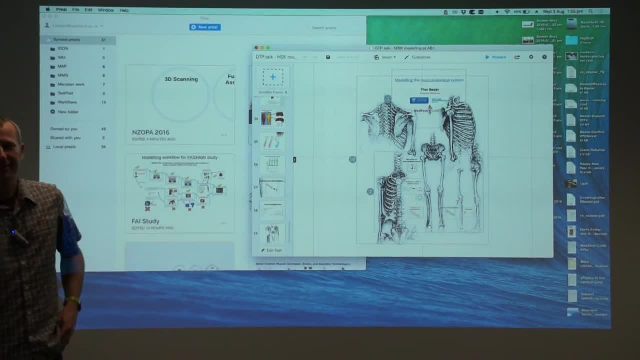 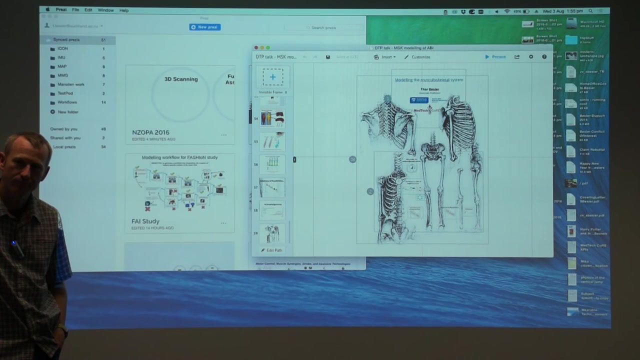 What, Yeah? Can I ask another question from our side of the spectrum? So all these elements in the workflow that you presented just now, they are done only with MAP client, Or there are also other software? Yeah, Okay, That's a good question. 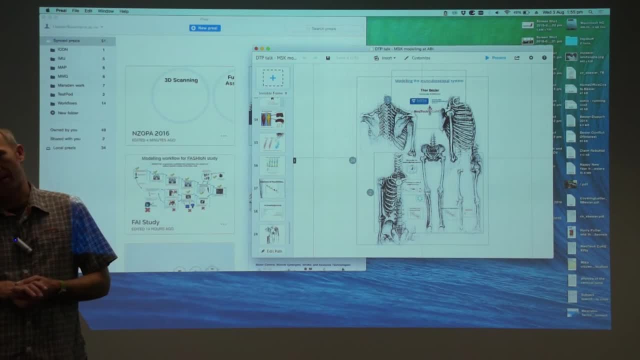 So ultimately, we would like to have a lot of these steps integrated into MAP client, That it's a one stop shop, It's all free, It's all open source And the idea is that people from around the world will contribute and everyone works together. 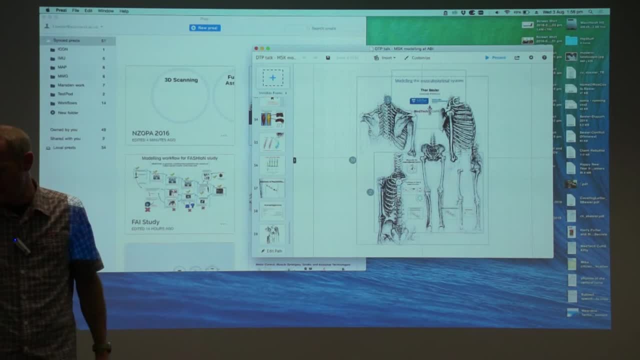 Not just our Institute. You know it's broader than that, And science is all about adding on top of what people have done before. It doesn't make sense that we're all doing the same thing in different silos, So it's very much an open source philosophy that we have on it. 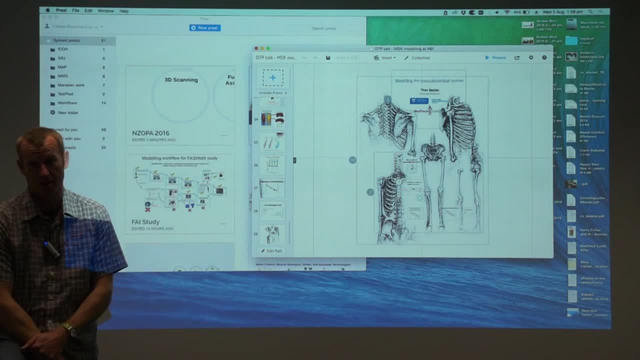 The reality is that there's still a few parts of the puzzle that are done elsewhere. So some of the simulation, in particular, of course, the dynamic simulation, we do. we use OpenSim for doing certain parts of the rigid body dynamics, But then we write our own code. 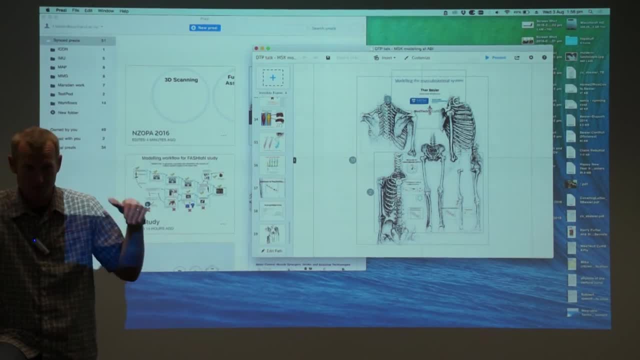 For example, we have our own C code that does the EMG to muscle force, And that's work that I did for myself. I got my PhD and we've continued to develop over years. So that's a separate component, But the idea is that we get access to those components via the MAP client. 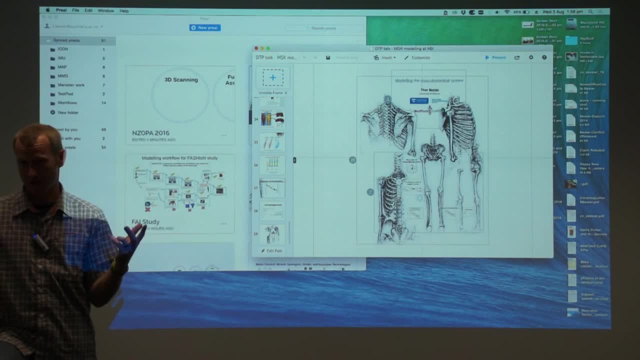 So even if you don't know that code, if you have the hooks in place that you can have a wrapper or some calling function that says: OK, here's my model. Now spit it out to this bit of code or this software over here and run a simulation and come back. 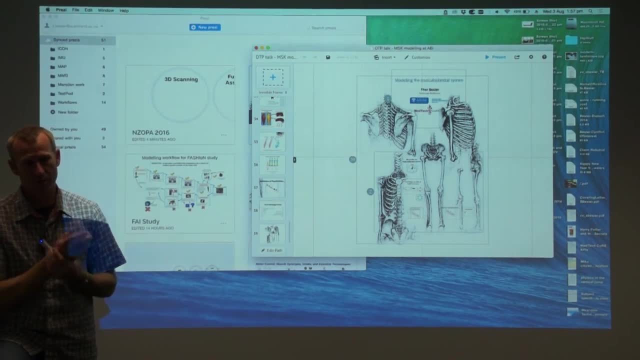 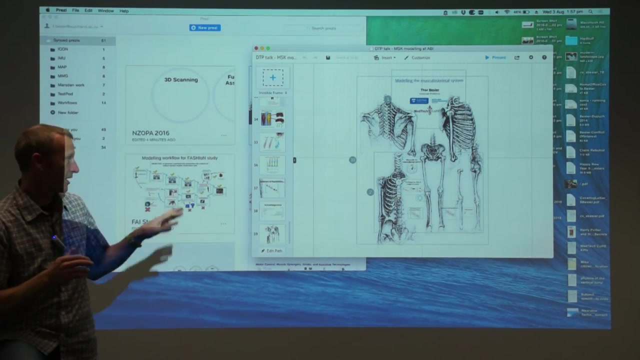 then that's great. There's one thing I will say about that approach- And it's a caveat or it's a bit of a danger- is that when you provide tools that are so easy to use, they can sometimes be misused, And I think this is what I mean by that is, the finite element method is kind of a good case in point. 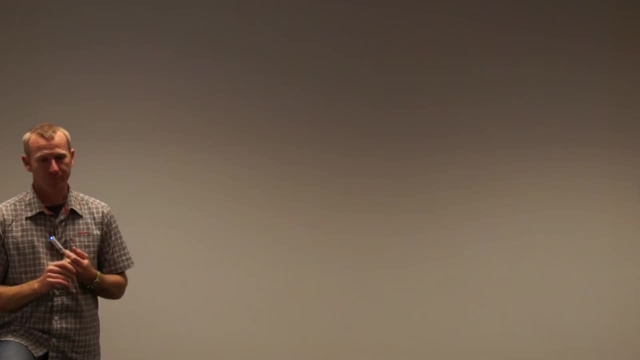 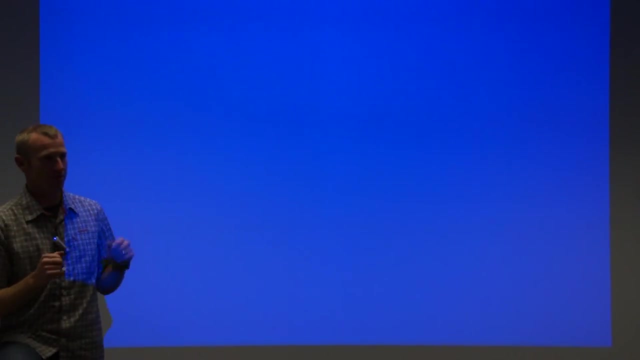 The finite element software that you can get nowadays is pretty easy to use: the commercial packages. You can put together some geometry, You can find some loads and boundary conditions And you can run a simulation And anyone can pretty much be taught how to do that. 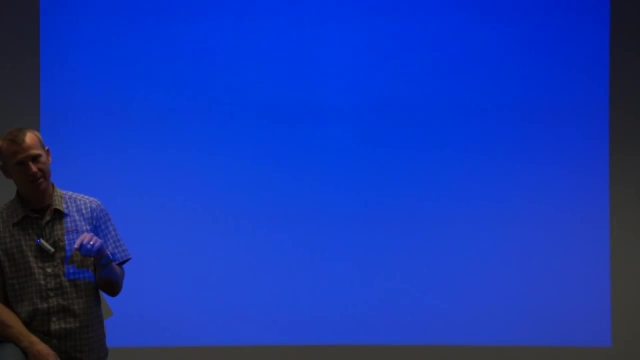 The biggest question, though, is: well, what is that simulation telling us? What are the inputs to that simulation? I need to have a pretty good understanding of that model, and what's in the guts of it, before I can be confident in what it gives me in the end. 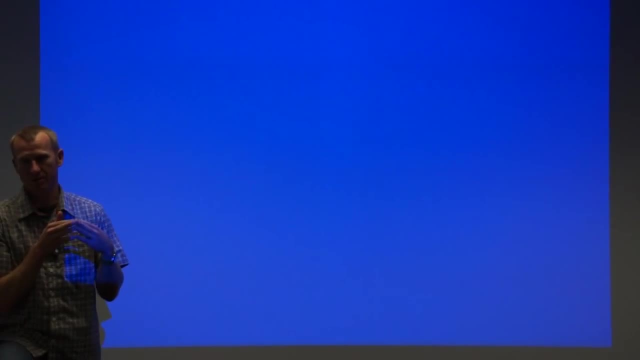 And so there's a bit of a clash there, because ultimately you'd like to know everything of that model, But you don't have the time to derive the finite element method from first principles and write your own FE code. It just doesn't make any sense to do that. 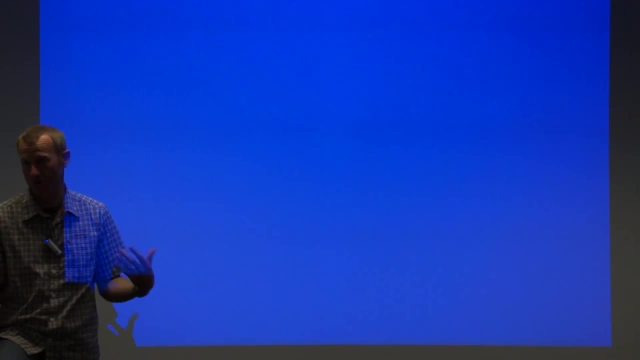 And the same is true for rigid body dynamics and other codes and other solvers. But you just want to be critically aware of the models that you make and the limitations and the methods that you've used, so that the results are all taken under that context. 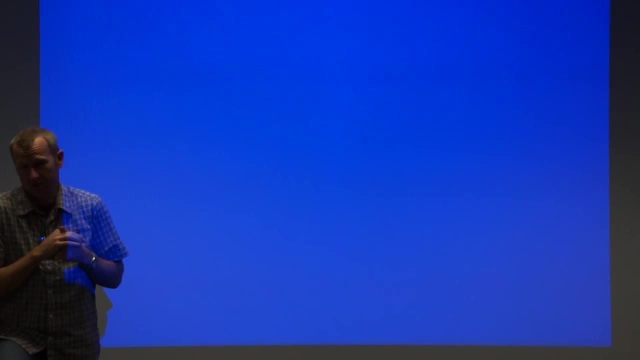 Does that make sense? Yeah, Because nowadays, yeah, it's easy. It's easy to plug and play and grab a model and run it and, you know, get results. But you want to be very critical of those results and where they come from and understand what's under the hood. 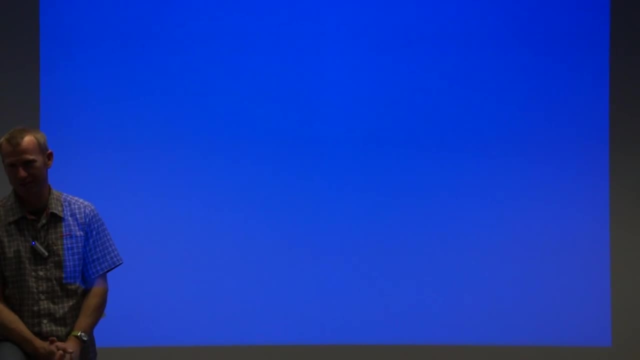 So that's. the only caveat with making the software tools easy to use is that you still want to have a good understanding of what's under the hood. Cool, Okay, Thanks everyone.